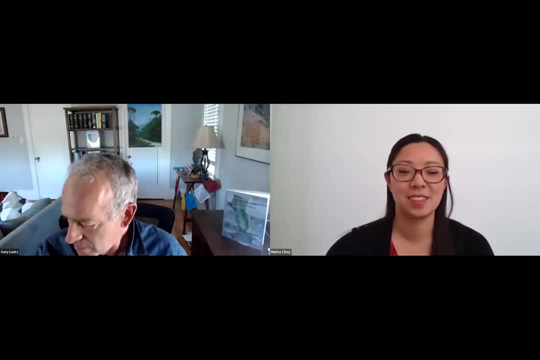 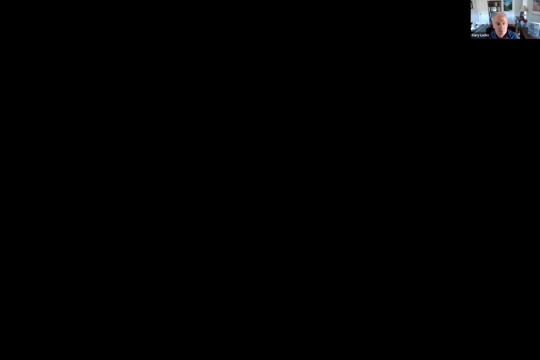 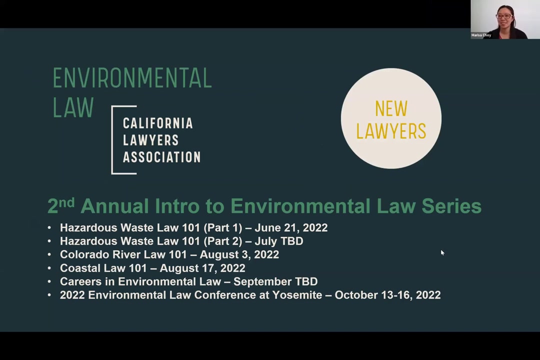 Gary, can you see the slides I can Perfect. All right, everyone, I think we'll get started. It's 12.01.. Welcome, My name is Marissa Choi. I'm an attorney in Los Angeles with Greenberg. 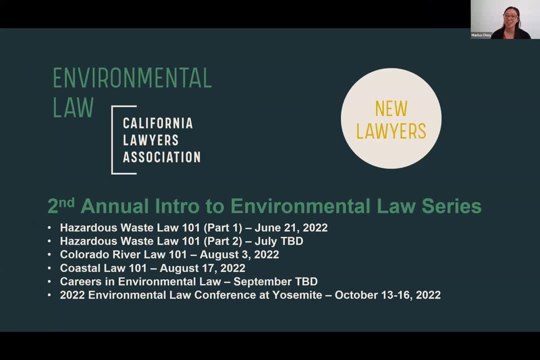 Lusker And I am delighted to kick off our second annual Intro to Environmental Law series. So I will talk about some of the organizations on the next slide. But basically we are a volunteer bar association And we are hosting this summer a series of 101 free webinars on Zoom And they're 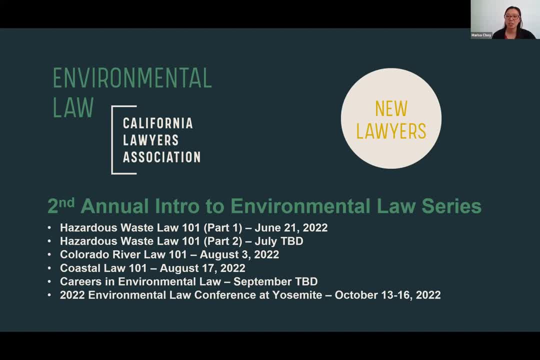 covering different topics in environmental law. Last year we had four sessions and they're available on our website to view if you missed those and want a refresher. But you can see, today we're kicking off with hazardous waste law And today's is going to be more of a lecture: learning. 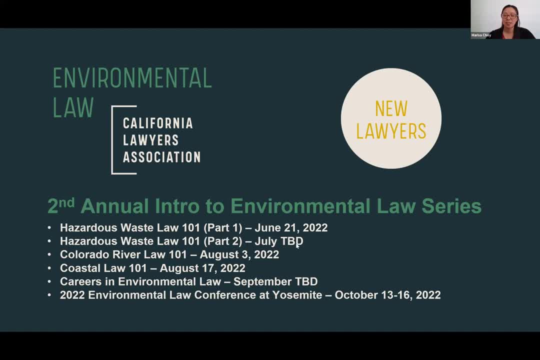 session And we're hoping to have a follow up with some more discussion and kind of real world practice examples. In August we're going to have a session on Colorado River Law, followed by coastal law, And then was quite popular a couple of years ago. we had a careers. 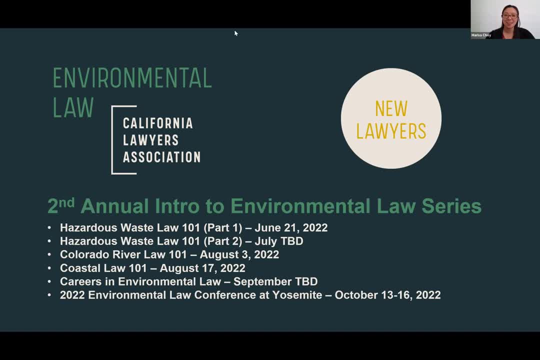 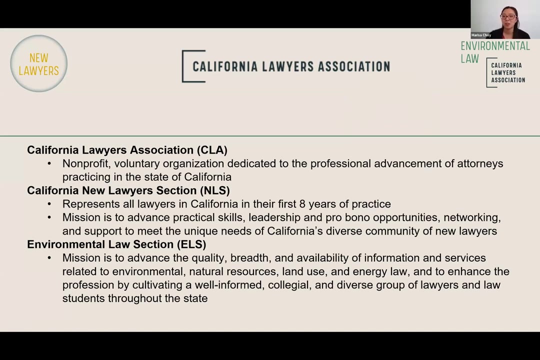 in environmental law series. So we're going to do a short panel in September leading into our annual Yosemite conference. So with that I will just explain what these organizations are. So CLA was formerly part of the state bar, but it's a nonprofit, voluntary organization dedicated to. 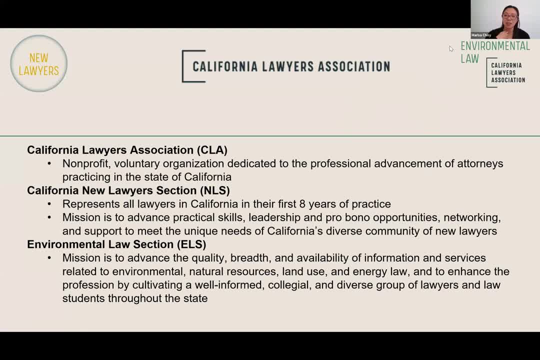 environmental law in California. I am the new lawyers liaison to the environmental law section. So CLA is the umbrella organization And it's got sections for lots of different practice areas: IP, international law, criminal law, tax law, anything you can think of. So 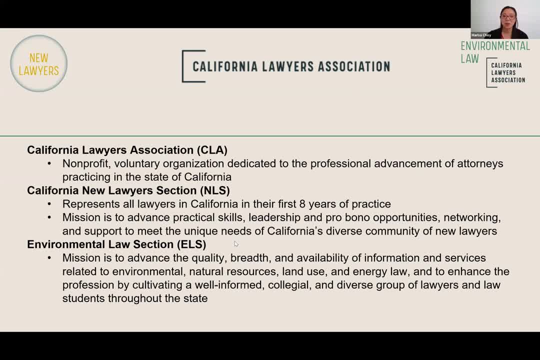 Gary is a longtime member and advisor to the Executive Committee of the Environmental Law Section. And then the new lawyers section is a section that's targeted towards lawyers in their first eight years of practice, And so we put on a bunch of programming and CLE And there's a lot of different ways to get involved. So, for example, 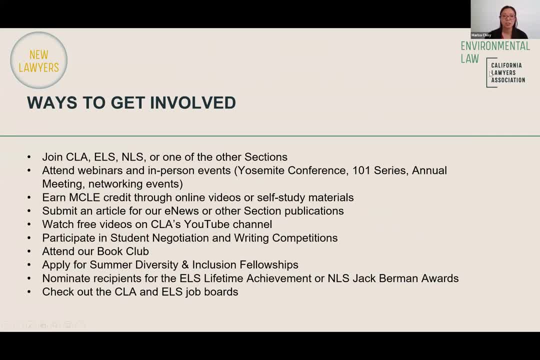 you can join any of these sections to get access to our materials. you can attend these free webinars or in person events. networking: there's an annual meeting. you can earn continuing education credits. submit things for publication. we have some free content. 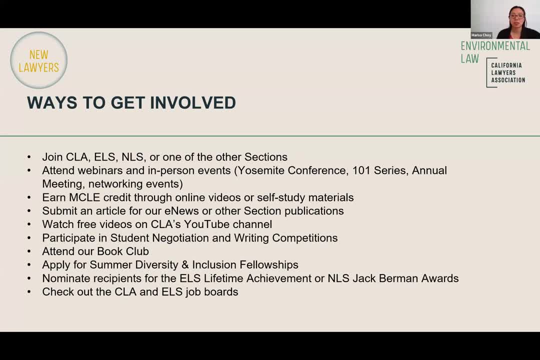 online on YouTube. the environmental law section sponsors every year a student negotiation And this year is brand new- a writing competition. We also have summer diversity and inclusion fellowships for law students. We we award lifetime achievement And then the new lawyers section has. 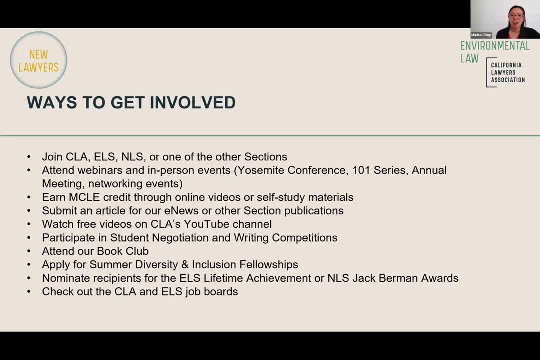 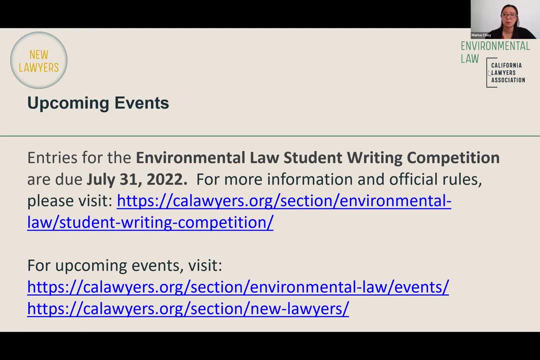 something called the Jack Berman Award for public interest each year, And we also have job postings on our job board, So please check out our websites and find ways to get involved. This is just info on the environmental loss writing competition that I mentioned. that's brand new this year, And feel free to look on the website at CA lawyersorg You. 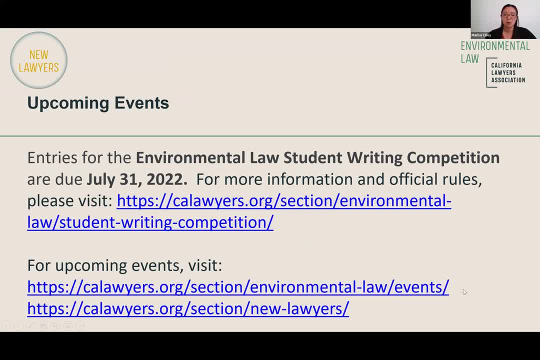 can find all the different sections. environmental law has a bunch of events: book clubs, webinars- Gary's actually doing a legislation webinar in a couple days- And then the new lawyers section also has content as well. So, again, my name is Marissa. 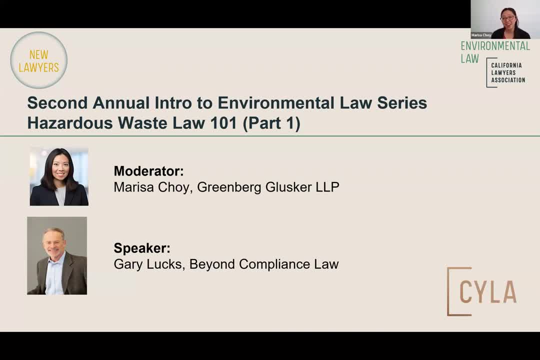 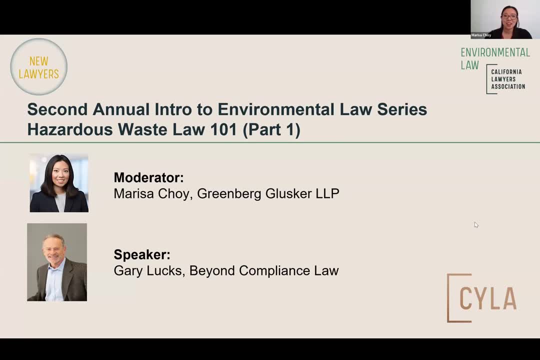 I'm in in Los Angeles- Greenberg, Wesker- and I am delighted to introduce Gary Lux with Beyond Compliance. He's in the Bay Area And Gary has deep expertise in environmental, health and safety, EHS law, legislative affairs and sustainability strategy. He is a licensed attorney, a scientist and a certified professional environmental auditor, CPEA. 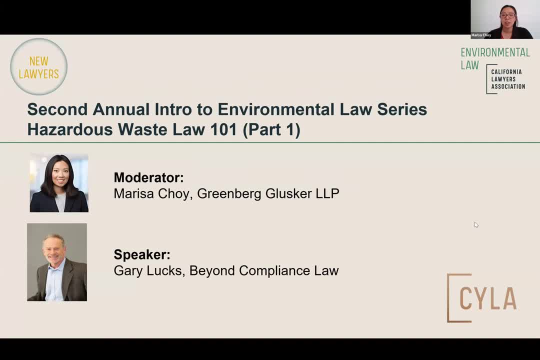 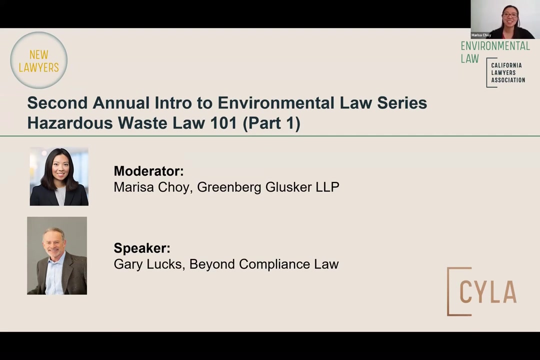 And he specializes in compliance counseling, environmental auditing, environmental management systems permitting and training. Gary has written policy papers for a lot of high level legislators, He's published a book, environmental guidebook and chapters in environmental treatises, And he has taught courses on environmental law, auditing, sustainability, climate change and legislation for over 30 years. So he is very well qualified and has tons of good content for us. 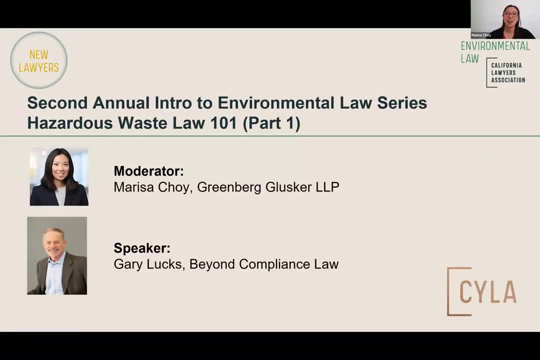 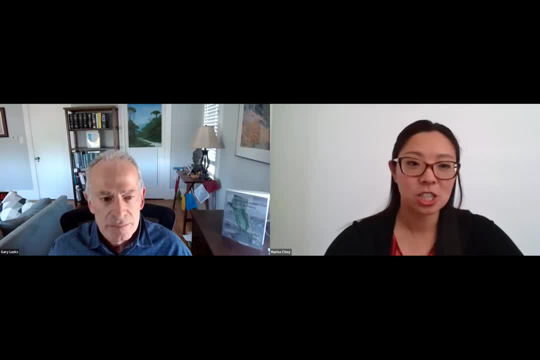 Because this is such a meaty topic, we thought that we would give him a little more time. Last year- if any of you watch the series- we did kind of quickie lectures and then got to hear from practitioners who talked about some of the real world examples. This year for hazardous waste, we are trying 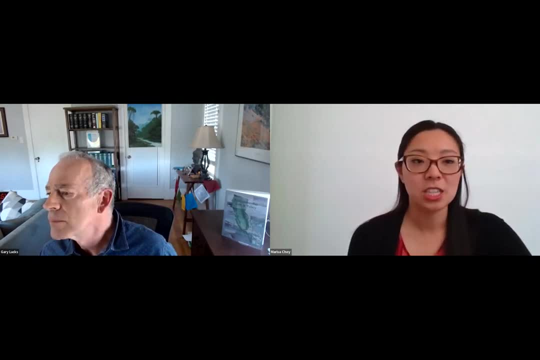 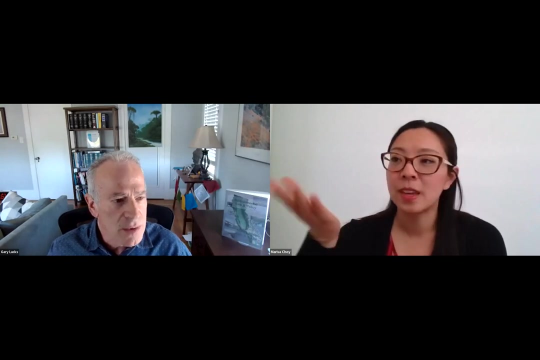 to make this session more of a lecture and get all the good content and teaching and then we'll follow up with more of the interactive professional perspective at a later date. So keep posted And Gary, I will let you take it away. Yeah, and I'll just mention these will be recorded. So if you need to drop off they'll be available later for viewing on the website And we'll try to leave some time for Q&A at the end and I'll monitor the chat. So if things come through, Gary graciously said he can kind of field questions for you. 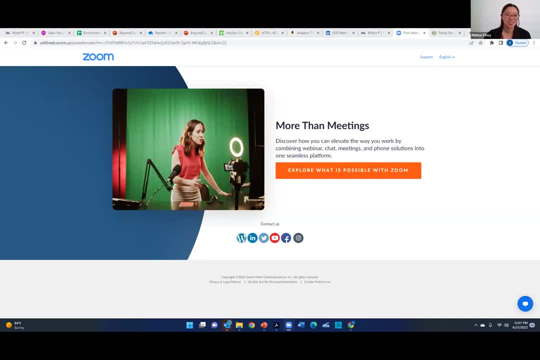 questions as we go along, Thank you. Thank you, Marissa. Can you see my slide deck here displayed Or do you need to share yours? I'm just going to zoom the Zoom screen, So if you click on the screen, Let me try that again. Let me stop the share and share again. 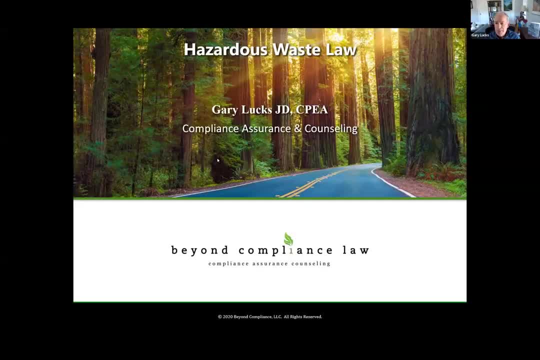 Do you see that? now The slide? Yes, Perfect, Okay, Great Well, thank you, Marissa. Thanks for Marissa put a lot of time and effort into developing this one on one series And we thought it'd be a valuable opportunity for lawyers cross training from one discipline to another or new. 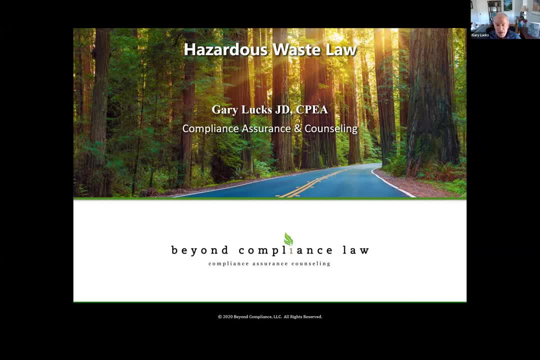 lawyers in the field, And so I'm pleased to be sharing the high level overview of the framework that governance has of this waste law, And what I'll cover in the next few minutes is a little bit about what it is, And what I'll cover is really the federal and state requirements as 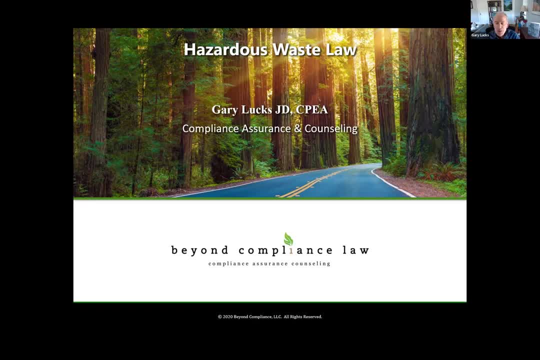 they relate to each other And what we'll find with hazardous waste law. as with most areas, except for CEQA, NEPA and the Superfund law, these environmental regulatory programs are very prescriptive And, yes, there's case law that interprets the statutes and regulations and how. 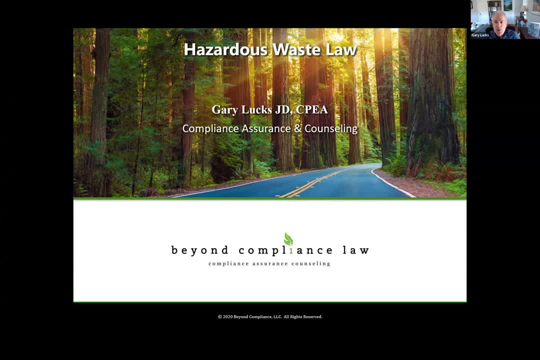 they relate to each other, But it's very, very, very prescriptive And I think it's very, very much a prescriptive framework, unlike CEQA, which and NEPA, which is quite focused on writs of mandamus and litigation and Superfund pertaining to potential responsible parties and liability. 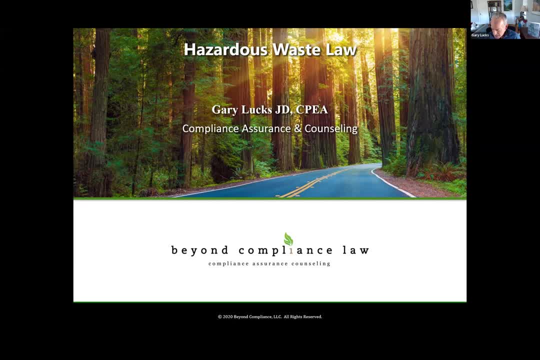 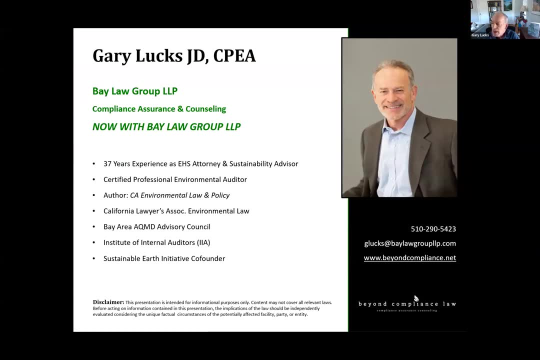 What I'm going to cover is really this framework here And see if I can advance my slide. Okay, There we go, Okay, And so you'll see that the slide deck will show Beyond Compliance Law, my former law firm- I just recently. 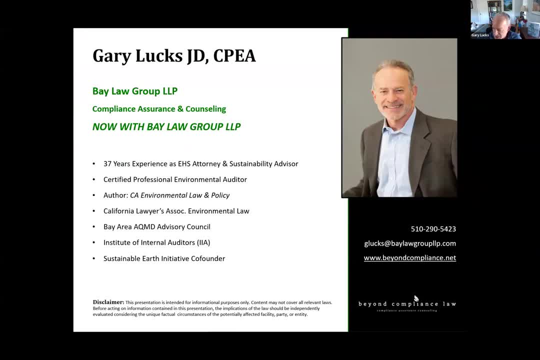 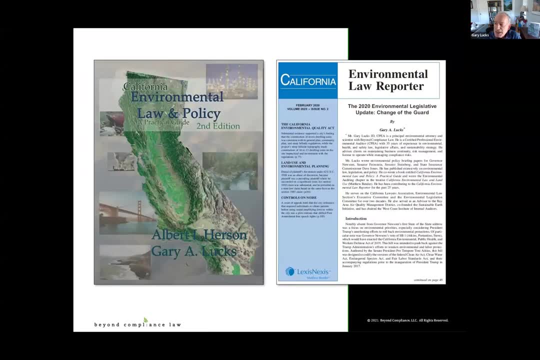 joined Bay Law Group, So we're in the midst of transitioning, So there might be a little confusion there, but I'm with the boutique law firm of Bay Law Group, And so to the left. you see, this is the book that I co-wrote with Al Herzon, which is a textbook that is focused on 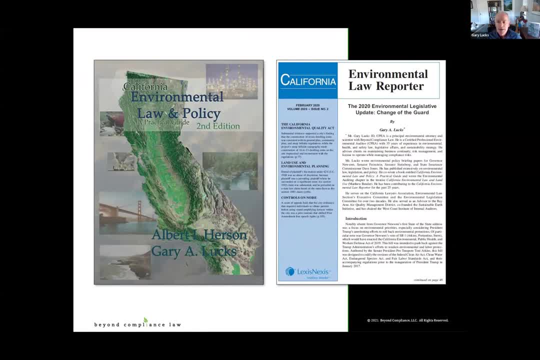 the overview of the universe of environmental federal and state laws. There's a whole chapter in there covering hazardous waste law, which I've drawn from for this slide deck, And so the book is about to go into its third edition within the next year or so, And anyway, if you're interested in new developments as well, 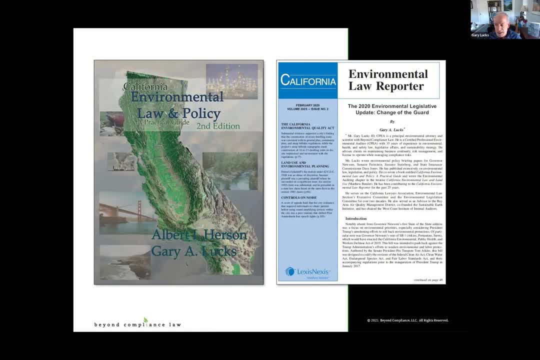 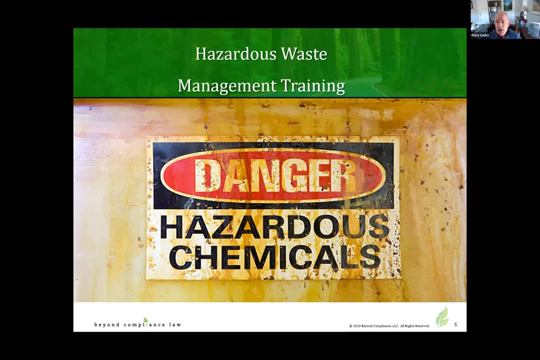 I write the annual article on new California environmental legislation. You see a somewhat more recent copy here. I'll share some of the the developments along the way during this topic, But, as Marissa said, 90 minutes is barely enough to scratch the surface, So I'm sharing with you a subset of what I normally teach, which is: 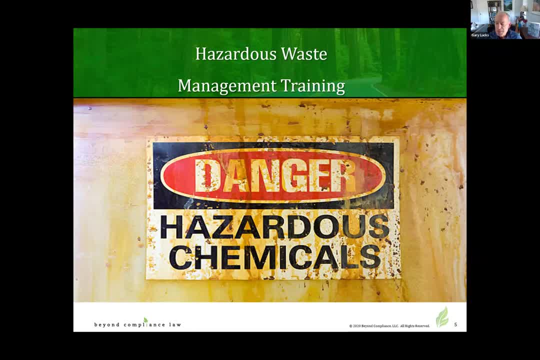 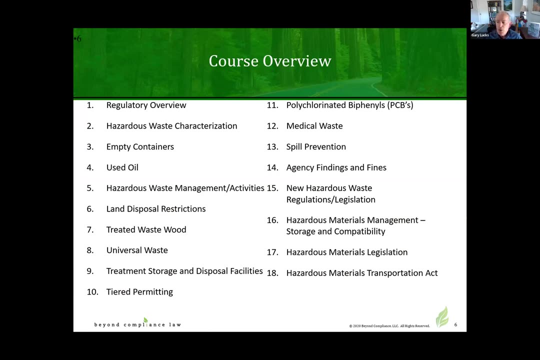 many, many more hours of topic, But we'll cover this at a reasonably high level and I'll try to stick to that level to maintain our time here. So coverage is quite broad-based and we're going to focus primarily on item number two. 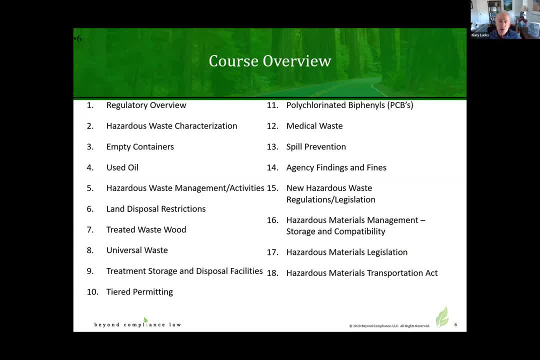 the hazardous waste characterization which, as lawyers, we need to have a level of understanding around chemistry and toxicology and the law, And so we'll see the interface and intersection between those disciplines from a hazardous waste profiling standpoint, And often lawyers are called in to address ambiguities around whether in fact there is a waste and if 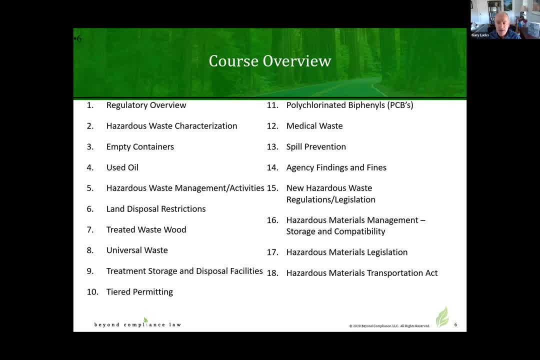 that waste is in fact a hazardous waste, And so oftentimes we'll be working with chemists and toxicologists together to interpret the law, and characterization and profiling is a big part of that, And then the framework of cradle-to-grave requirements I'll cover. 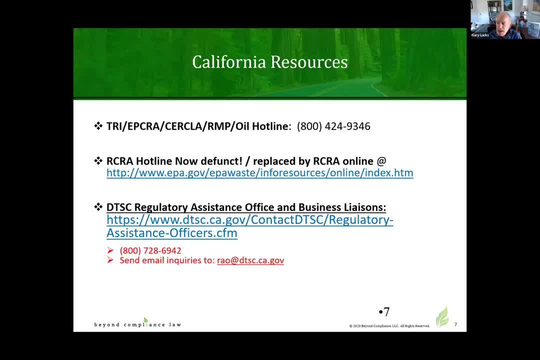 as well at a high level, as I mentioned. Unfortunately, the famous RCRA hotline, which was a real go-to resource for me earlier, is no longer maintained at the level in which it was years earlier. So there are all kinds of online opportunities to research, but not a human being who can help guide you. But 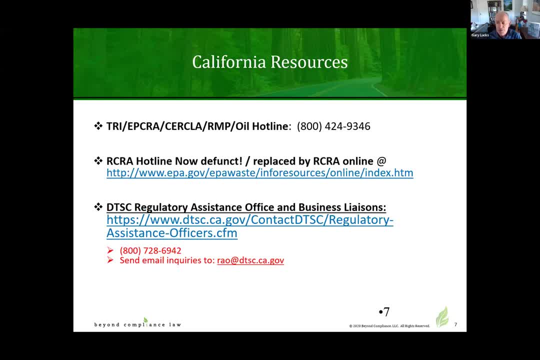 nonetheless, there are federal resources available in the second bullet here for RCRA, Of course, for the other programs above, And then here in California we have the luxury of actually being able to connect with a human being in the regions throughout the state with a duty. 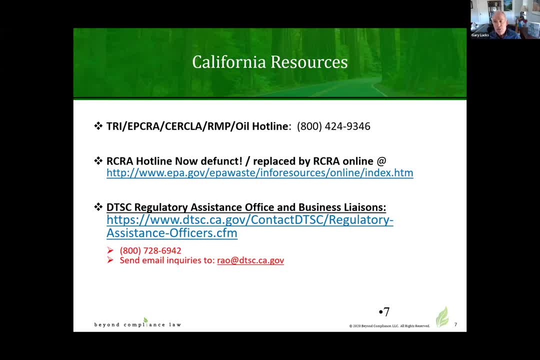 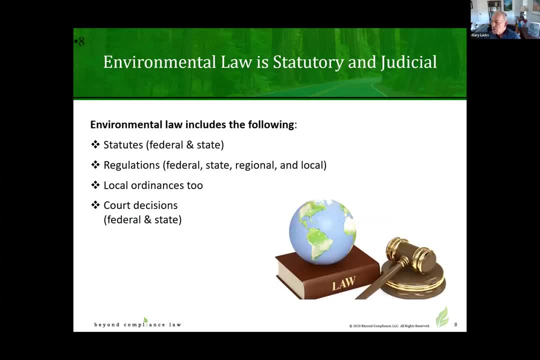 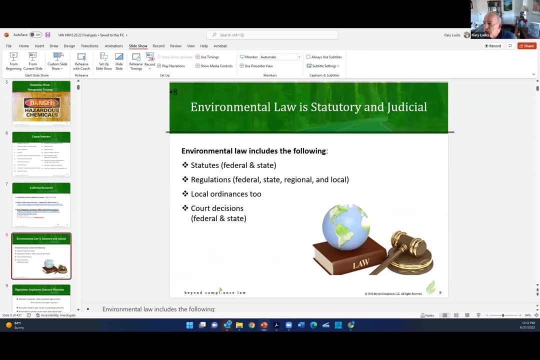 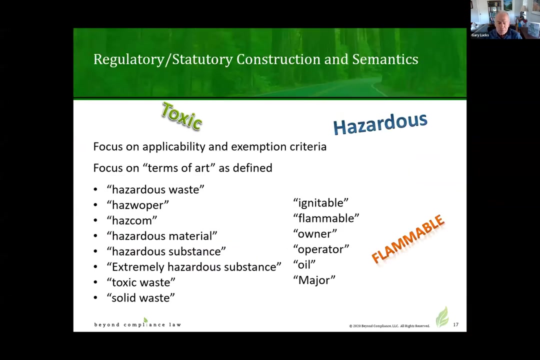 officer who can help guide you to resources and interpretations as well in California. So let's see, Did I? Okay, I think I – bear with me one second. I think I need to shift this to the custom show. Okay, Yeah, So all right. So terms of art are critical in the field of environmental. 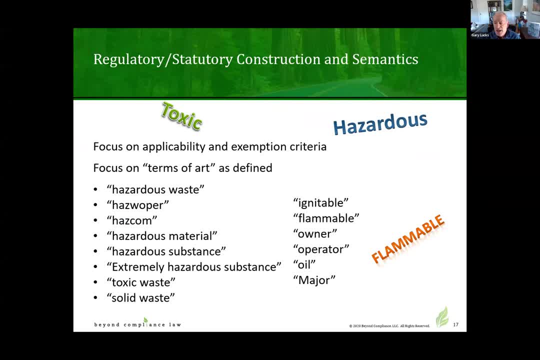 law and particularly in the hazardous waste field And, as you can see on the left-hand side, those terms all look quite similar, right? Hazardous waste, which is the theme of our discussion, is similar to HAZWAPR HAZCOM. 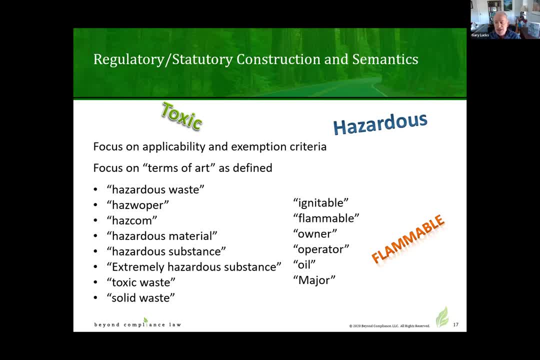 hazardous materials, Hazardous substance and so on, And every single one of those words has a distinct meaning in definitions And it's critically important to not overlook and glaze over the term and its particular connotation. So we'll touch on some of that And I can't emphasize it enough because it's often a challenge. 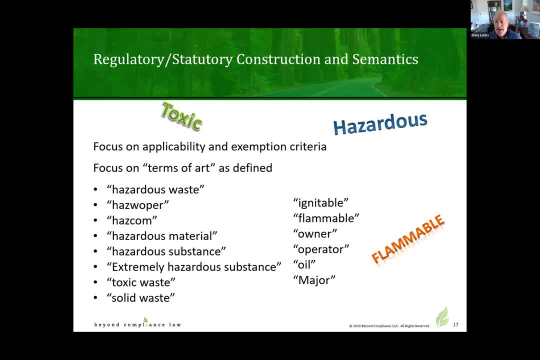 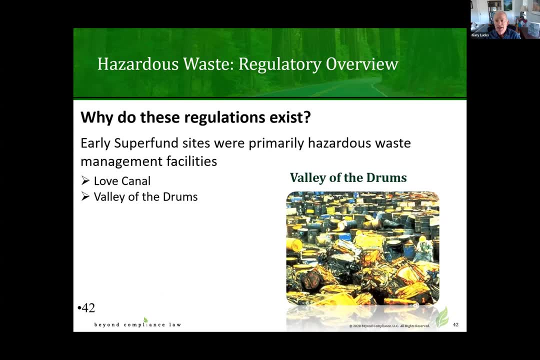 or mistake. So we'll touch on some of that, And I can't emphasize it enough because it's often a challenge that young attorneys make by assuming and not taking the time to go to the definitions. This field of hazardous waste management grew out of mismanagement over decades in the industrial 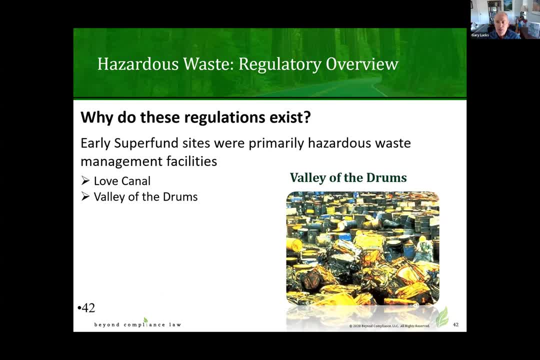 era, And so we're stuck, as many of you know, with a legacy of tens of thousands of contaminated sites across the country, especially as well here in California, from landfills that leak to industrial facilities where there are practices that resulted in solvents and other chemicals. 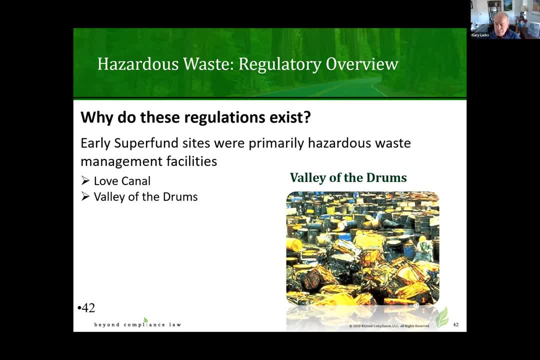 being released to the land or the water or the air, as well as a number of military bases as well. So we have a legacy of cleanup, And some of the most noteworthy ones were the Love Canal and Valley of the Drums, where, if you see in this picture, the Valley of the Drums was a notorious criminal. 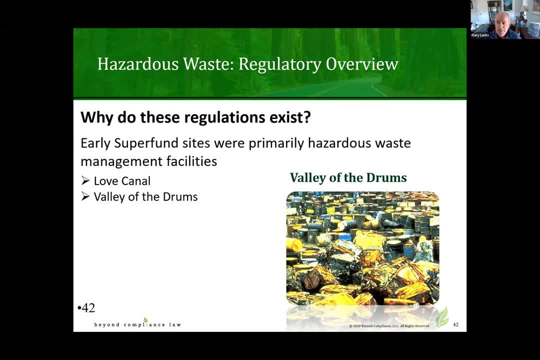 matter in Kentucky where a company collected spent chemicals in drums and containers and basically just collected them and staged them in a valley where they leaked into the groundwater and subsurface and resulted in its own Superfund site, And so out of that grew a need to try to 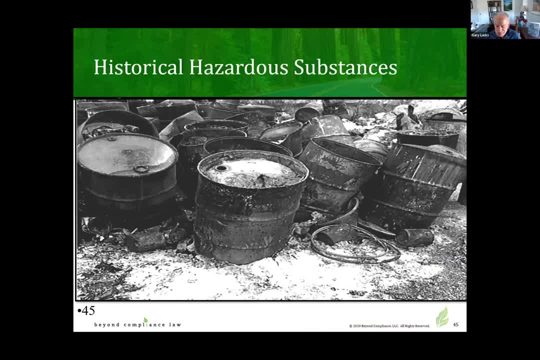 organize the management of these dangerous chemicals. Yeah, This picture is a picture a colleague of mine took just not that long ago, maybe less, maybe 20 years ago, even when the hazardous waste laws were in place. So it's a matter of rigor and 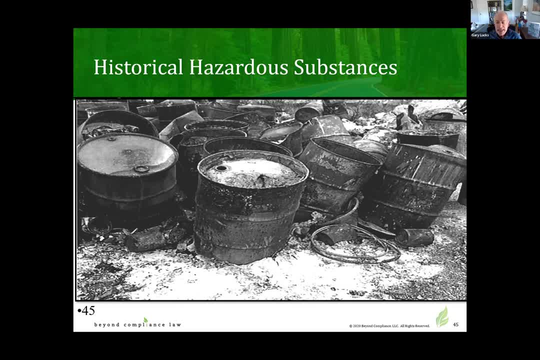 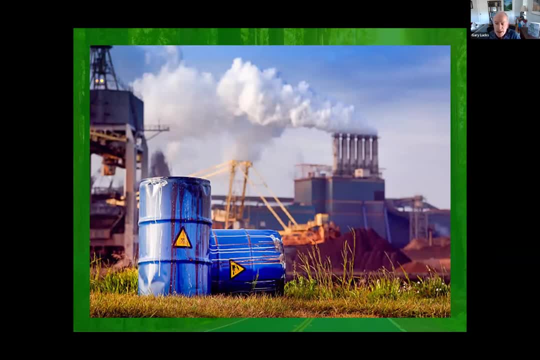 awareness to maintain compliance. So, of course, chemicals are generated from industrial processes and we'll try to decipher what chemicals are managed. in what way Are they a waste? Are there exemptions? If you have a non-exempt situation, what are the prescriptive requirements in terms of 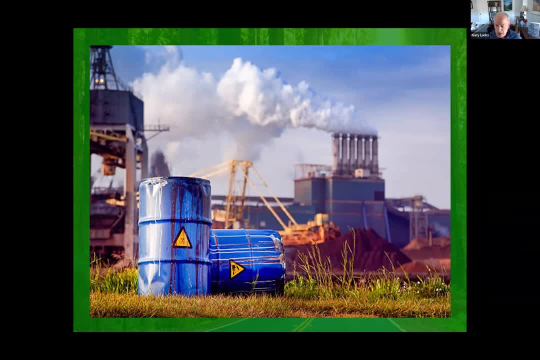 labeling, staging, how long reporting, training, transportation, all that goes into managing the waste. Because the whole idea, if you distill it down to its essence, is: we are the, the. the legislatures have essentially taken what one could refer to as common sense good. 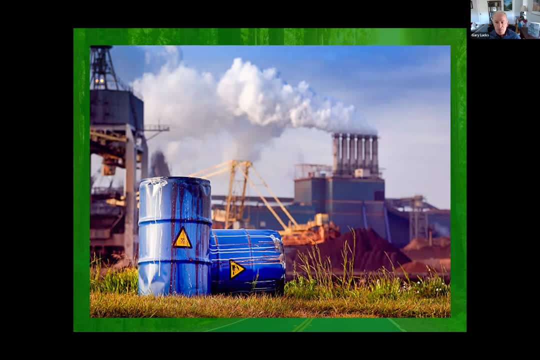 management practices, chemical management practices, and codified that, And so in other countries it's not often that the regime is focused on prescriptive rules, like we have in California and the US. They're more performance-based to ensure compliance or 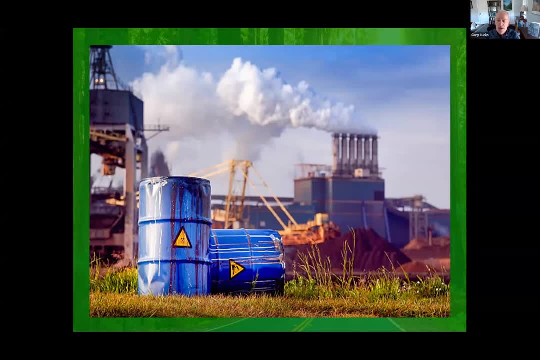 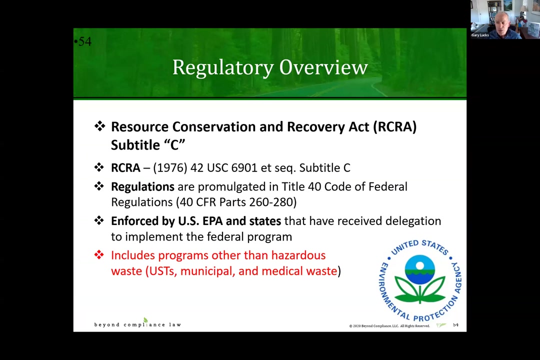 certain performance outcome. Here we focus on: who does the law apply to, what must you do, how must you do it and when must you do it. And that's really the framework that we're dealing with here, And our focus will be on the federal RCRA and the state equivalent law, And 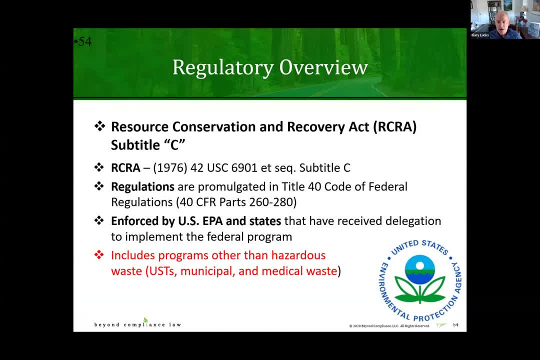 RCRA of course stands for the Resource Conservation Recovery Act or RCRA, And other people pronounce it differently, but I refer to it as RCRA, So DR KURTISLAND RICRA, a relatively old law, now several decades. It's been codified in 40 CFR and delegated to the 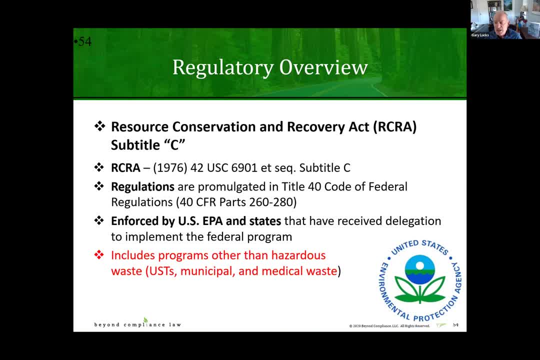 state of California. What is often overlooked is that RICRA not only covers hazardous waste management, but it covers other areas as well: managing underground storage tanks, municipal solid waste and lightly medical waste at the federal level, And so there are three major 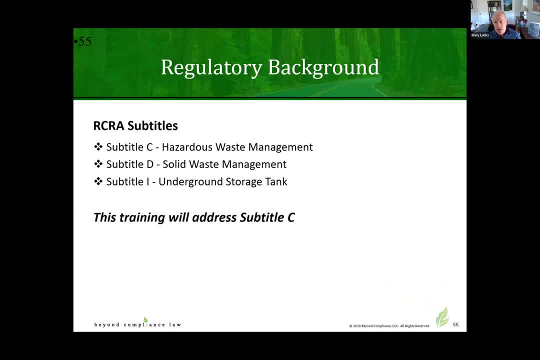 subtitles, And the subtitle C is where we'll draw our attention for today with respect to hazardous waste management. But non-hazardous wastes, referred to as solid or municipal waste, are also regulated by RICRA, but under a different subtitle D, And RICRA's subtitle I relates to management of. 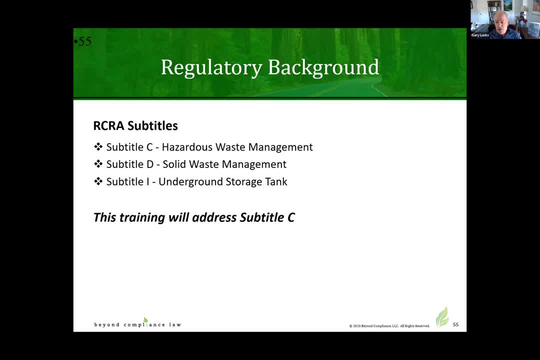 underground storage tanks That cover- and it's a little distinction, but that relate to underground storage of materials like hazardous materials or oils, but not hazardous waste. Underground tanks dealing with hazardous waste are regulated under subtitle C, not subtitle I. Everything else other than 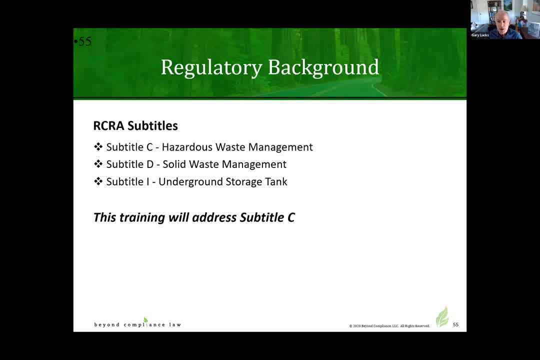 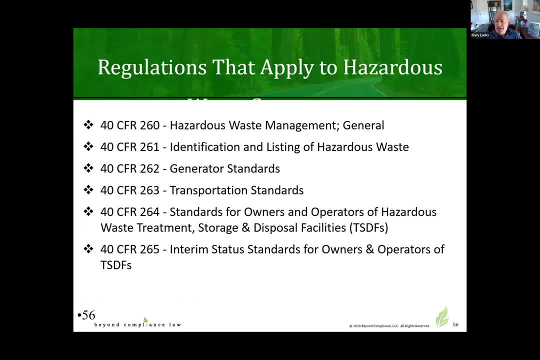 hazardous waste in underground tanks is regulated under RICRA, subtitle I. We'll focus on subtitle C. The federal regulations appear in 40 CFR, section 260 and, following When I mentioned earlier about the terms of art and definitions, it's critical to look in section 260 at the top. That's where 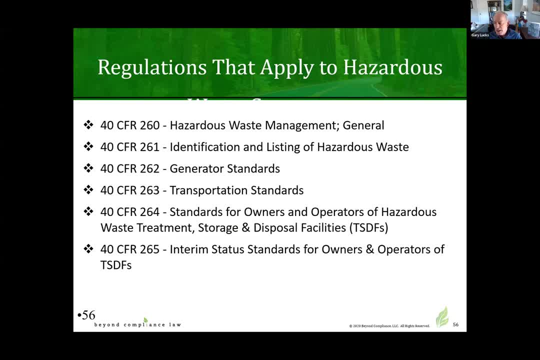 the definitions exist And, as lawyers interpreting rules and advising clients, we really have to be familiar with section 260. And it's often overlooked. as I mentioned, We'll focus today on section 261, because characterization is a big part of this And we'll cover it lightly, but 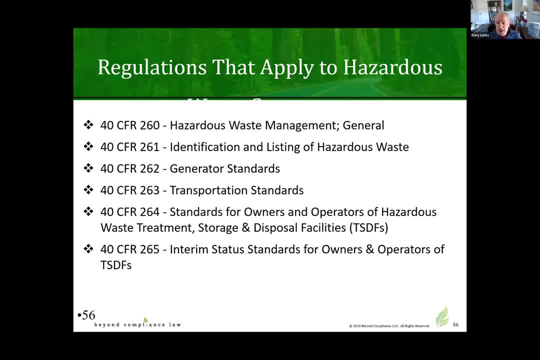 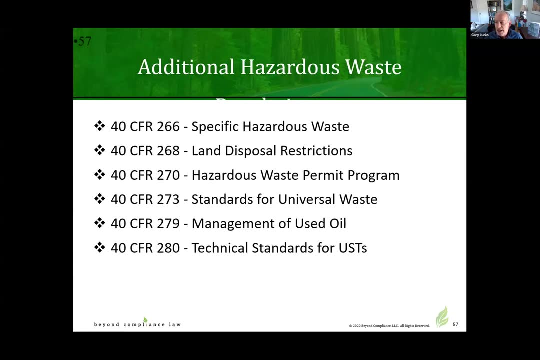 enough for you to spot the issue. And then we'll spend a little bit of time on section 262, which pertains to general generator requirements, that is, And we'll touch lightly on all the other areas. but in the interest of time we can't go there other than just to give you the headline And 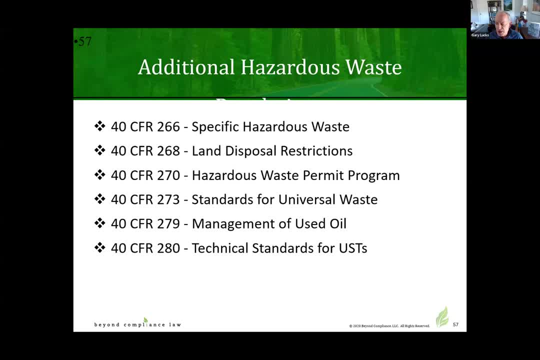 you'll see some of the other key regulations as they are listed here. Note that the last two- section 279, is a standalone requirement dealing with used oil, which under federal law is regulated more lightly, And in California we regulate used oil. 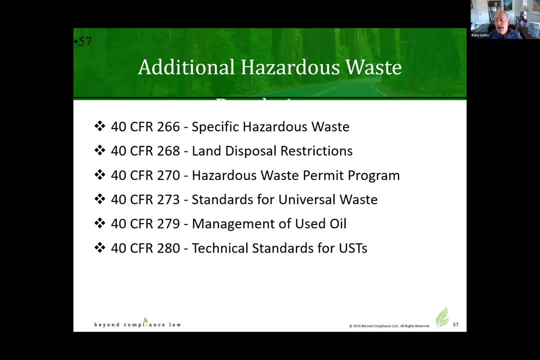 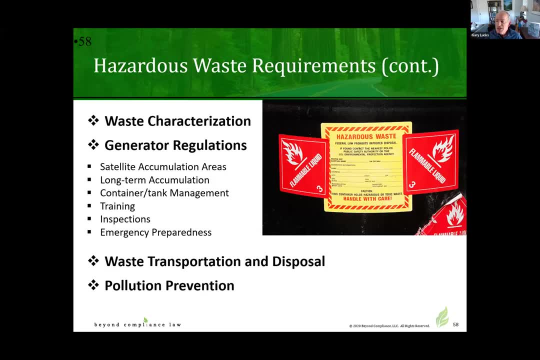 in many instances as if it was a hazardous waste. And then section 280 are the regulations that deal with underground storage tanks. So our focus again will be waste characterization or profiling, And then the generator requirements that govern what, when and how you manage your hazardous. 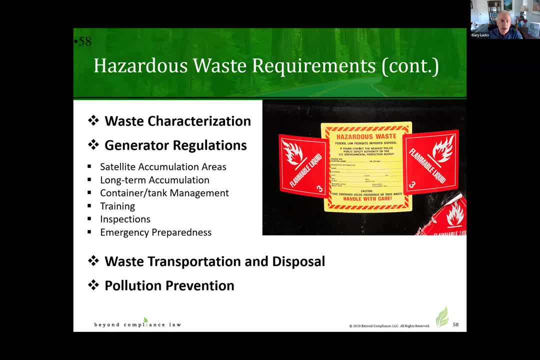 waste are in these sub-bullets here where we talk about the requirements governing near-term accumulation of hazardous waste, sometimes referred to as satellite accumulation, where you have a near-term collection But to ensure you don't have a superfund scenario we have to manage. 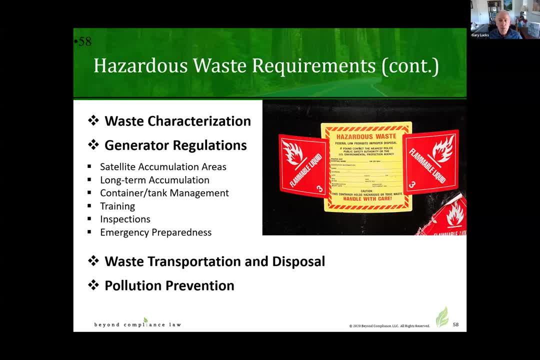 a way that they can be moved off to a more appropriate facility for long-term storage, ultimate treatment or disposal. So we'll talk about how we move chemicals from the near-term satellite to the interim staging area referred to as a long-term accumulation area, and then 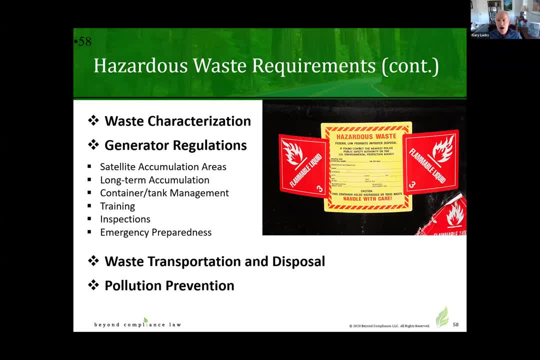 all the requirements that ensure that the containers and tanks are managed in a way where they won't result in a release of the chemical to the environment. Training, which we're doing here, is a requirement. for generators of hazardous waste There's a duty. 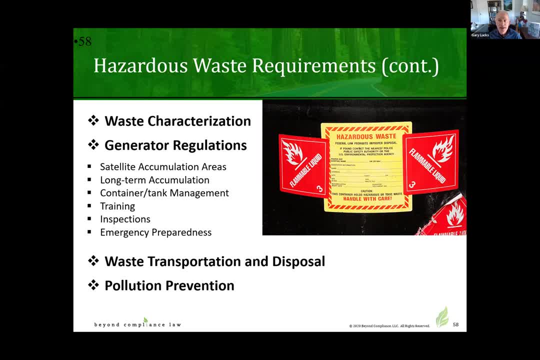 to inspect the accumulation areas and other aspects governing what to do to prevent and manage a possible release or spill. There are other requirements governing the shipment of hazardous waste, which we'll cover lightly, and pollution prevention, which we'll not really cover at all in. light of our time. It is a critical requirement to ensure that the containers and tanks are managed in a way that is effective. and it is a critical requirement to ensure that the containers and tanks are managed in a way that is effective. and it's a critical requirement to ensure that the containers and tanks are managed in a way that is effective. 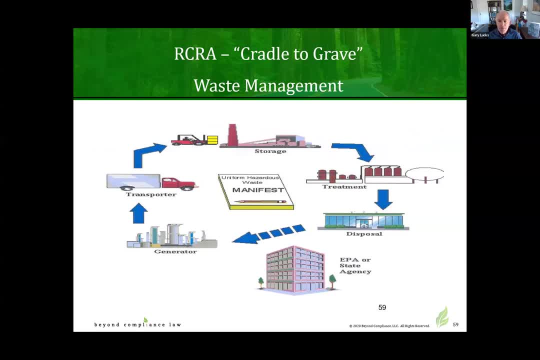 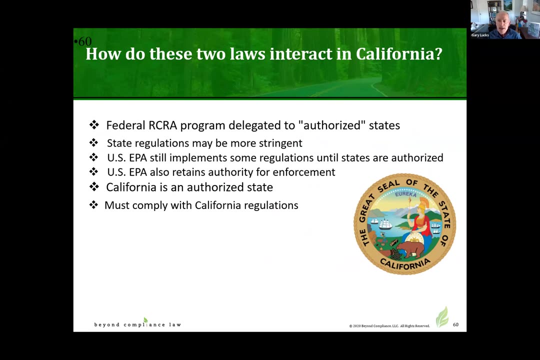 And then there's the cradle-to-grade scenario, where we want to very tightly regulate the waste, from the moment it becomes a waste to its ultimate destination, And so in California, we are delegated authority from US EPA to implement this federal RICRA. 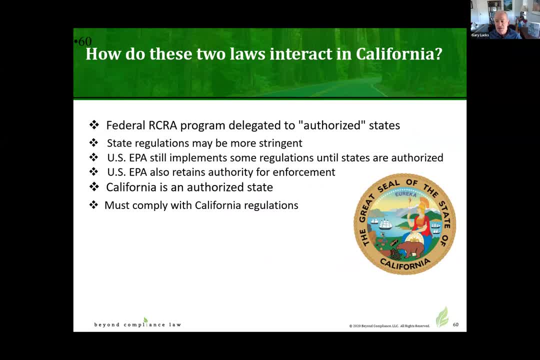 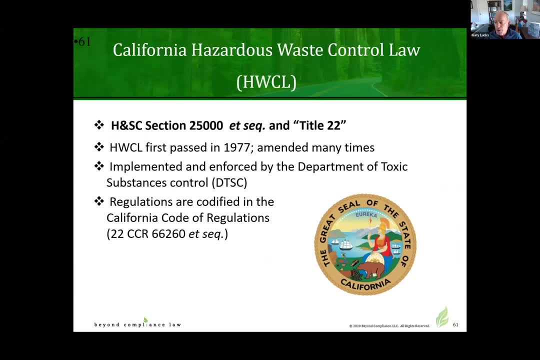 program, which I'll begin with and I'll talk about how California's different along the way. So we're an authorized state And the vast majority of states are authorized to implement the federal program. The agency of course that is responsible is the California Department of Toxic Substances Control, DTSC, which interprets the California Health and Safety Code, which is the repository for those federal rules in Section 2500.. 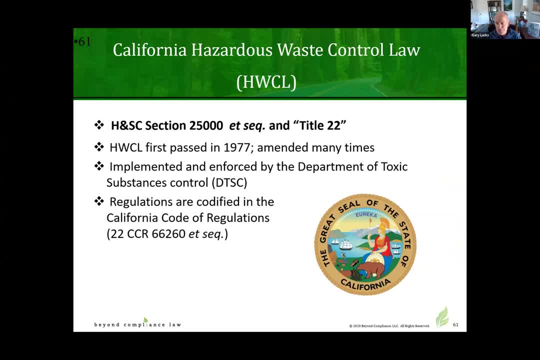 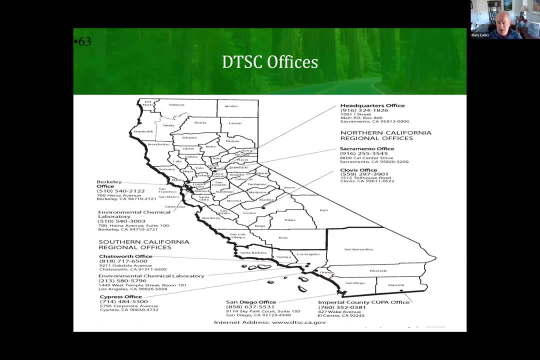 And then that's the statute, the regulations in Title 22.. And we'll talk shortly about the subordinate agencies that further implement the DTSCs. the Department of Toxics program, The DTSC, the Department of Toxic Substances Control, is headquartered in Sacramento and there are several regional offices that serve the regulated industry in implementation and enforcement at the state level. 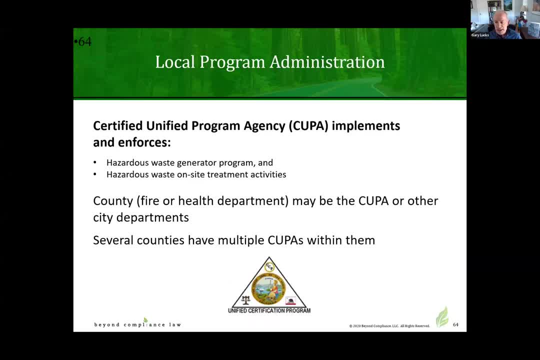 Because of the complexity of the state and its scale, the law changed several a couple decades ago to delegate the program further, from the Department of Toxics down to the city and county level, where the CUPAs, the Certified Unified Program Agencies, implement the hazardous waste program in two functional areas. 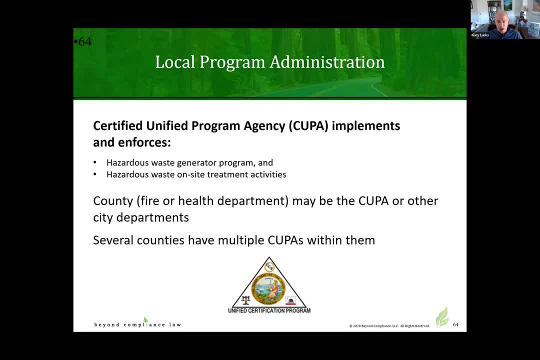 One, the hazardous waste generator program, the cradle-to-grave function I mentioned, and then also selective on-site treatment, referred to as tiered treatment, which we'll cover lightly a little bit later. But essentially the CUPAs are kind of all over the map. 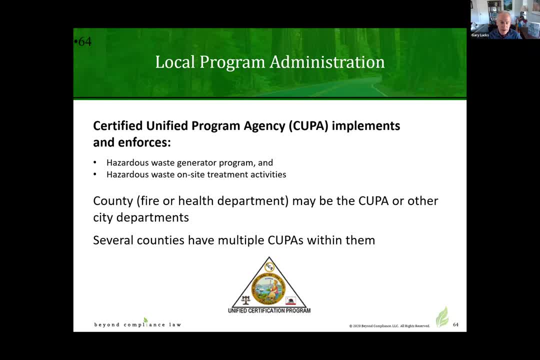 There are well over 100 of them in the state that represent counties or cities or several cities within the county, and they're either the city fire department or county fire department Or, in some cases, county environmental health departments. There are several different flavors of CUPAs. all that further implement the federal law that goes down to the DTSC state level and ultimately down to the county or city level. 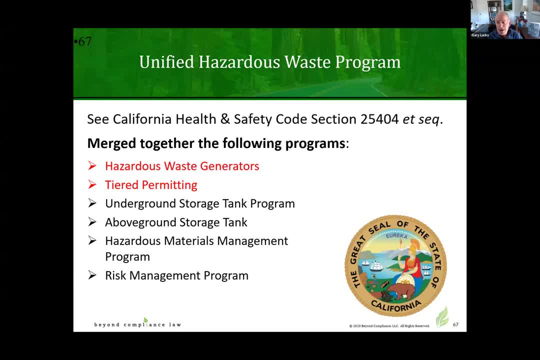 So those CUPAs, as some of you may know, not only regulate hazardous waste generation and tiered permitting, but they also regulate other areas at the local level, From underground and above ground storage tanks to non-hazardous chemical management, referred to as the hazardous materials or products programs, and then risk management program, dealing with preventing accidental release of highly hazardous chemicals. 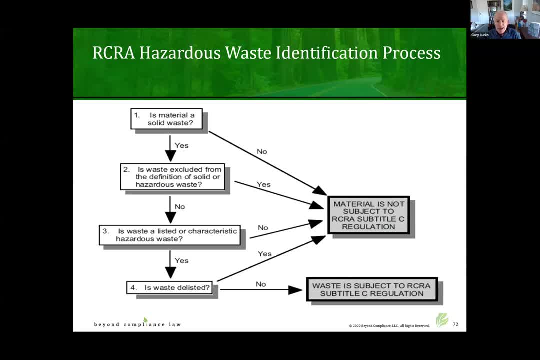 So let's begin by looking at whether there is a hazardous waste to begin with, because there's all kinds of waste in terms of types and volume. So let's begin by looking at whether there is a hazardous waste to begin with, because there's all kinds of waste in terms of types and volume. 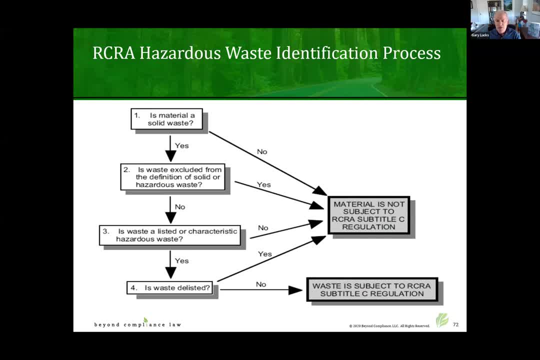 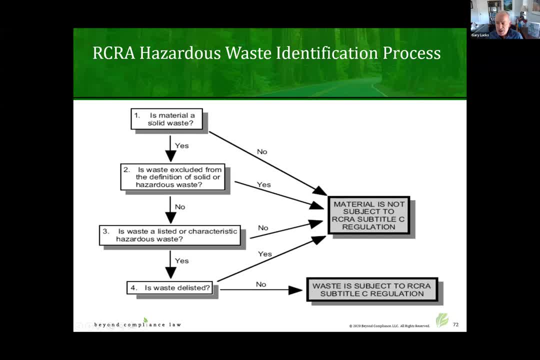 And we'll see that there's a lot of different ways to look at it, And we'll see that there's some semantic challenge with the word solid waste, which I'll get to in a moment. But for our purposes now, the question is: is the substance, is the material, a waste? 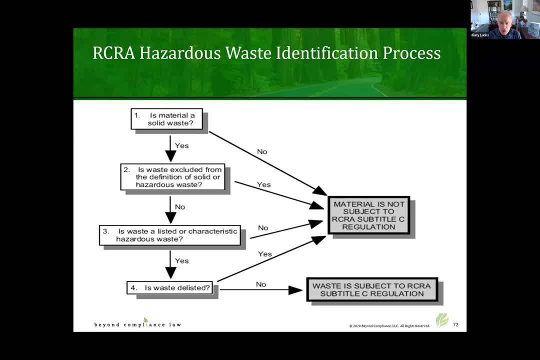 And if so for you. is it your desire to no longer use this material and it's waste to you? And then we ask the question of if it is a waste, are there exclusions, exemptions that allow you to not have to? 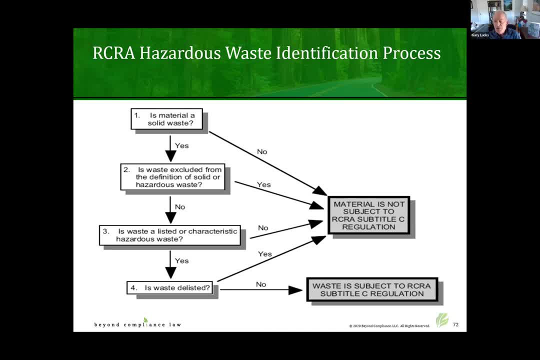 manage it as tightly as a hazardous waste Or if there's no exemption, then you ask the next question in item three: what flavor of the waste is it? Is it a characteristic waste, which we'll see includes any waste that exhibits a characteristic of ignitability, corrosivity, toxicity or reactivity? 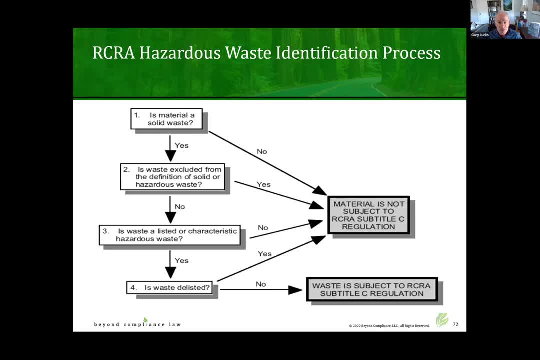 Is it characteristic, And if so, then it's a hazardous waste, And if so, then it's a hazardous waste, And if so, then it's a hazardous waste for that characteristic, one or more characteristics. It may not exhibit a characteristic per se, but it may appear on a list of chemicals that, when they're wastes, 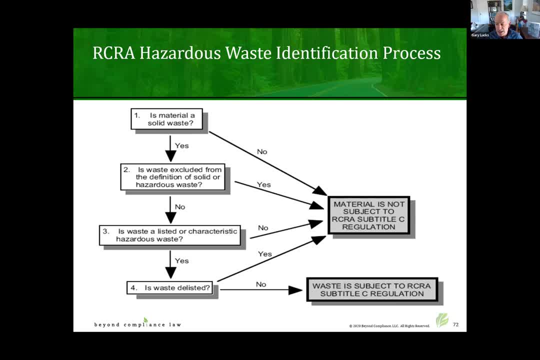 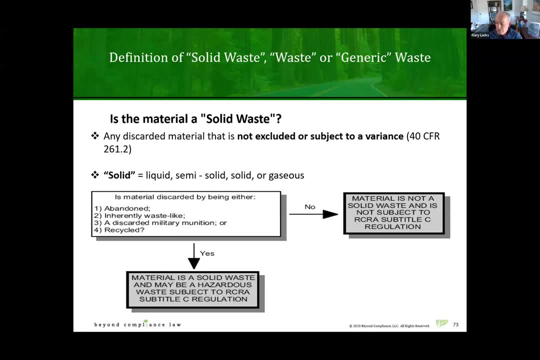 they are automatically managed as a listed hazardous waste. So that's the big picture of how we manage or determine whether we have a hazardous waste to begin with, And so I mentioned earlier that the definition, the terminology at the federal level is: is the substance, is the material- a quote: solid waste? 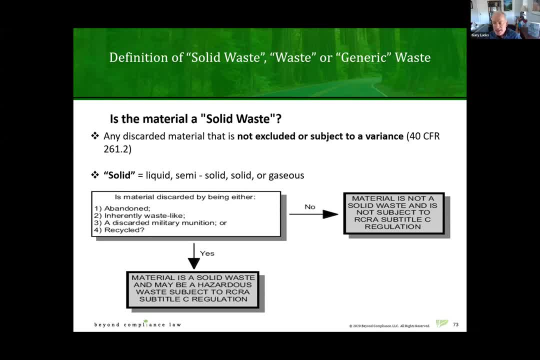 And back to definitions. we have to look at the definitions, And the definition of solid, sadly, was not written by a scientist. It was written probably by a lawyer, And solid is defined to mean more than solid. It means something that happens to be liquid, semi-solid or solid or gas. 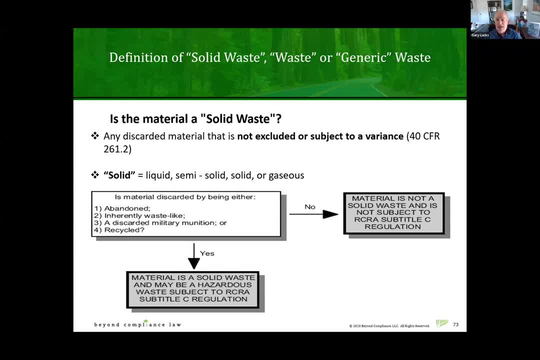 So It's absurd the way the definition appears, but we're stuck with it, And so just you may have something that's a liquid, that is also, by definition, a solid waste, which of course is absurd, but that's kind of what we're stuck with. 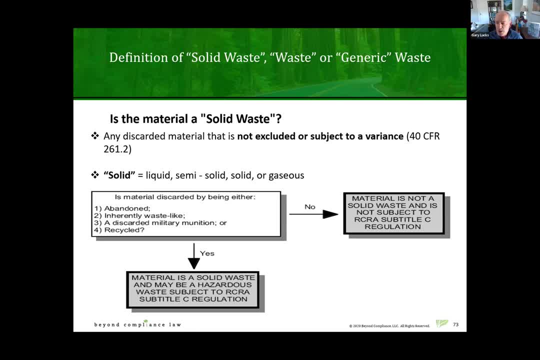 So we look at the definition and we also ask whether it's a waste. and waste is defined as something that's abandoned, inherently waste, like a discarded military munition or something that is destined for recycling, And there's a lot of nuance and a lot of depth, and I'm often advising clients in the weeds on these definitions because, you know, ultimately we have to comply with the regulatory standard of whether we have a hazardous waste or not, and if there's an argument for it to be managed in a lighter way, then you can make that argument, but you've got to dive into the weeds to do that. 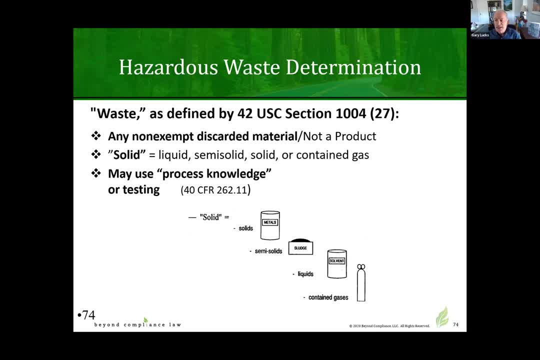 So the definition of a solid waste is, As I said earlier, liquid, semi-solid solid or gas, as you see illustrated in this picture here. So any material or substance that exhibits is in any one of those phases of reality could be a hazardous waste. 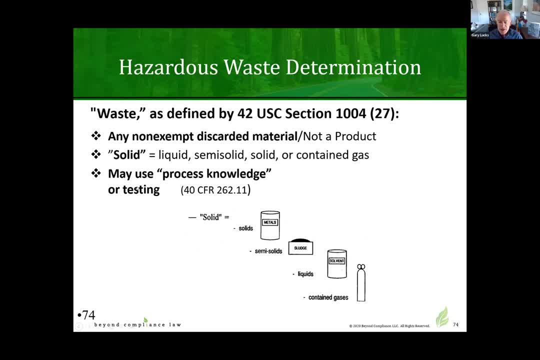 And we determine that either by testing using laboratory tests or our process knowledge, because we know what we started with, We're familiar with the process, We know what we're going to end up with. So we have two options We can- it's cheaper to use process knowledge but and more expensive to send out samples to a laboratory for testing. 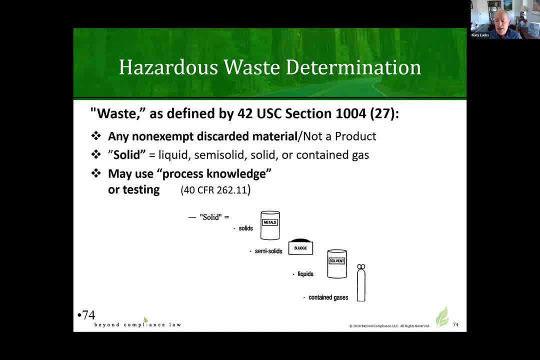 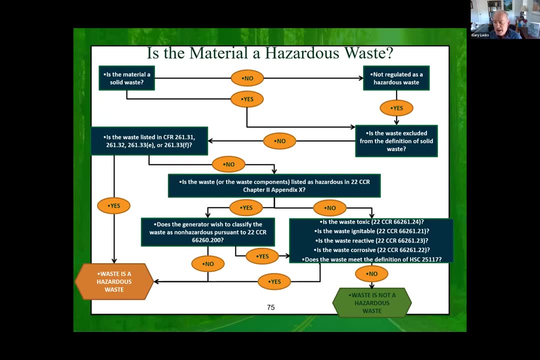 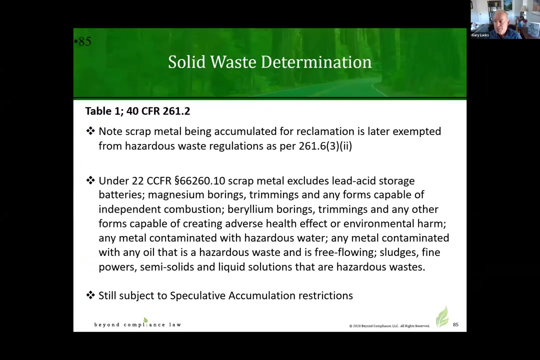 But in some cases we may want to send something out for testing to be absolutely sure and pay the money because getting it wrong could result in significant fines. This this is not meant to confuse you, but this is actually my attempt In my book to show how we run through the analytical process for the California hazardous waste profiling exercise. the federal process is challenging. the state process is even more challenging and we'll see. that is because there are fewer exemptions under California law and more opportunities for a waste to be considered hazardous waste under California law than under federal law. 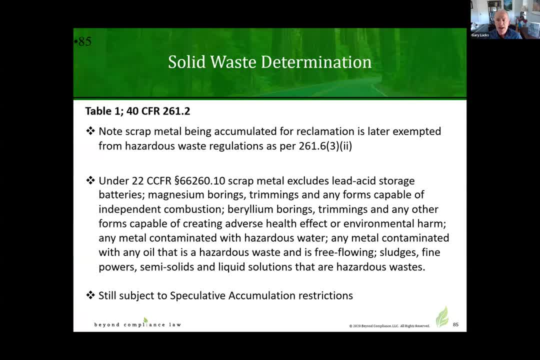 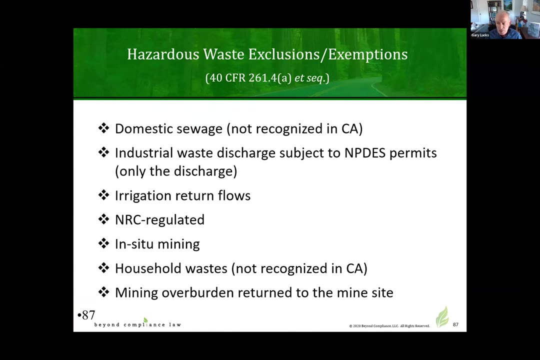 And the next couple Slides just point out that there are a number of exemptions. So even if you have a solid, semi solid, liquid or gas material that you consider to be a waste, Then you have to ask: well, can I at least enjoy an exemption? And there are a number of exemptions, like scrap metal under certain circumstances, or domestic sewage- under federal law but not in California law, or waste that is a hazardous waste but it's going through a pipe pursuant to the Clean Water Act permitting, then there's a lot of exemptions. 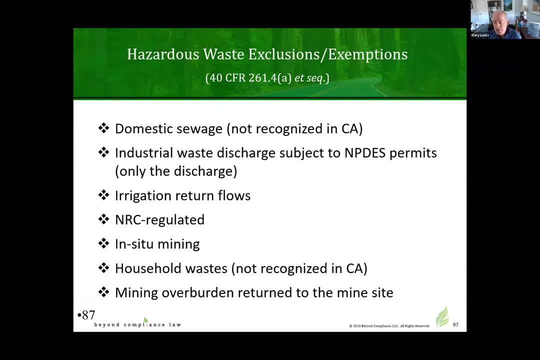 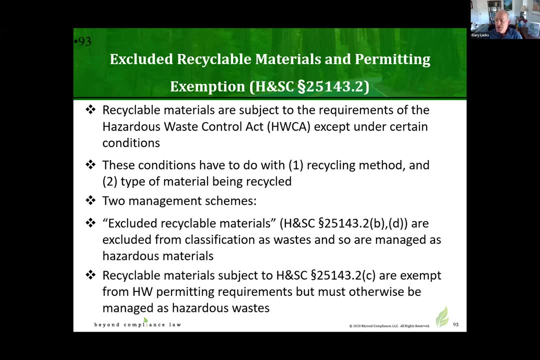 That is captured under the Clean Water Act and other examples of mining waste known as under the devil amendment and others. so there we have to sort of walk through the exemptions and the definitions to work our way to an outcome, And so there's a very important California exclusion. that is, I think, the most complicated exemption and convoluted leave drafted statute I may have ever written. 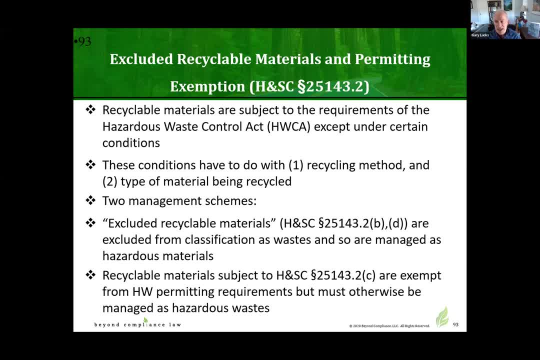 And it is referred to as health and safety code section 25 143.2,, which is a state statute that allows in some cases for a material to be reused, reclaimed and repurposed. So again, it's not trash, it's treasure, And but to enjoy that 25 143.2 exemption. 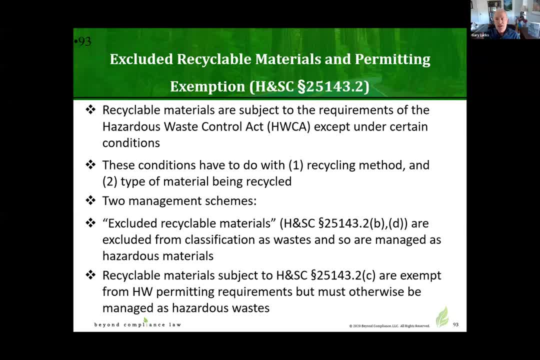 It's a real challenge to walk through the exemptions and exclusions and exclusions or exemptions to ensure that you can actually enjoy the more relaxed regulatory requirements. I'm just introducing it as an issue here. we could spend hours walking through it, but it is something that I spend some time with and have done a lot of work with with clients, and it's something to be alert to. 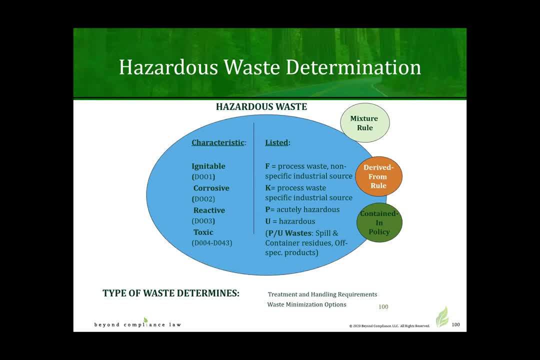 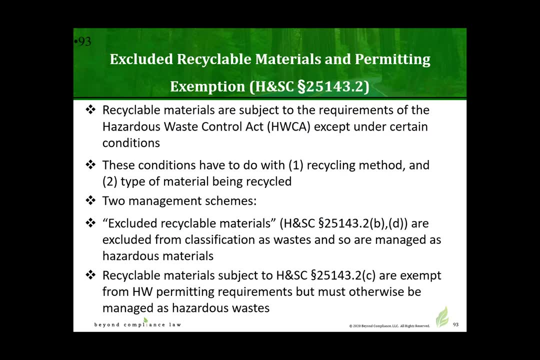 Yes, I see that. Yeah, there's a Actually a question for you on the exceptions. Maya Jorgensen wanted to know: are there other examples of exemptions under California law for policy reasons? and so you gave us the example of the recycling which is a little complicated. to make sure you qualify. 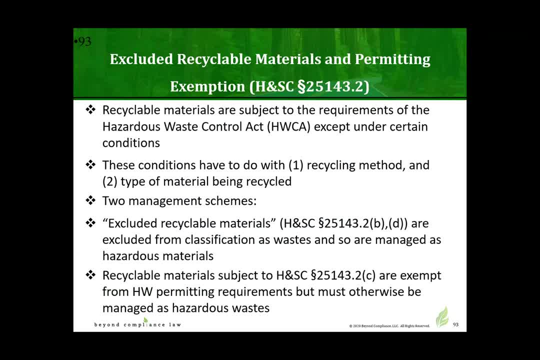 And she specifically was asking about CO2.. Can you answer those? What was that? last part was just specifically asking about. what she wanted to know is a CO2.. Oh, under California law? My understanding is that CO2 is exempt under federal law despite corrosive properties when commingled with water. 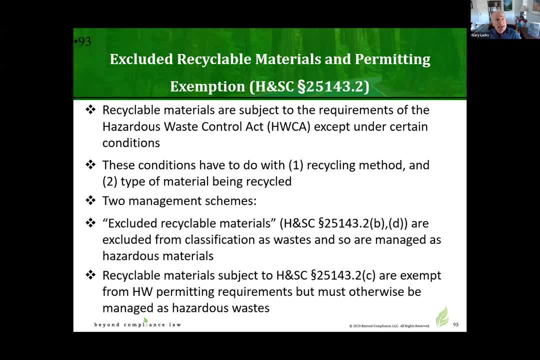 That's really interesting. so this. so the specific question is: is carbon dioxide, the greenhouse gas, a gas? so it's a solid, if it's a waste, Solid, semi solid, liquid or gas, that's a gas Is it. if it's a waste, Is it exempt? I'm on. I'm unaware of any exemption. 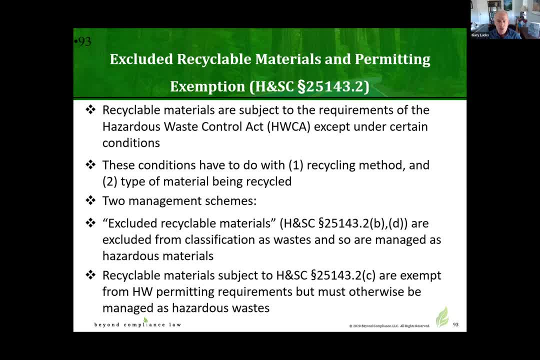 I'm aware of any exemption for CO2 under the state or federal hazardous waste law And so see if, in theory, if you could, if you could capture the CO2 in a storage vessel, then- and it's contaminated, it CO2 ended up itself would not be hazardous. 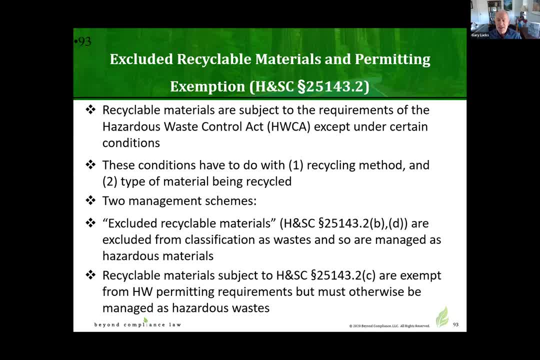 We'll see later that it's not corrosive for our purposes. It's not reactive, It's not It's not, It's not toxic And it's not on any list so it would. It's unlikely that CO2 would be hazardous waste unless it was cross contaminated with something that was toxic, corrosive or meet any meeting any one of these other requirements or other definitions. 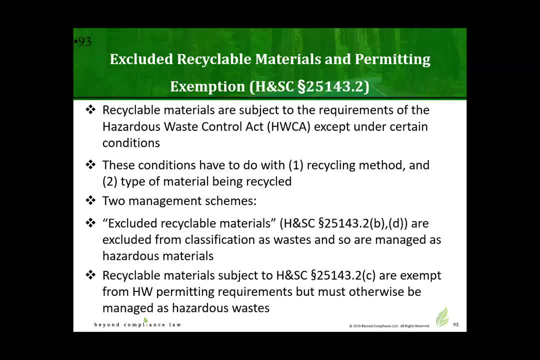 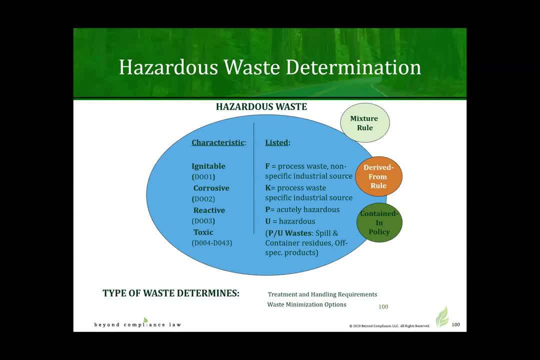 Any other questions there? Marissa, Yeah, I think. maybe just to wrap up this section. Ellie Oh wrote wrote in the chat. Do you have any suggestions for resources to better understand the exemptions? Yeah, are, there are good places. if people are curious, they're. they're looking at their waste and they're trying to figure out. 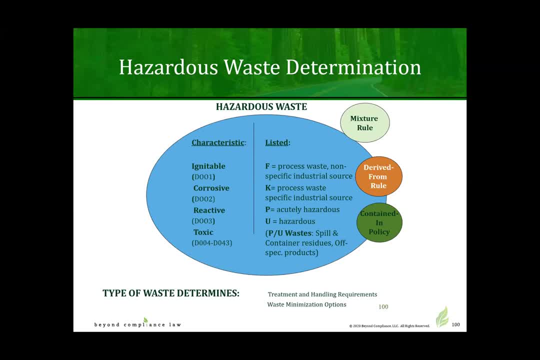 Does this exemption or exclusion apply? where would they go? look, Yeah, that's a good question. So I think my our book is too high level for that. I think the California environmental law and land use treatise is probably a really good start. 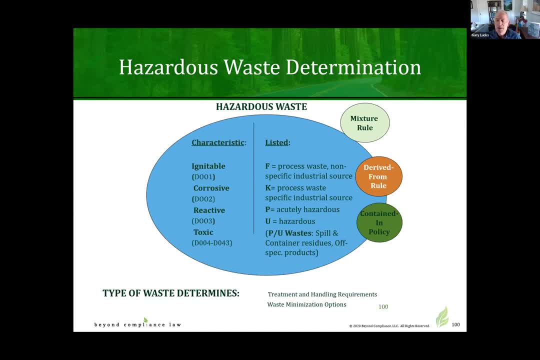 And if Ellie- who I believe is the name- wants to email me, I have my my contact information at the end, but it's Gary at beyond compliancenet. Gary at beyond compliancenet. I've got some other books on my bookshelf I can share as well. 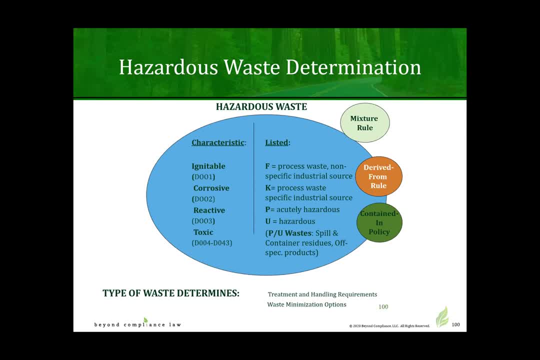 Great, Thank you. Yeah, So this picture illustrates the big picture of If, of determining whether the non exempt material that we now refer to as trash or waste is a potential flavor of a hazardous waste. And you see, on the left hand side. 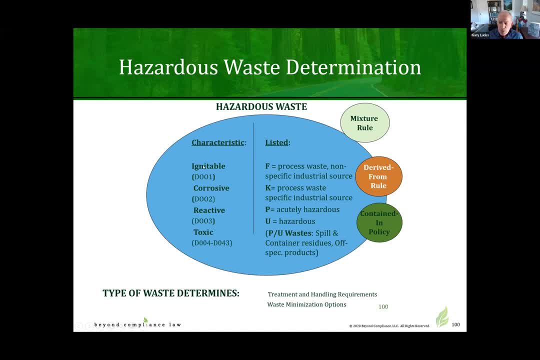 There are the three characteristics: If the material exhibits characteristics of ignitability, The risk is obvious: corrosive, reactive or toxic, Then by definition it's a hazardous waste, must be managed with all these prescriptive detailed requirements and must be labeled accordingly. And this is not. This is an ad, not an or. it could also be a waste that appears on a list and there are different categories of lists, referred to as process wastes that are 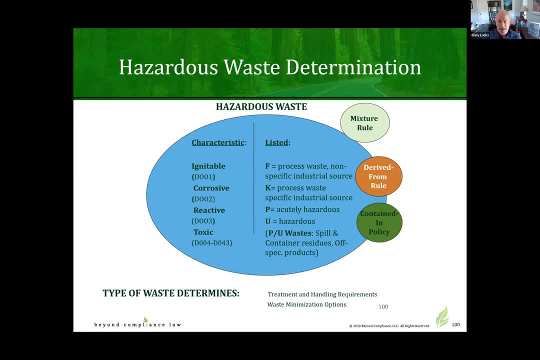 In fire waste Anyways, bro忾 Wha or not, bodies and who are generated in industrial activities, like solvent degree seeing ways, for example, and that the referred to as, as as in Frank waste, K waste are also processed waste that are generated due to the process. 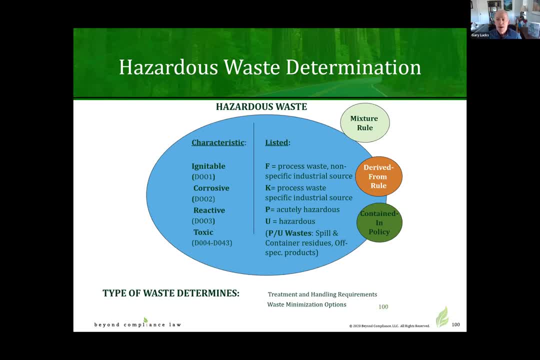 But those ways are unique to different industry types- Michael Mann pharmaceutical industry- and they are peer under K wastes, so you could have an ignitable, corrosive, reactive or toxic Michael Mann waste, one or more of them. that happens to be also a process waste in an industry category category or generic industry, and so we have to identify all. 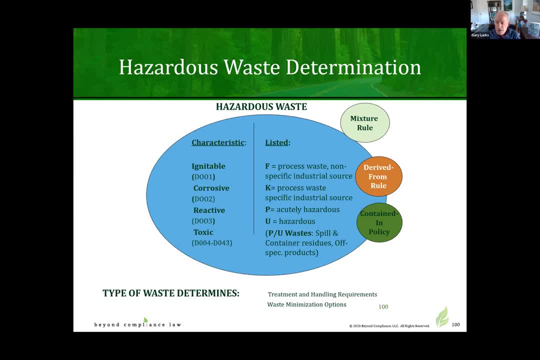 Michael Mann scenarios in which the waste is considered a hazardous waste. and then we look here on the P and the you wastes. there are hundreds and hundreds of chemicals listed, Michael Mann, In the regulations under what we call the the you wastes, and these are chemicals that you can buy from a supplier and they're not waste due to a processing activity. they become waste because 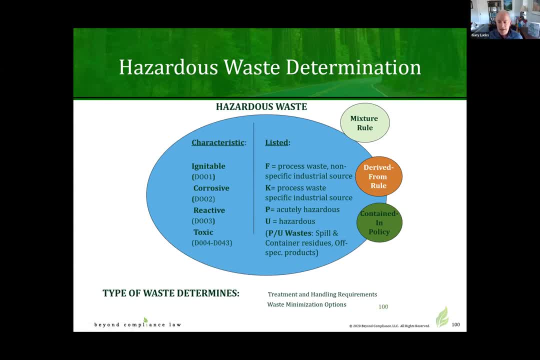 Michael Mann, You spilled it, and now it's like spilled milk: you can't use it. so it's a material that was not processed, but it was spilled, Michael Mann, Or it was a material that sat on the shelf for ages and started breaking down and was not. 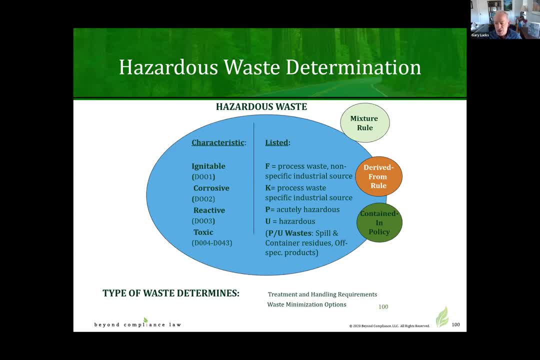 Michael Mann No longer efficacious for its intended use. so a container residue would be something that, again, is not due to processing but due to aging, that it became a waste. and finally, if you have Michael Mann- And I missed, but that's all- spec product, excuse me- and a container residue is a situation where you start with, let's say, 55 gallons. you use 45 of those gallons. you've got 10 gallons left. 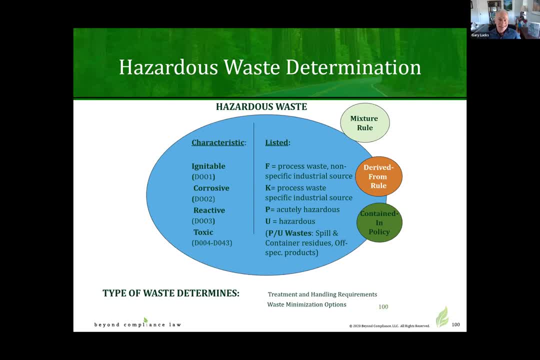 Michael Mann And your project done, Michael Mann. You don't need, Michael Mann, The other 10 gallons. it's a waste for you and you never process that. 10 gallons is just left over residue, Michael Mann. And now what do I do with it? you know it's, it's the last couple ounces in the spoiled milk we got. you're going to get rid of it. 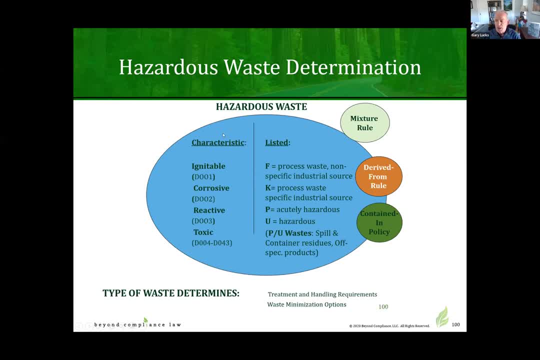 Michael Mann. So these are the ways in which these are the big picture descriptors of the flavors of hazardous waste, Michael Mann. And then we'll take a look here, the the mixture. if you, in many cases, if you have a hazardous waste, let's say you're right- by a swimming pool. 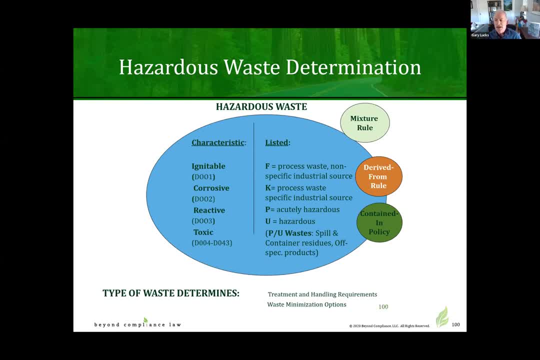 Michael Mann, And somehow you dump the 55 gallons of your toxic waste into the swimming pool. well, now you've mixed, now you've co mingled and now the swimming pools contaminated- and it's a mixture in many cases, depending on the situation- or 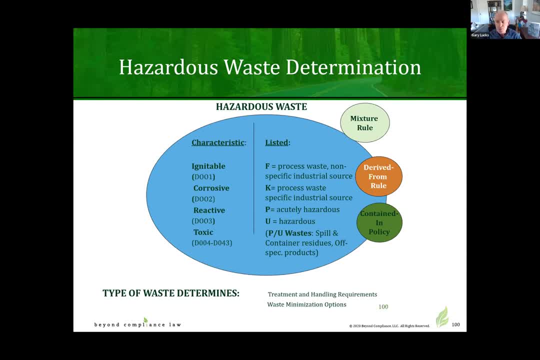 Michael Mann, You under the derived from rule. Michael Mann, You take a characteristic listed or and or both hazardous waste and you treat it to make it less dangerous. Michael Mann, Either through less harm or smaller volume, and the treatment process yields a benefit, but it also generates a more concentrated filtrate in a filter. 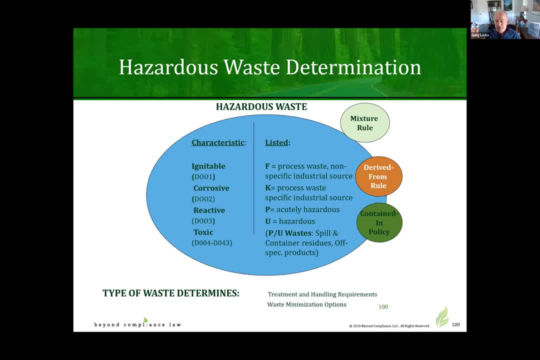 Michael Mann Using a filter. so what's the concentrated filtrate, for example, would be derived from the treatment process and therefore is a hazardous waste, Michael Mann. And lastly, if you have a hazardous waste, let's say you've got a chemical truck driving. 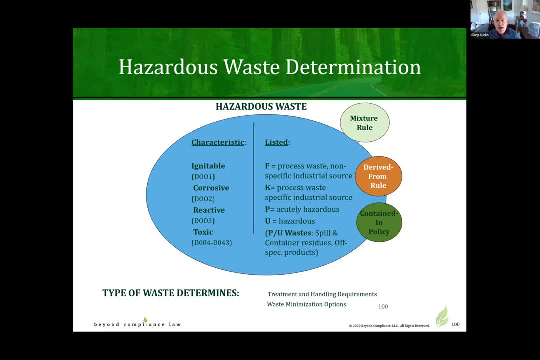 Michael Mann On the on the road. it's not a, you've got a pure chemical of methyl ethyl ketone. it's going, it's on and route to a factory truck. gets into an accident. the truck turns over, Michael Mann, The 55 gallon drum of the solvent spills into the environment or nearby stream or creek. well, now you have a mixture in the contained in the natural environment that makes all the contaminated soil 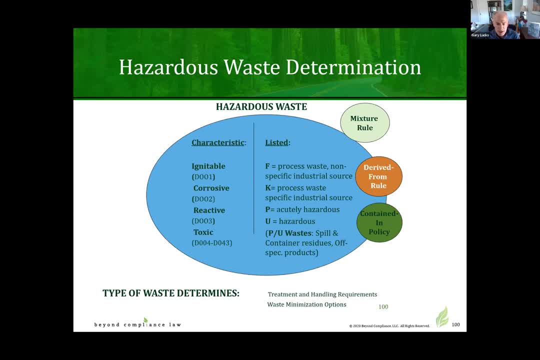 Michael Mann, And groundwater or surface water also contaminated. so now you have a commingled, larger problem, not so much in the pool where you, you know, you've mixed it, you, Michael Mann, it's actually in the environment as well. so that's the big, big picture and honestly, we can spend three hours go into depth, but i'm going to just go lightly here. so 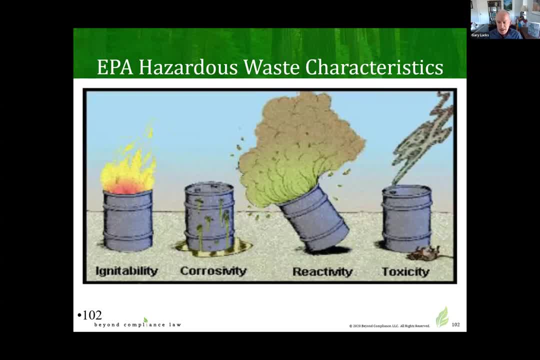 Michael Mann. Another look at the characteristics: Michael Mann. There you know something that's Michael Mann, Michael Mann, When we'll see later that that has a lot to do with what's called the flashpoint. something that's corrosive, that's either strongly acidic that burns your skin or tissues are strongly corrosive and does the same. something that's reactive, that can cause a. 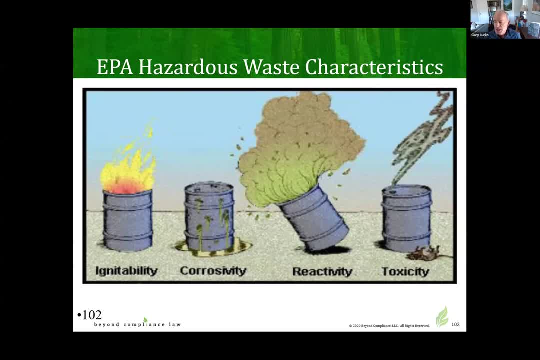 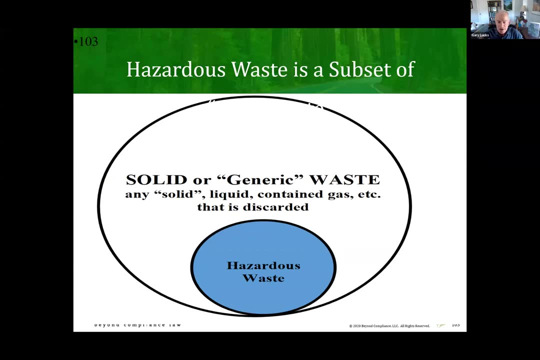 Michael Mann, explosion or a vapor cloud, a toxic vapor cloud, for example, or something that is just toxic, that can cause, Michael Mann, reproductive harm. Michael Mann, or chronic health issues. Michael Mann, If we look down, looking in the plan view, looking down at a trash, can we throw all kinds of things into the trash, and some of those things are benign ish and some are not, and we're only focused on that subset that meets the definition in the blue dot we looked at earlier. 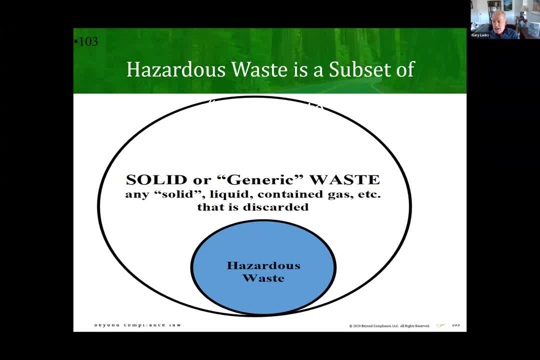 Michael Mann, With the characteristic enlisted definitions. and so if we, Michael Mann, fail Michael Mann, Any of those definitions, then then that portion of the waste stream must be managed as hazardous waste, Michael Mann. But of course, much of what is discarded is not toxic. reacted, corrosive toxic are listed or mixed or derived from, are contained in and, as a result, if it doesn't meet those definitions of hazardous waste or it's exempt, then it's in this white band and can be managed in other. 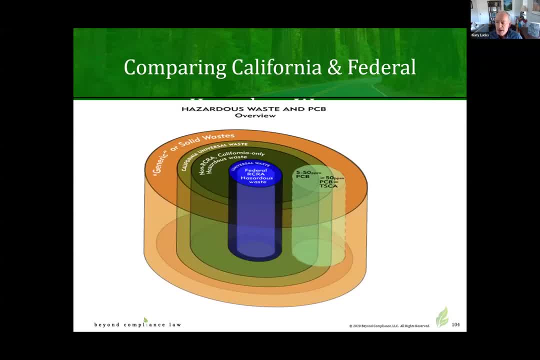 Michael Mann Ways less, less rigorously, Michael Mann, And in California, if we, if we focus on the blue dot in the middle of this imaginary trash, can, Michael Mann, The federal definitions which i've just shared with you determine what you have? a hazardous waste. 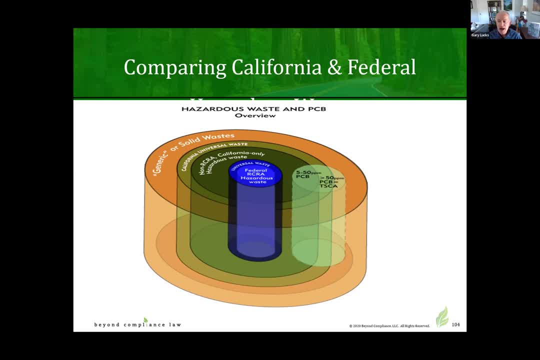 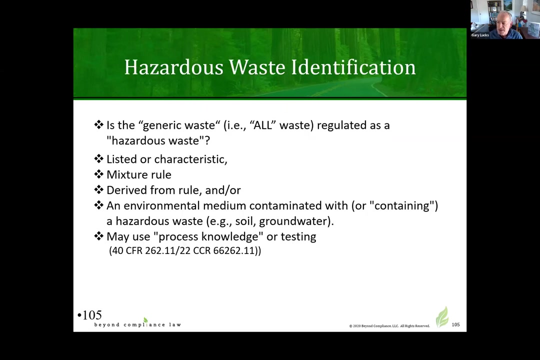 Michael Mann. Under California law we have what is known as non record California only hazardous waste in the brown larger band Michael Mann. And the point here is something may pass the definition of the federal Michael Mann hazardous waste and not be regulated, but fail the California more rigorous standard and be regulated. so we'll see examples of where that fits in a little later. 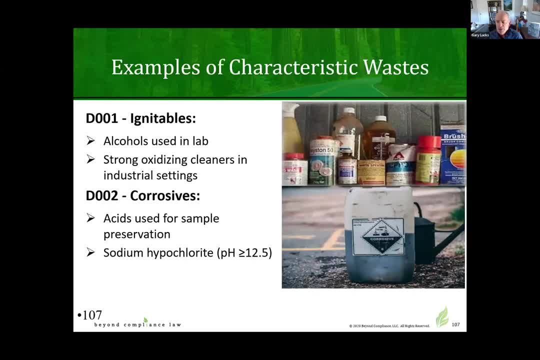 Michael Mann. So we've covered the slide already. just to give you a rough illustration, ignitable wastes can be something that's highly flammable or something that is a strong oxidizing agent, and an oxidizer basically adds more oxygen, Michael Mann, To the chemical reaction, to to the fire, that is, to to make the a, the the fire risk more amplified. corrosives. as I mentioned earlier, there are very talk, very acidic chemicals like 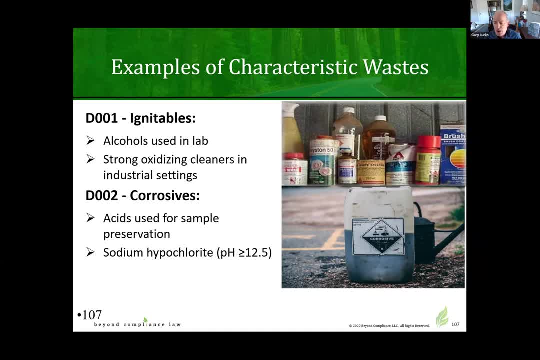 Michael Mann. nitric acid or sulfuric acid or sodium hypochlorite- very basic, and sodium hypochlorite is used. Michael Mann To Michael Mann. bring about, Michael Mann, potable drinkable water to kill, kill the pathogens, but nonetheless it's still waste. type of hypochlorite needs to be managed accordingly. 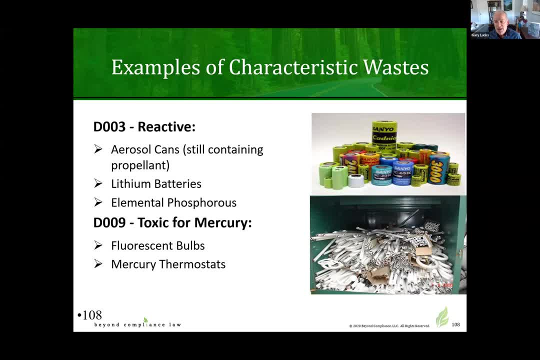 Michael Mann. reactives are. even aerosol cans are reactive. lithium batteries that are in our electric cars are Michael Mann, can be reactive and very hard to manage a fire from a lithium Michael Mann source. Michael Mann. And then mercury is an example of a toxic, and mercury is a neurotoxin that is found in our fluorescent light bulbs and also found in our our 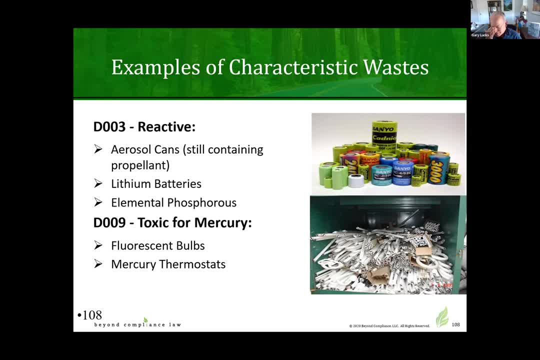 Michael Mann Are the new generation of light bulbs that. see that Michael Mann- I can't think of the name, the Michael Mann, Not the Michael Mann incandescent bulbs, but the other, you know, Michael Mann bulbs. they have mercury and it's methyl mercury and it's gases. 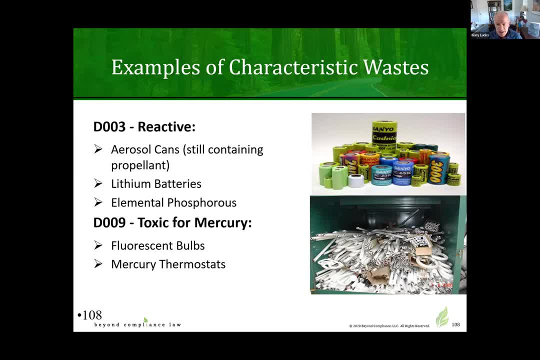 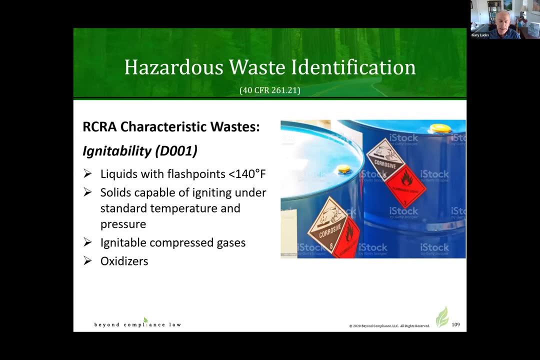 Michael Mann. So we can't dispose of those bulbs in the regular trash because of the mercury and so, or fluorescent tubes, like you see in the picture, and batteries, of all kinds of batteries- are regulated as hazardous waste, even nightcap batteries, Michael Mann. I mean alkaline batteries, that is. 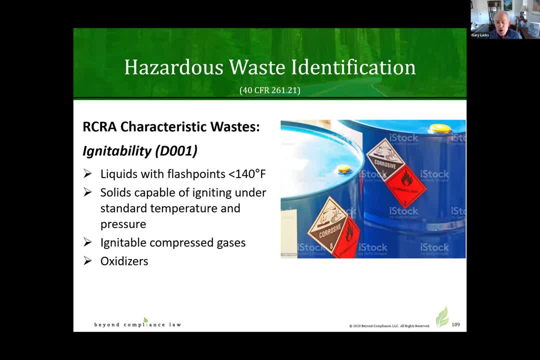 Michael Mann. So deeper definition. or look at ignitability, essentially a low flash point, which gasoline has a low flash point, Michael Mann. So at room temperature gasoline will turn from a liquid to a gas and that's when it becomes dangerous. because, Michael Mann, If there's an ignition source and the gaseous chemical, that's when a fire can start. so low flash points in gasoline, solvents and other chemicals are dangerous for that reason. or oxidizers, as I mentioned earlier. 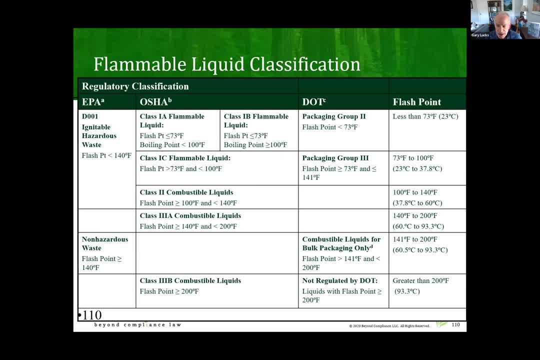 Michael Mann. there's some. we talked about definitions. it gets unfortunately complicated when you look at the definition of a Michael Mann ignitable hazardous waste compared to a flammable liquid, which may not be a waste yet, and the OSHA definitions. 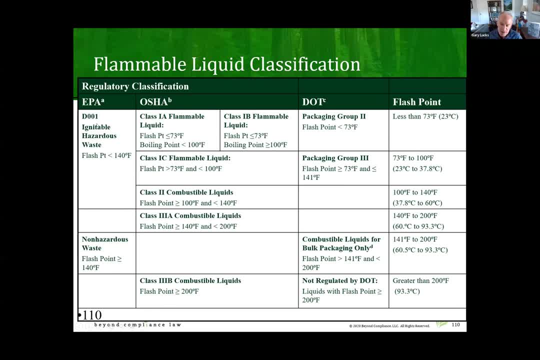 Michael Mann, are different than the hazardous waste definition and the word flammable sounds a lot like ignitable, as does combustible, but they have very precise meanings and an interest of time. that's all I can share with you, but just be aware of the definitional importance. 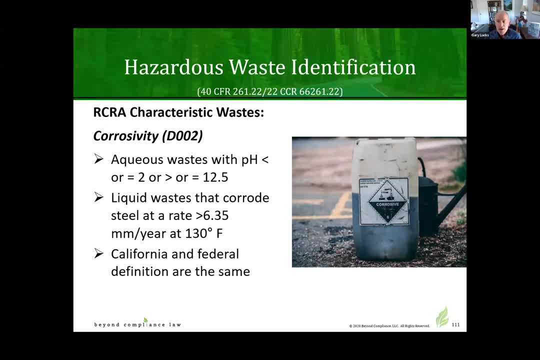 Michael Mann. corrosivity, Michael Mann, there's two kinds of crossivity with a corrosive waste that have water in them, known as aqueous corrosives, and corrosives that don't have h2o but are just the pure chemical that's corrosive. 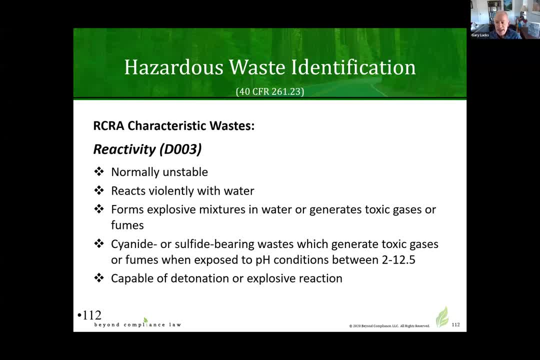 Michael Mann reactivity or chem or chemicals, waste chemicals that are normally unstable. that can that, depending on what they come in contact, whether it's water or some other Michael Mann material like sulfur cyanide, Michael Mann can cause an explosion. military munitions as well. 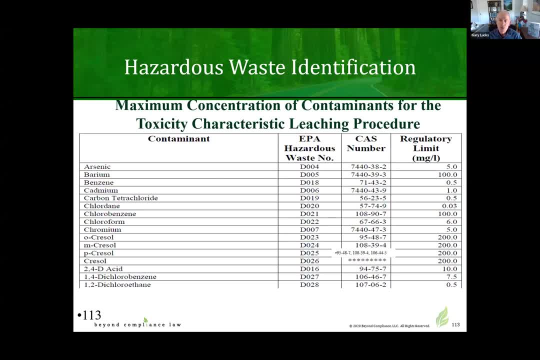 Michael Mann. And then, lastly, toxic Michael Mann wastes are comprised of a list under the federal request, subtitle C, of 43.. Michael Mann metals organics or pesticides. and you see at the top, arsenic is a heavy metal and benzene is a. 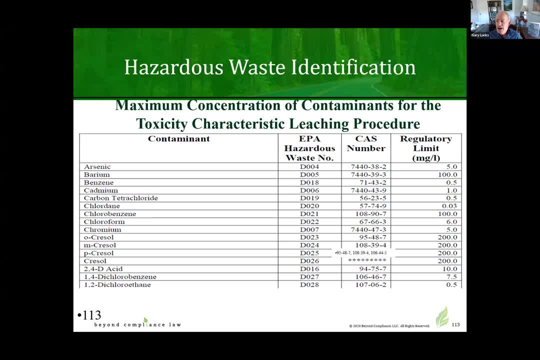 Michael Mann, Organic chemical. cadmium is another heavy metal. Michael Mann, The crease alls are pesticides, and so they're 43 of these chemicals. if you have an extremely low concentration of that chemical, it may be so low that it's not detectable. 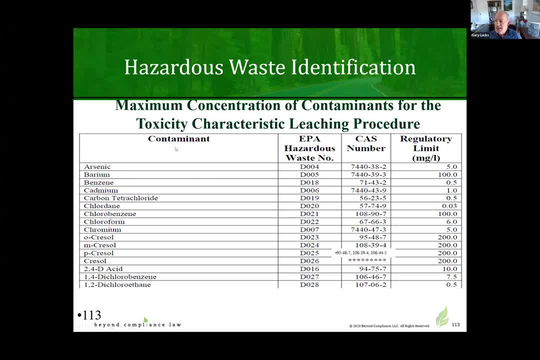 Michael Mann. But if you run a laboratory test known as the toxicity characteristic leaching procedure- the tc LP- that's the acronym, Michael Mann- And you exceed any one of these limits which, as you know, are different depending on the chemical- you exceed that five milligrams for arsenic- then you have a toxic, hazardous waste because you tested it. 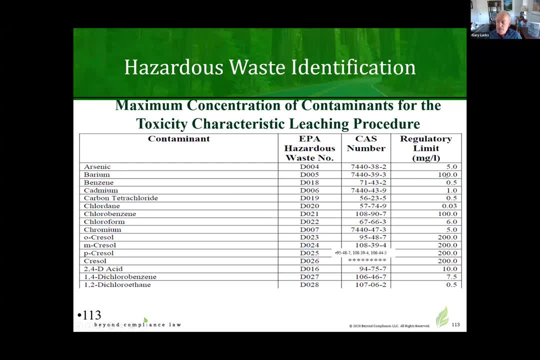 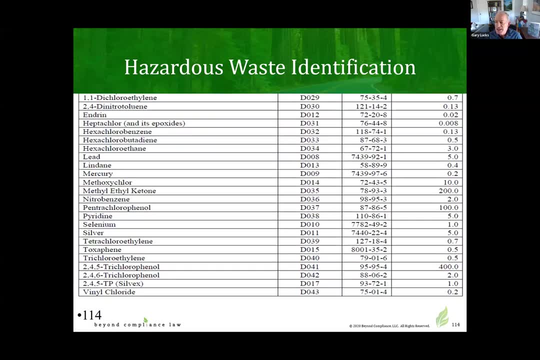 Michael Mann, barium is not as toxic, so you can have a higher amount- you know, 20 fold more before it becomes toxic- and milligrams per liter. so I just lifted these from the regulations and here's more, more of them. the idea is that you start with your sample. 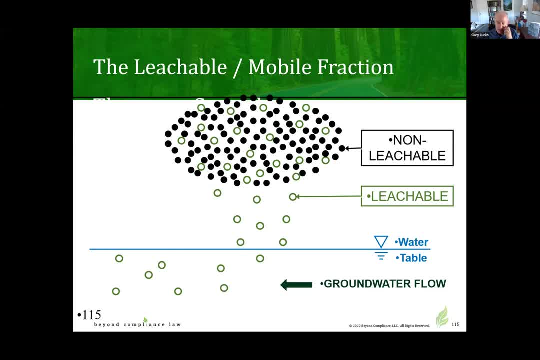 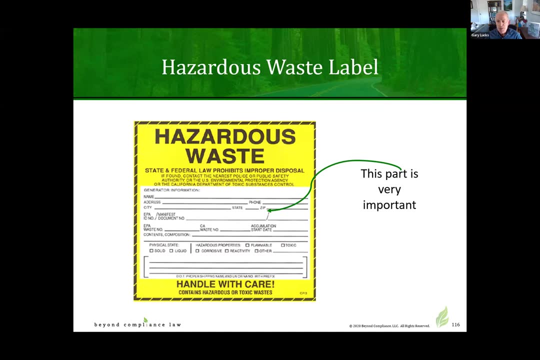 Michael Mann And the parking Michael Mann part that leaches. if you have a certain amount of the dangerous chemical that leaches at high enough level, then it's. it's by definition toxic for purposes of the federal definition of toxicity. Michael Mann, Then we must, once we determine whether we have a characteristic or listed hazardous waste, we have to comply with labeling requirements as well. and you put, among other things: 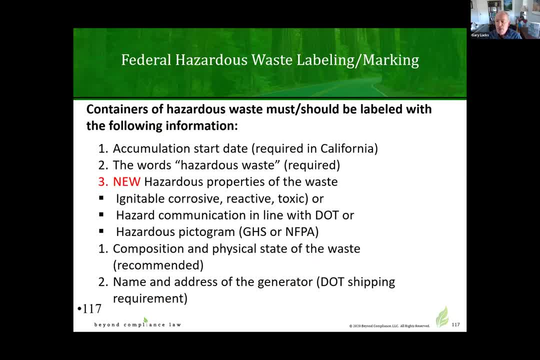 Michael Mann, Because we have to manage the time, Michael Mann. We have to ensure that we don't indefinitely accumulate our hazardous waste, and so California has very hard deadlines by which a hazardous waste must be removed from its source of origin and and shifted to a ultimate. 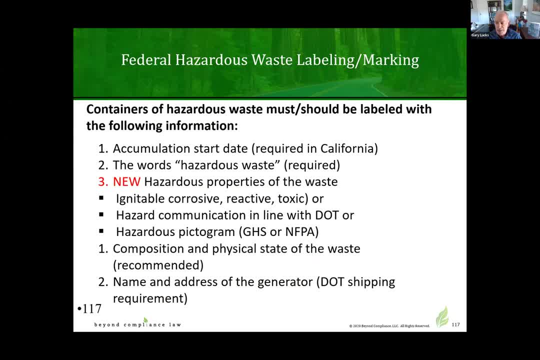 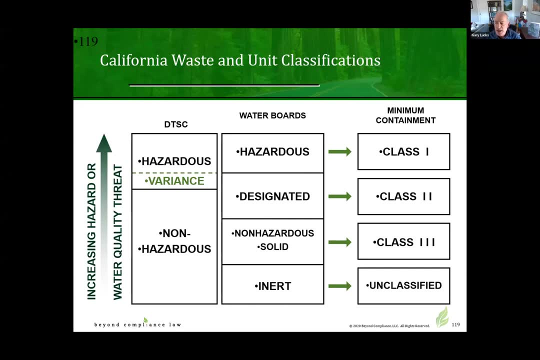 Michael Mann facility that treats, stores or disposes of them. and then the label must have the words hazardous waste and details about its, its Michael Mann properties. Michael Mann, Among other things. Michael Mann- The crossover between hazardous waste and the clean water act and california's law is the destination of a hazardous waste. 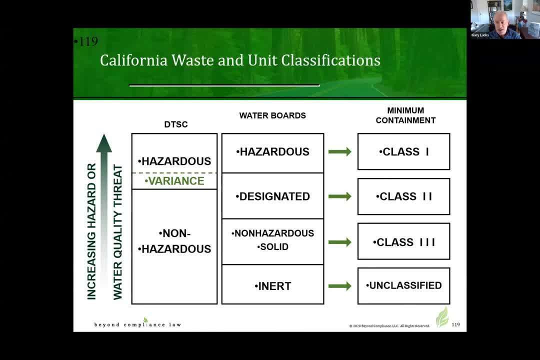 Michael Mann. There are different commercial off site landfills throughout the state that are permitted and license to accept hazardous waste that are generated at individual locations and that's the ultimate end of the line, Michael Mann, Where they're Michael Mann, Either further treated and ultimately disposed of in different types of landfills or surface impoundments, waste piles or other waste management units and a class one hazardous waste facility is regulated under the 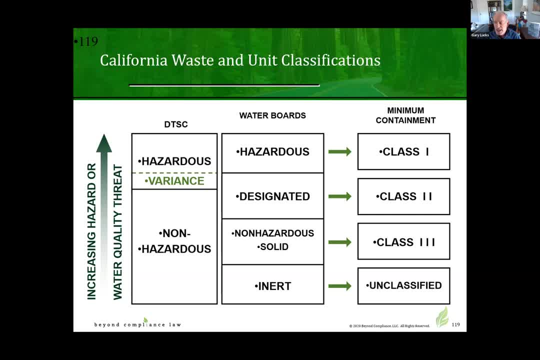 Michael Mann The California porter cologne. water quality control act. that state water quality control act has rigorous requirements for ensuring that any hazardous waste in a class one. Michael Mann water quality control act. Michael Mann water quality control act. Michael Mann water quality control act. 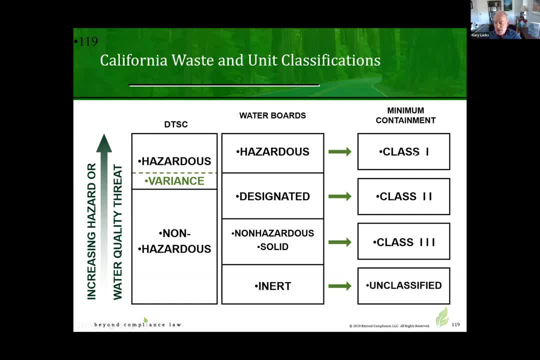 Michael Mann waste management unit will not leak to the environment and there's lots of Michael Mann Engineering and design and implementation requirements that govern these licensed facilities and Michael Mann. Only hazardous waste can go there. they cannot go to the less rigorously managed landfills. the class to landfills are less rigorous and the class three 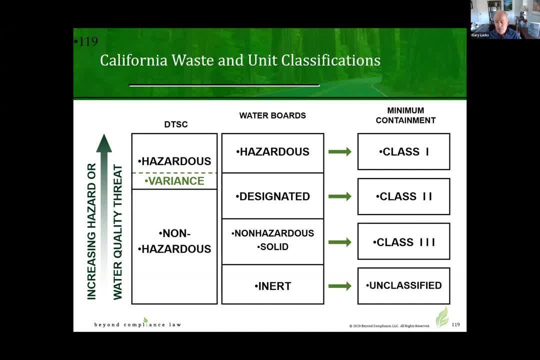 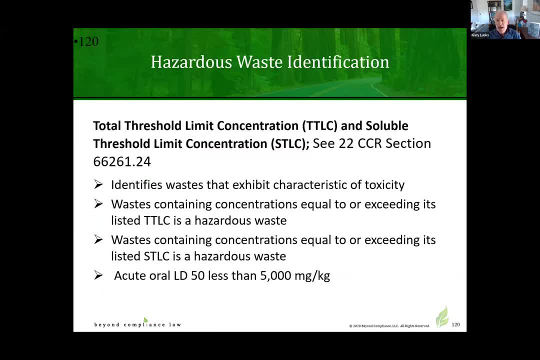 Michael Mann Are where we send our municipal waste from residential and commercial operations. Michael Mann, California has a more rigorous toxicity test than the one I shared with you earlier, and so California regulations. Michael Mann list some of the same toxic chemicals under the federal law. there are 43: metals, organics and pesticides. California has many of the same and has a. 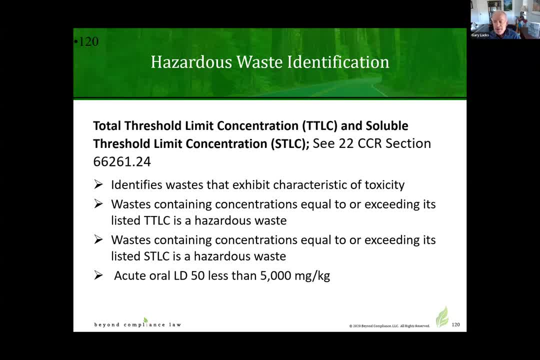 Michael Mann A different test. and why is this more rigorous? because this test is will liberate more of what is is contained in the original sample. because they use a stronger acid, Michael Mann, So you could pass the federal definition and not liberate enough of a toxic chemical to be regulated. you can take that same sample. 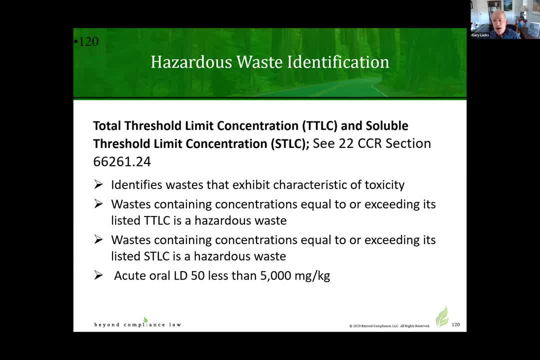 Michael Mann and use the more rigorous California test and liberate more and reach that threshold Michael Mann level as well. so that comes back to the blue dot surrounded by the brown larger dot, where you could pass the federal and not be regulated, but fail the California and be a non rick. rick California hazardous own California, only hazardous waste. 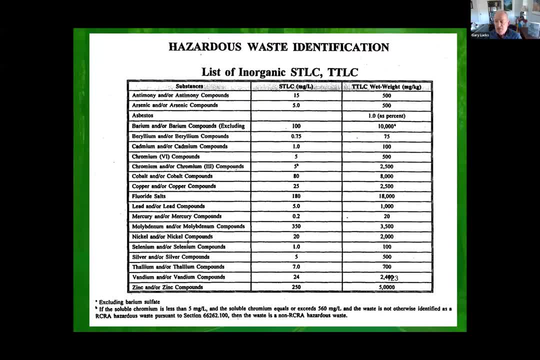 Michael Mann. And so here's a quick glance at the more rigorous California test with some of the same chemicals that are potentially toxic. Michael Mann. And so here's a quick glance at the more rigorous California test with some of the same chemicals that are potentially toxic, with the different 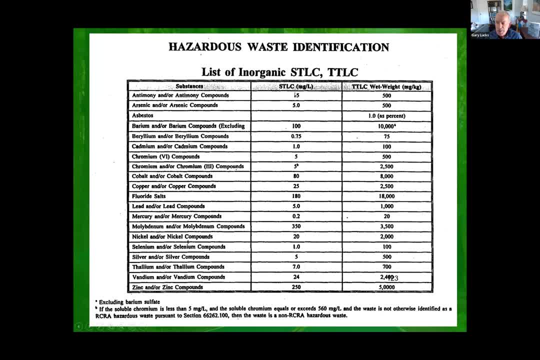 Michael Mann threshold levels by which a waste could be considered hazardous under what's called the s TLC, the soluble threshold limit concentration, which is a more rigorous version of the federal test. there's another test, known as a total threshold leaching concentration, which 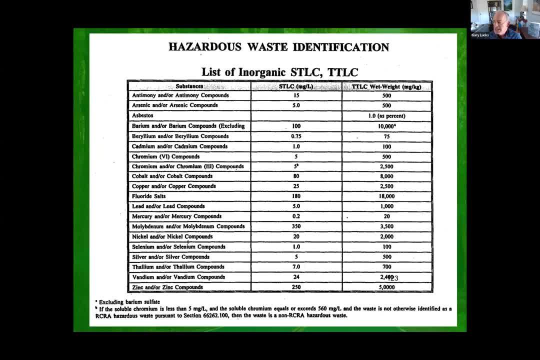 Michael Mann Is kind of a different flavor Michael Mann, And essentially you digest the entire sample and see how much was originally contained there in the first place. you can use one or both test. the T TLC is is a cheaper test but in some ways not necessarily as accurate, and the s TLC is more expensive, and so there's some judgment that goes into which tests you use. 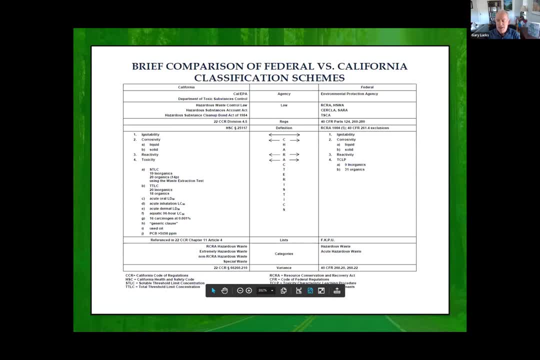 Michael Mann, At the end of the day, if you look at the universe of California requirements and and federal requirements, Michael Mann, You see on the right Michael Mann hand side the ignitable test. we just walked through corrosivity reactivity and the T TLC, the toxicity characteristic leaching procedure. 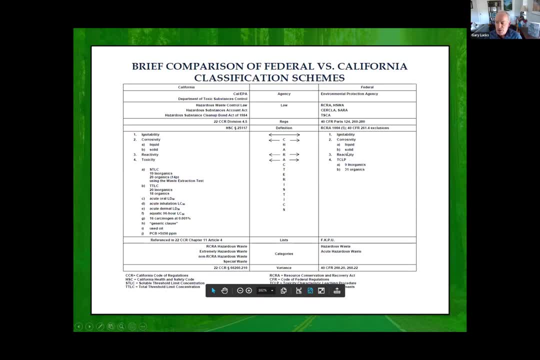 Michael Mann, that's how you determine a hazardous waste under federal law, under California law. you see, there are many more tests that that raise the possibility of failing. where you might pass with fewer tests and limits under the federal law, Michael Mann, You might fail under the state law. 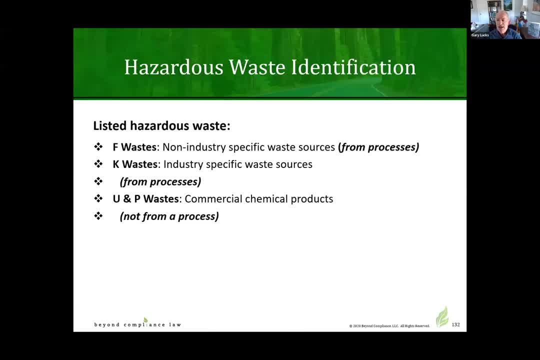 Michael Mann. And so we saw, in the blue dot to the right, Michael Mann. We have Michael Mann, Four categories of lists and the regulations, the F waste, go on for several pages and same with K ways, you and P ways and, as you remember, the first to represent waste that are generated from processes. 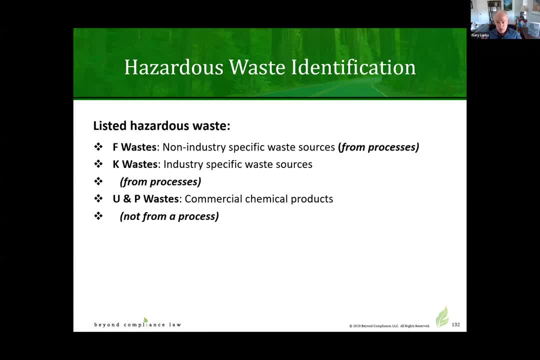 Michael Mann. The waste is. the material does not become a waste unless you work with it and process it and degraded or shift its chemical Michael Mann outcome due to a process Michael Mann And we saw that the K wastes are those that are generated by certain industries. so there's a couple of pages that speak to industry or oil and gas waste. 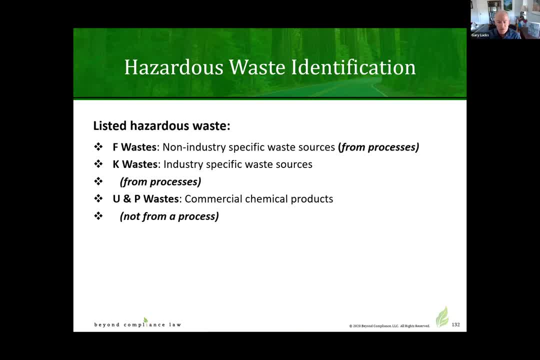 Michael Mann, If you're not in the oil and gas industry, you don't care about K waste unless you fall in one of the other Michael Mann industry specific categories and regardless you can generate waste through processing, irrespective of whether you are in a particular industry type, for example, solvent waste. 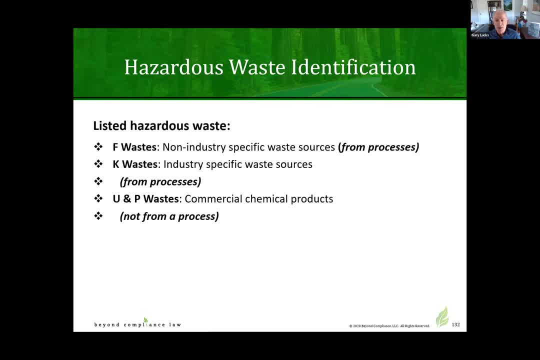 Michael Mann will be generated from the process of using the solvent for decreasing, and you can decrease using a solvent, whether it's in a Michael Mann factory or Michael Mann auto shop or any other type of facility. that is not one of the industry type, so it's generic and again. so the first to deal with processing. 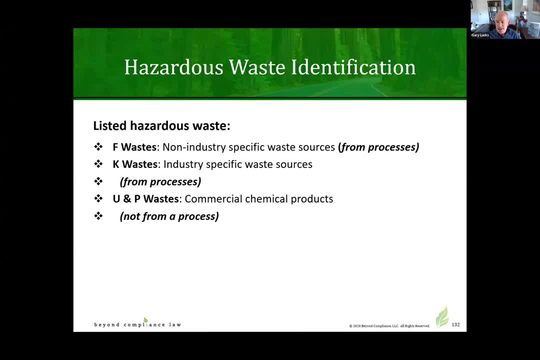 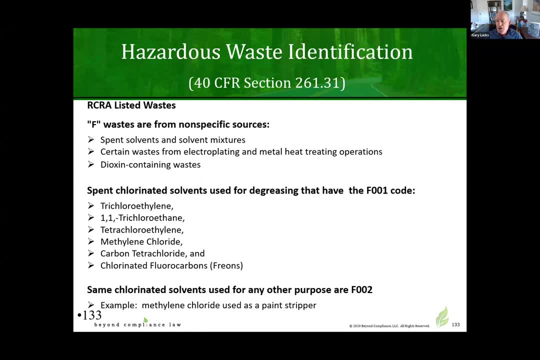 Michael Mann, The second to, are generated not through processing but through spills. container residues are off spec products and, Michael Mann, In your materials that you'll be getting copies of, you can take a deeper look at examples, but i'm not going to go into them for. 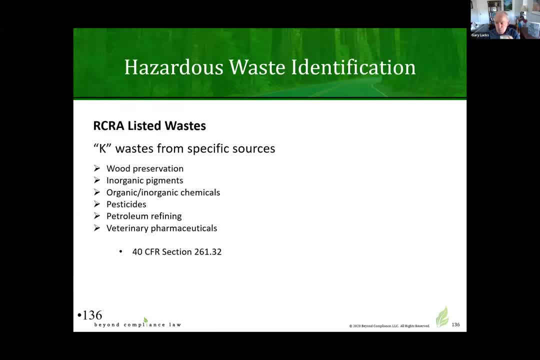 Michael Mann. Our limited time here. Carrie, we have a like a 30 minute time. check, Michael Mann. What Carrie Campbell About 30 minutes to go, Michael Mann gotcha. Thank you, I thought you made a 30 minute question. 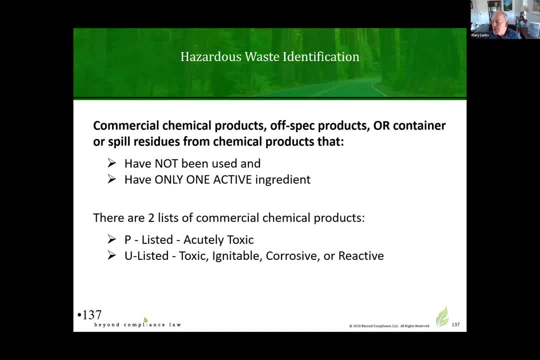 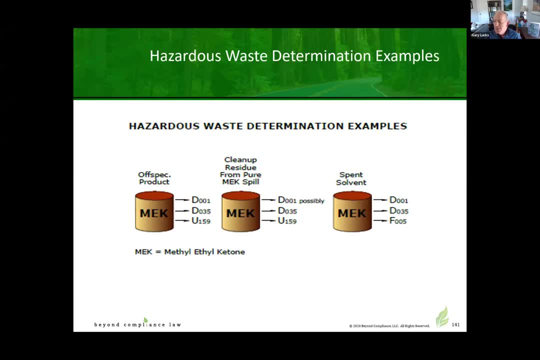 Michael Mann. Okay, yeah, so the next couple slides illustrate what I shared with you, so I think, in the interest of time, you have the material here and I will move past it. Michael Mann. This slide Michael Mann illustrates: 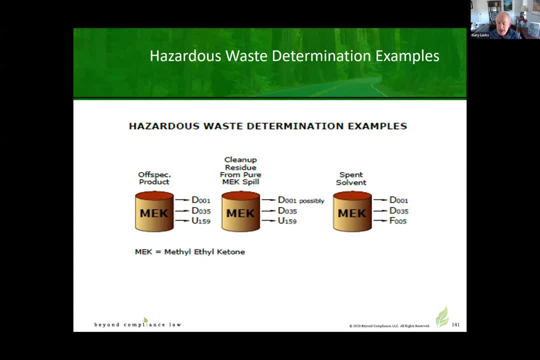 Michael Mann, The point where the the drum contains me K and that stands for methyl ethyl ketone, which is a very dangerous solvent. Michael Mann, And depending on the circumstance, you could label or characterize that waste with one or more of the characteristics or listings that I just shared with you, and each characteristic and listening has its own nomenclature with D you. 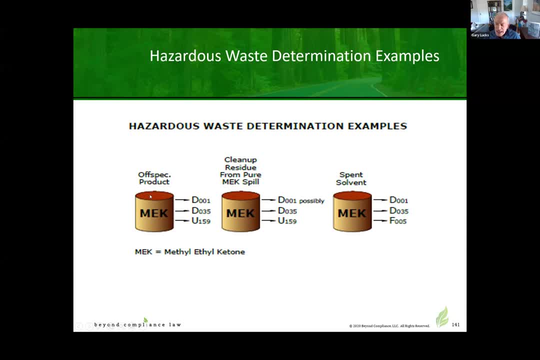 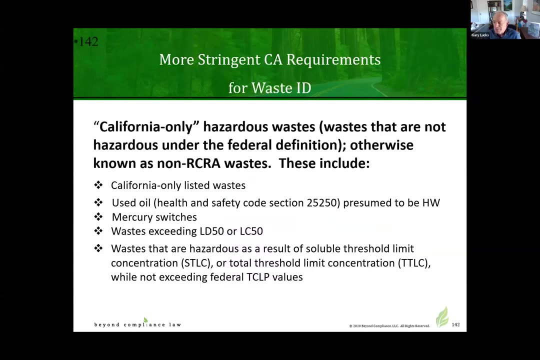 Michael Mann, F or K, and so, without going into that, the point here is that, depending on whether you have a spent solvent, a cleanup residue or aspect product, that same drum might be managed or profiled or labeled differently. Michael Mann, One thing to point out here: so not only does California have a more stringent toxicity test, 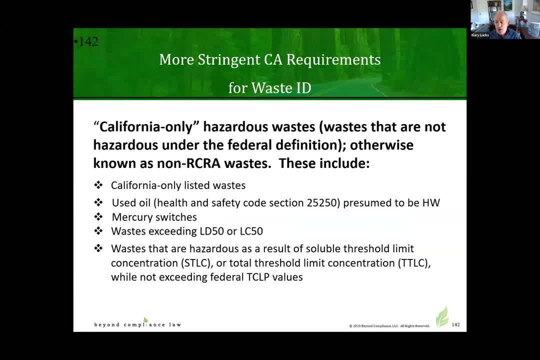 Michael Mann, But it also regulates Michael Mann Used oil more rigorously than under the federal law. under California law there's a rebuttable presumption that all used oil is Michael Mann hazardous waste, and we'll see that we must manage used oil as hazardous waste. 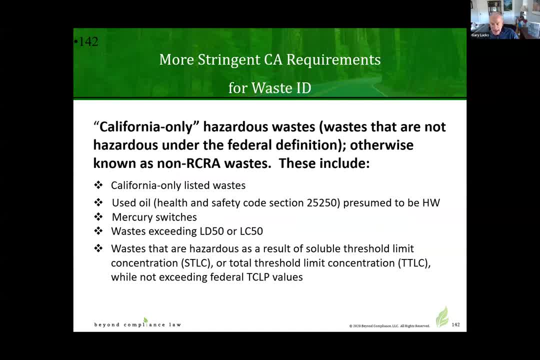 Michael Mann, As if it was any other hazardous waste. Michael Mann, At the point of generation, at the location in which it was generated. but when we ship it off site, Michael Mann, We don't have to follow as rigorous standards for manifesting it and department of transportation requirements. so rigorous on site, less rigorous off site. 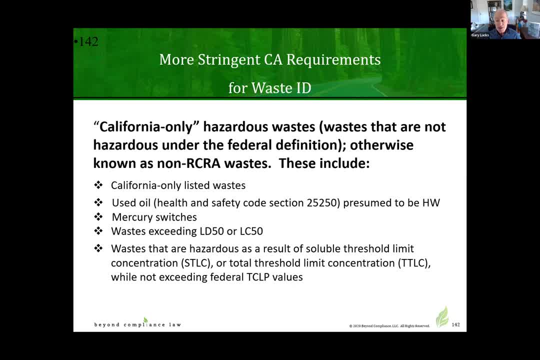 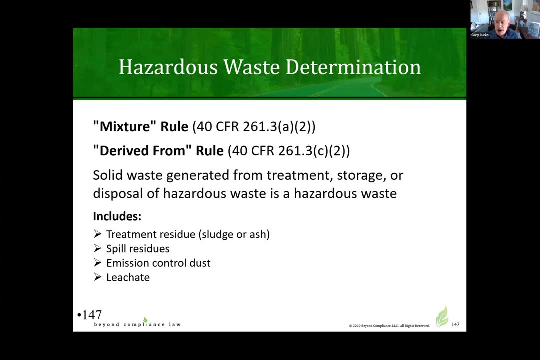 Michael Mann, There are other statutory definitions of listed waste under California law as well, including mercury switches and others. so that just gives you a flavor for how California is a bit tricky. Michael Mann, We talked about the mixture role in the drive from role. so the drive from role, as I said, you have a more highly concentrated 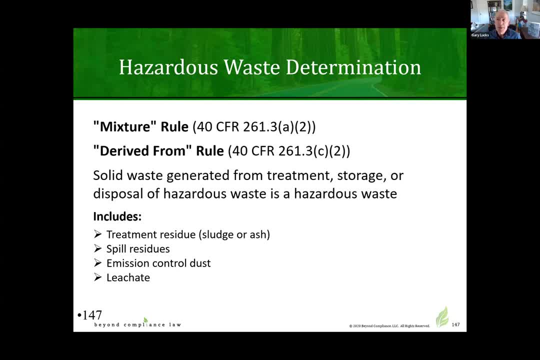 Michael Mann. outcome: due to the scrubbing or or filtering or other incineration or whatever you use to treat what you end up with as a more highly concentrated ash or filtrate Michael Mann At the end of the process and it by definition. 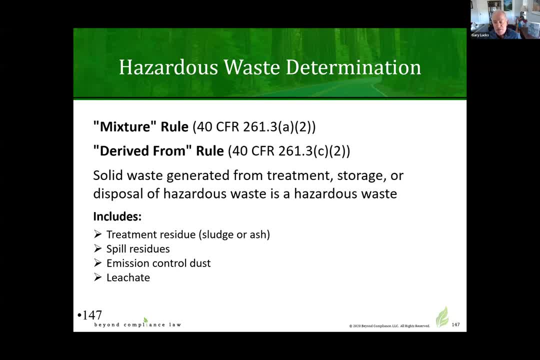 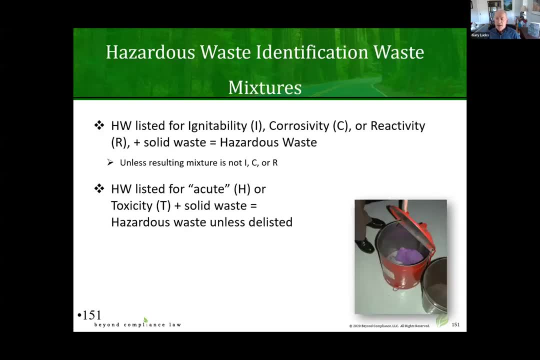 Michael Mann, The treatment residue, the derived that's derived from, must be automatically managed as a hazardous waste, no exception. and then mixed your role back to the swimming pool scenario we had. we started with a 55 gallon drum of a solvent Michael Mann And you've got like an Olympic swimming pool. 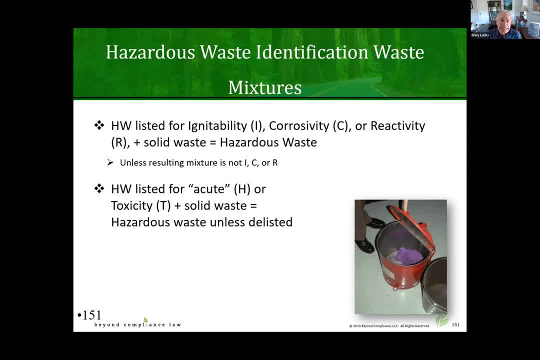 Michael Mann. The question would be is is: is the constant, is the, the concentration in the Michael Mann In the water safe enough to swim in? not if it's a 55 gallon drum, but what if it was just a drop of the solvent? 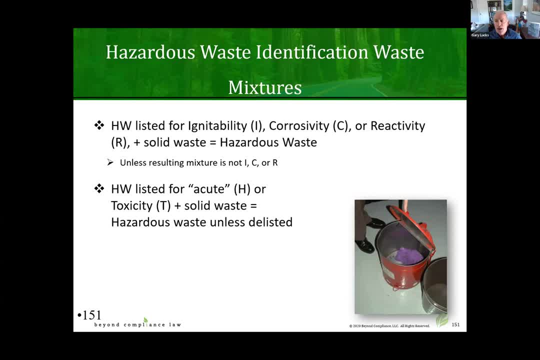 Michael Mann And it. it all comes down to sampling the water. to see if the character, if you would fail the characteristic of ignite ability with that one drop, would you fail the definition of reactivity. or if that one drop was an acid, with that one drop, 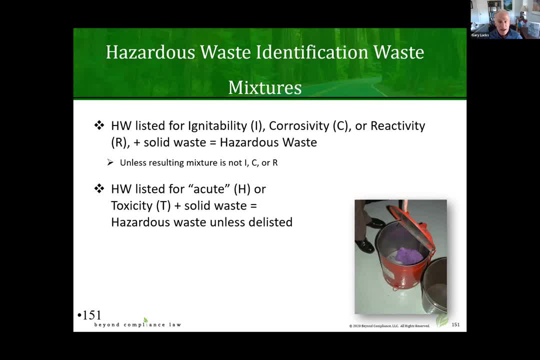 Michael Mann, fail for corrosive it? more than likely not, but you know, at some point between one drop and 55 gallons you're going to, the sample will exceed the characteristic test for ignite ability, corrosive it and reactivity. and notice, I did not talk about toxicity. so 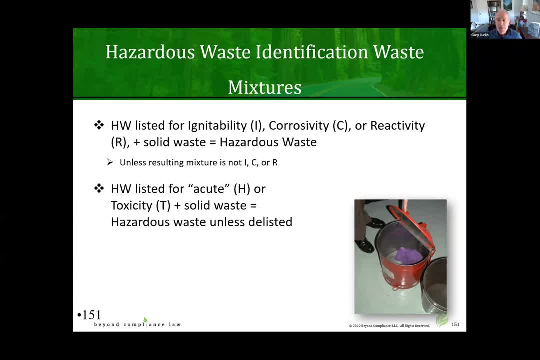 Michael Mann. The rule is a little different. it says: if you drop, if you spill or co mingle a toxic waste with a non toxic- Michael Mann benign material. Michael Mann, Regardless of the concentration for toxicity it is by definition and always will be toxic. so ignitable, reactive, corrosive commingled waste can be exempt if the concentration is such that you will pass the test for that characteristic. but the toxicity test will not. regardless, even if it's a tiny drop, it's automatically hazardous waste. 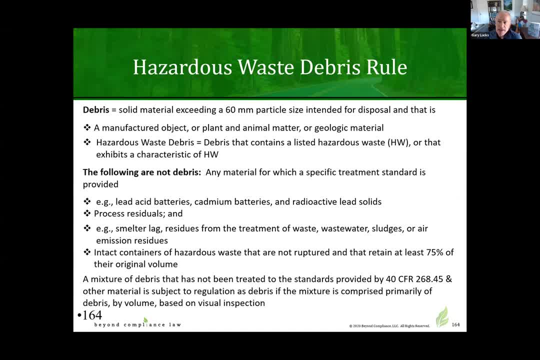 Michael Mann. If you've got building materials that can be, Michael Mann, contain hazardous waste like lead lead materials, for example. if it's over 60 millimeters that debris, which is roughly about two and a half inches, then the debris itself is. 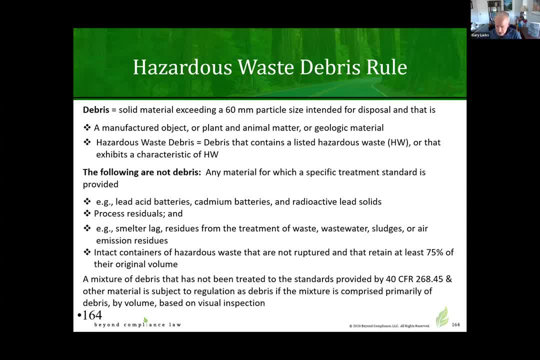 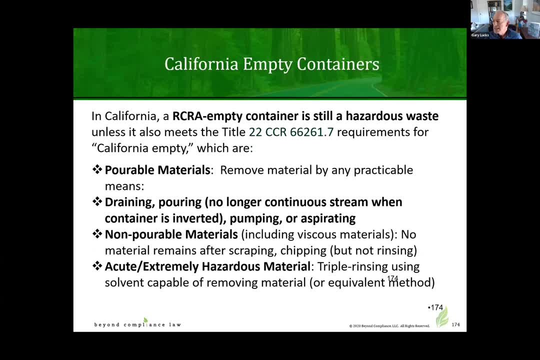 Michael Mann mixed with the hazardous constituents. so the debris itself must be managed as a hazardous waste, Michael Mann. Now let's imagine, Michael Mann, You have a 55 gallon drum, Michael Mann, That contain Michael Mann, The hazardous waste, and you empty that container. 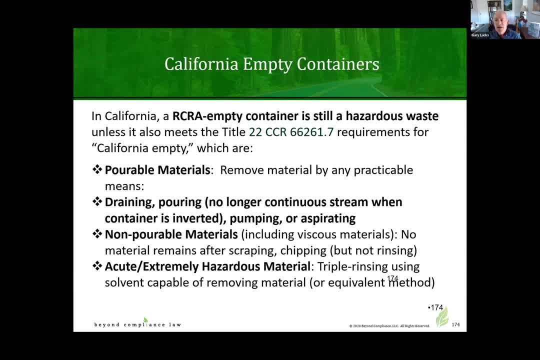 Michael Mann. The question is: is that container empty enough to be considered non hazardous? and could you just, Michael Mann, manage that empty container in a landfill like a class three landfill? that's not as rigorous as a hazardous waste class one landfill. Michael Mann, It all depends on how much residue is left in the container. if it's a, it's like a completely. 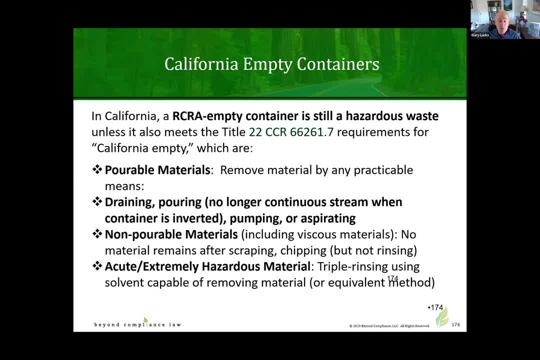 Michael Mann devoid of the hazardous material or waste that was in it before then. the empty drum is truly empty, but there's a definition legally of what is empty and empty. Michael Mann Is is driven by effort to cleanse the drum from what was in there. so you have to pour out what was in there, you have to drain. 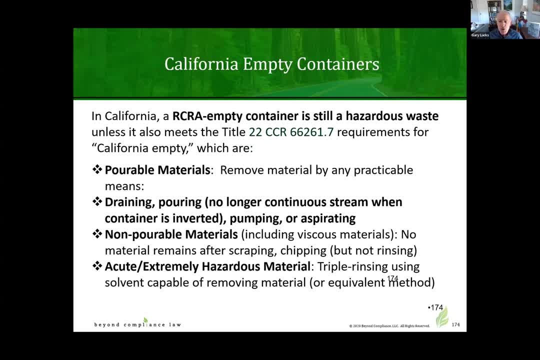 Michael Mann. And and you do what you can to scrape or chip what was in there, Michael Mann, And then if, in doing so, there's still enough residual that exceeds one inch or more, Michael Mann, Then it is not empty. but if it, if you pour, scrape or chip what was in there and you get as much of it out as you can and you have less than one inch, it's empty and an empty container legally under rick ra. 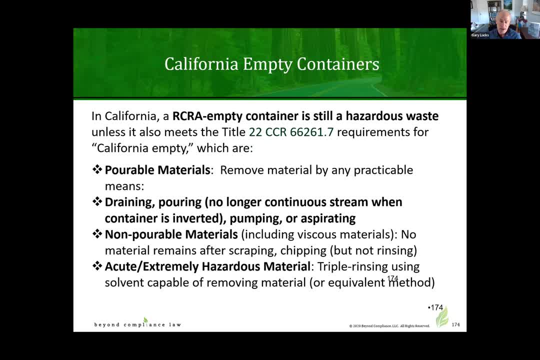 Michael Mann can be managed, Michael Mann Alternatively, and Michael Mann Not as a hazardous waste. but we under the super fund law it may not be advisable to enjoy the the rick ra empty container exemption because under the super fund law that that residual 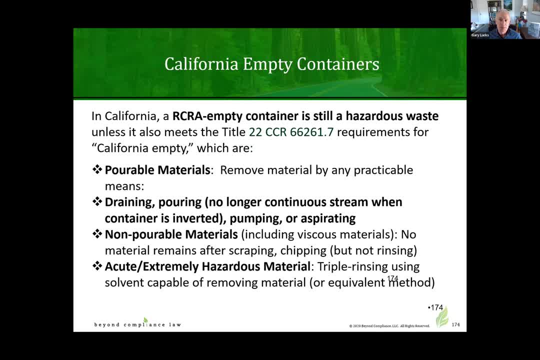 Michael Mann could expose the generator to potentially responsible party liability under the super fund if that landfill ends up being compromised. Michael Mann, And then, and if the if the clients name is on there, then they could be a deep pocket liability exposed to liability as well. 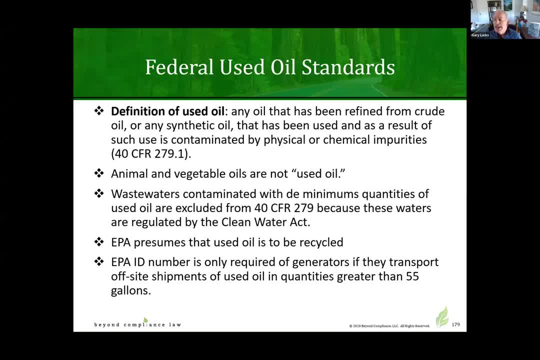 Michael Mann. So I mentioned used oil. under the federal law, used oil can be- does not have to be- managed as a hazardous waste. Michael Mann and Michael Mann, If you generate more than 55 gallons of used oil under federal law, you need to. 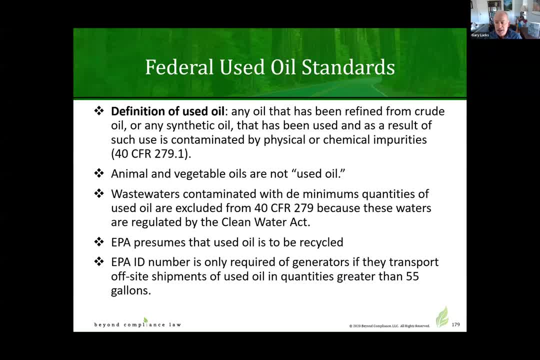 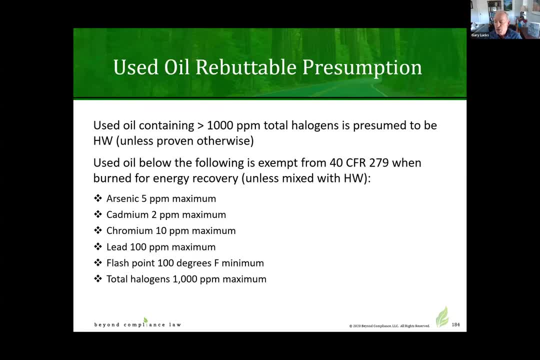 Michael Mann, Contact EPA and receive a identification number, as known as an EPA identification number, for transporting 55 gallons or more of used oil. Michael Mann, and used oil under federal law is presumed to not be hazardous. but let's say you have hazardous, you have used oil under the federal law outside of California, but that used oil was contaminated with heavy metals, as you see here, from arsenic to lead. well then, you don't enjoy. 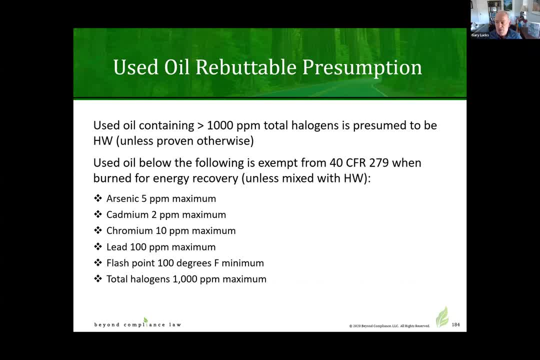 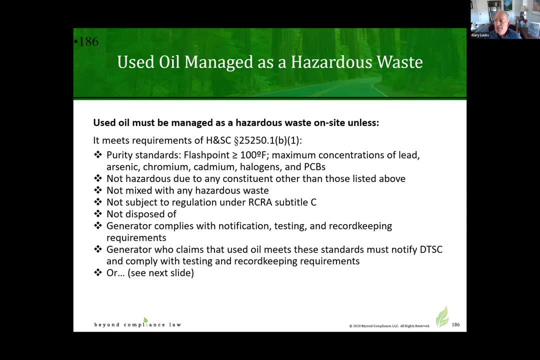 Michael Mann The exemption or the special treatment under 40 CFR section 279, because the driver is these heavy metals, not the fact that it's used oil. Michael Mann, Under California law- Michael Mann, I said earlier, it is presumed to be a. 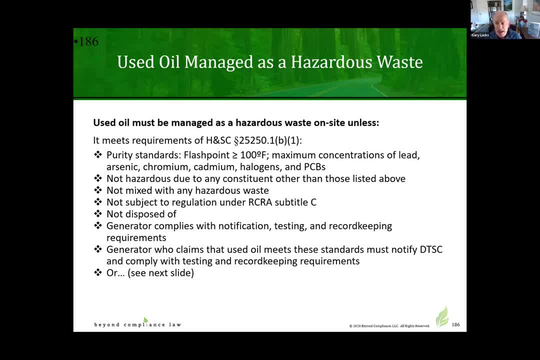 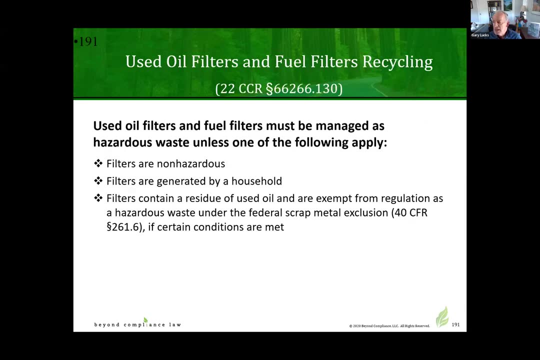 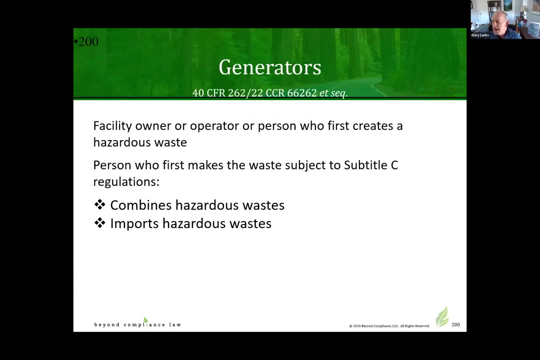 Michael Mann hazardous waste and must be managed on site like any other hazardous waste, but can be managed more lightly off site by Michael Mann By using a bill of lading instead of a more involved hazardous waste manifest. Michael Mann. i'm going to move past there some of the same kinds of labeling under California law, so i'll leave it at that. 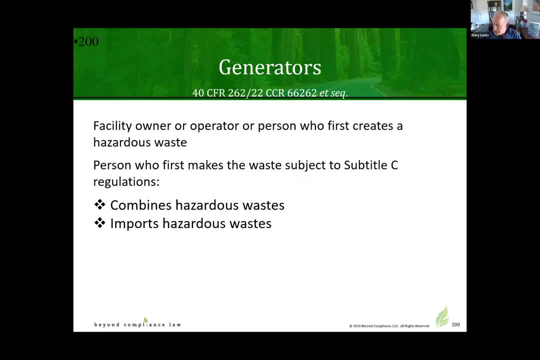 Michael Mann. And now we need to know that there are different types of generators. if you're a generator of hazardous waste and you generate very little, Michael Mann, You have lighter requirements than the heavy duty Michael Mann. And then there's the industrial facility that generates a lot, and so any facility that 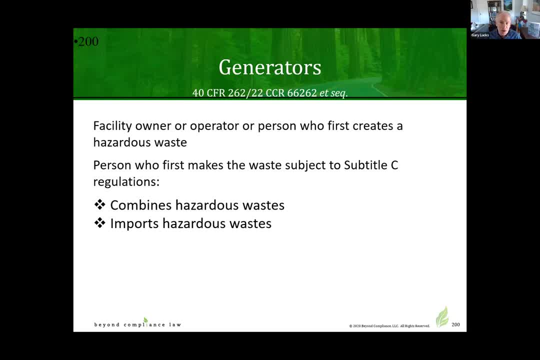 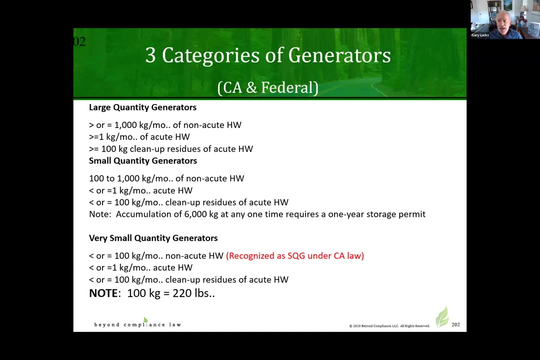 Michael Mann, Due to their action or inaction, causes a material to become a hazardous waste, is by definition a hazardous waste generator, or if you import hazardous waste, you also are become a generator. but, as I mentioned, there are different Michael Mann types of generators because large quantity generators have many more rigorous requirements than small quantity generators. 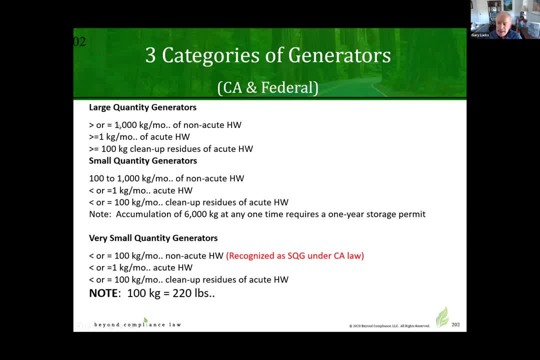 Michael Mann And a large quantity generator essentially is one that generates 1000 kilograms of hazardous waste per month. 1000 kilograms is another Michael Mann way. we mean it's a, it's a ton. so, Michael Mann, 1000 kilograms or 2200 pounds is a ton, and any facility that generates more than a ton a month must be managed as a large quantity generator. 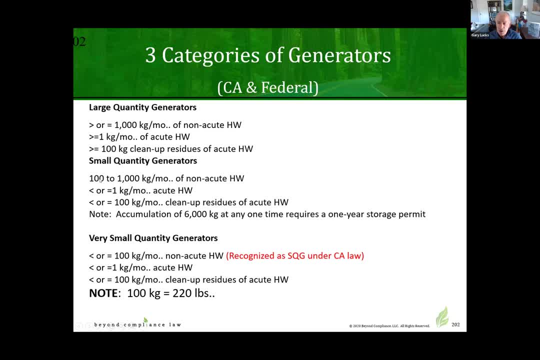 Michael Mann. Any facility that generates less than 1000 kilograms but more than 100 kilograms is a small quantity generator with fewer requirements, and under the federal law, a Michael Mann facility that generates less than 100 kilograms per month or less than 220 pounds is exempt. 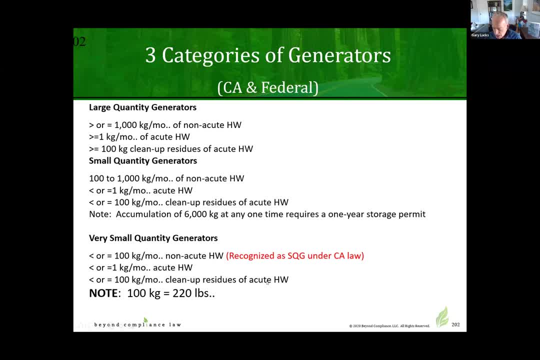 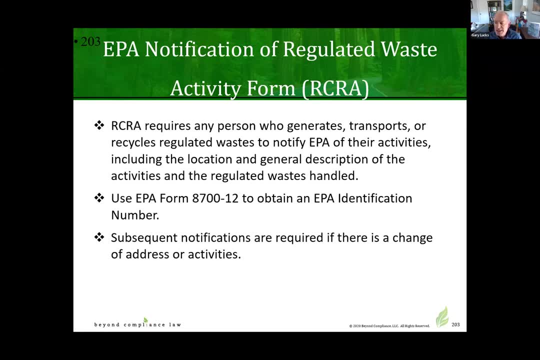 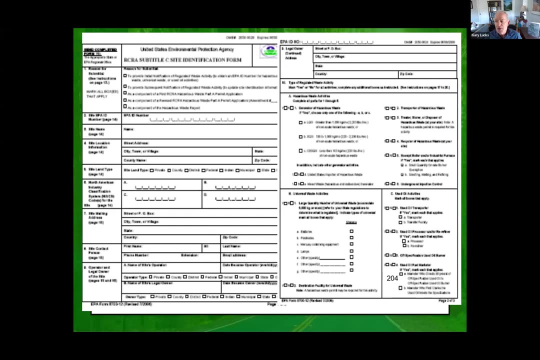 Michael Mann and considered a very small quantity generator. Michael Mann. Under under recently promulgated rules, Michael Mann, Any non exempt generator must also go to EPA. fill out a form to get an EPA identification number that corresponds with the physical address. 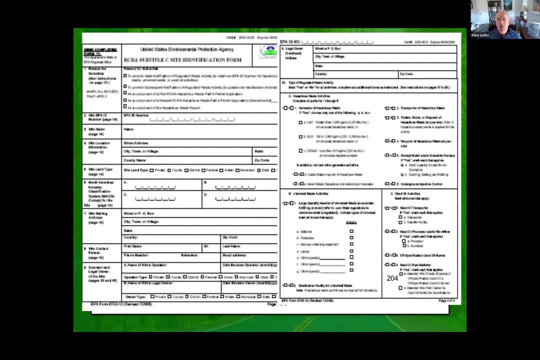 Michael Mann. So imagine acme manufacturing company at 100 main street. they generate wastes that are hazardous waste, Michael Mann. They get EPA number one, Michael Mann. Acme sells their business, Michael Mann, 10 years later to another company that doesn't generate hazardous waste or generates a different kind of ways. they get that same EPA, didn't he number? the ID number corresponds with the address. 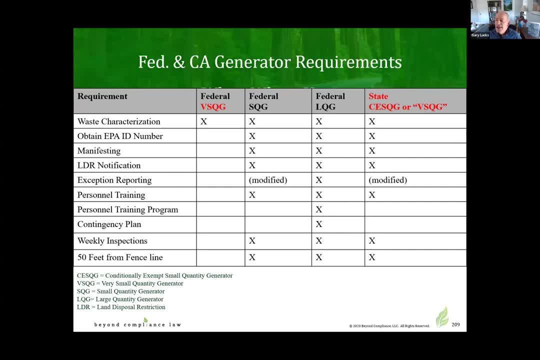 Michael Mann. And once you're a generator of hazardous waste, then what must you do? and we've talked a little bit about some of that, so let's begin with the federal Michael Mann Large quantity generator. the lq G is a generator that generates 1000 kilograms, or one time per month. they must do what we've already discussed: they must profile their ways to determine whether they're in or out. they must get an EPA identification number. 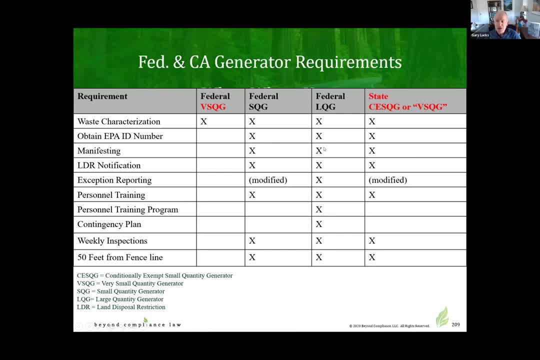 Michael Mann. They must ship their hazardous wastes using a special document known as a hazardous waste manifest. that care that identifies the amounts and types of waste, Michael Mann, And it's designed to ensure that the waste end up to a, a licensed facility for treating, treatment, storage and disposal, within 45 days. 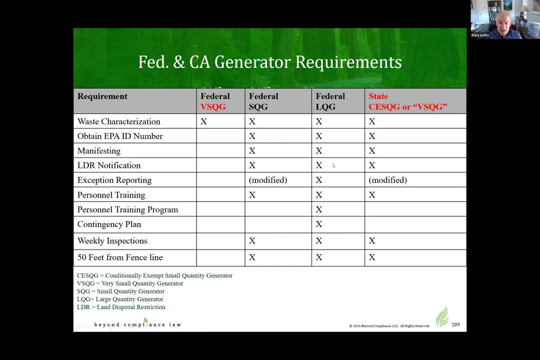 Michael Mann. And if 45 days go by and there's no evidence that the shipment arrived in that timeframe, then there is something known as an exception report, where you have to affirmatively chase down that load and do some paperwork, Michael Mann. there's also something known as an LDR, a land disposal. 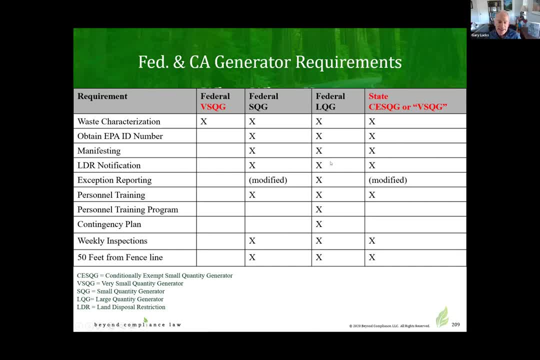 Michael Mann Restriction. a land disposal restriction is Michael Mann Information the hazardous waste generator must provide on the underlying characteristics of the waste they're shipping off site, Michael Mann, Because the generator knows the recipe or cocktail of the waste that they've generated and there it's important to know what's there. so the downstream facility that treats the waste 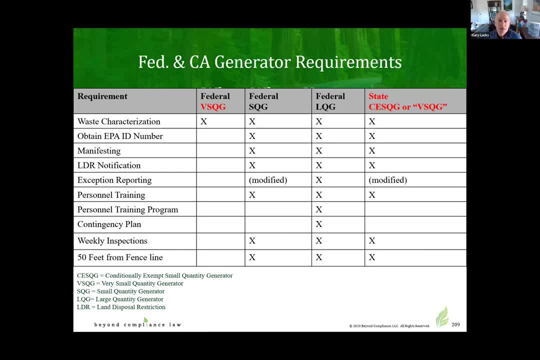 Michael Mann, will be safe. they, Michael Mann, they'll know what's like. for example, some ways cannot be treated with water. the cause: an explosion. so, Michael Mann, it's notable that the land disposal restriction provides valuable information for the downstream facility and the LDR stands for land disposal. 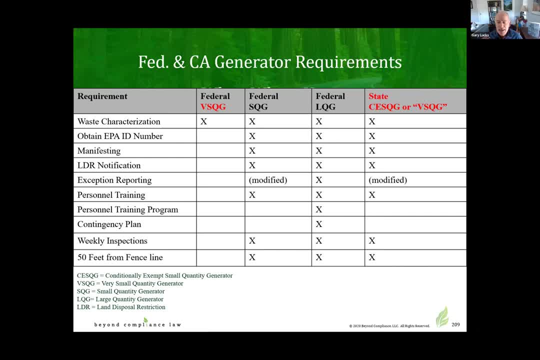 Michael Mann So, and a restriction. so the idea is the the the license facility downstream. will not, Michael Mann, dispose of the hazardous waste in the land based unit? it's restricted from doing so, Michael Mann, Unless they know what the underlying constituents are so they can safely manage it. personnel training, as I mentioned earlier. it's a legal requirement that 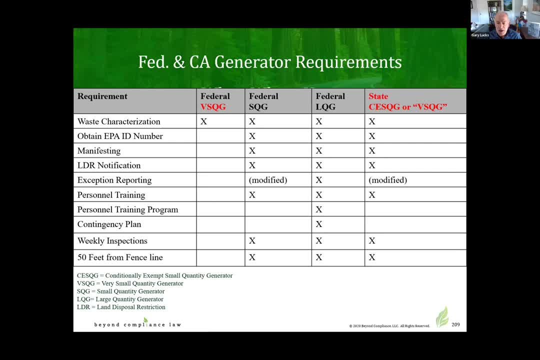 Michael Mann, Personnel and contractors especially people forget contractors, but contractors and personnel. Michael Mann Of the generator, Michael Mann, must be officially trained annually and i'll share some details on that later. the large quantity generators must develop a written training plan with bells and whistles in it. they must 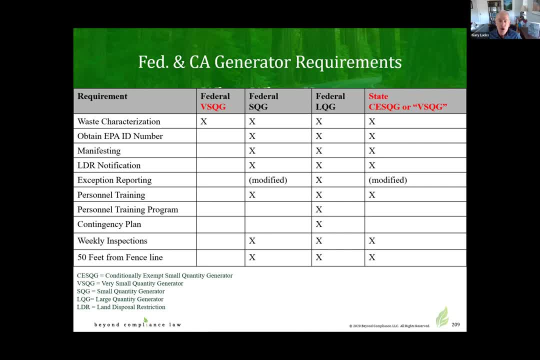 Michael Mann Draft a document for their long term accumulation facilities that store or accumulate hazardous waste. Michael Mann, To address the possibility of an earthquake, a fire and explosion, a terrorist act. Michael Mann, What do you do? how do you, how do you manage to prevent that from happening? you've got a draft, the contingency plan- and share it with the fire department, the police department and the hospital. 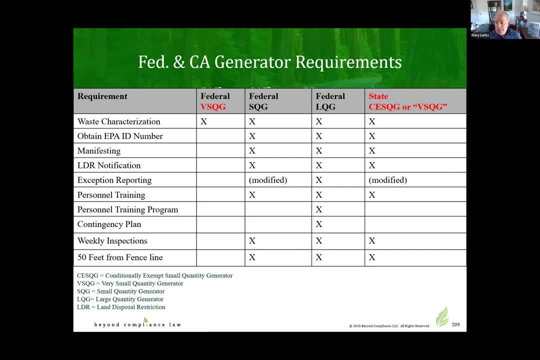 Michael Mann, The long term accumulation facilities must be inspected weekly and they cannot be located too close to the fence line. if there's a, Michael Mann, ignitable or reactive waste, Michael Mann, Oh. and so now, Michael Mann, Notice how the federal requirements are the same for the small quantity generator, except the personnel training is lighter. 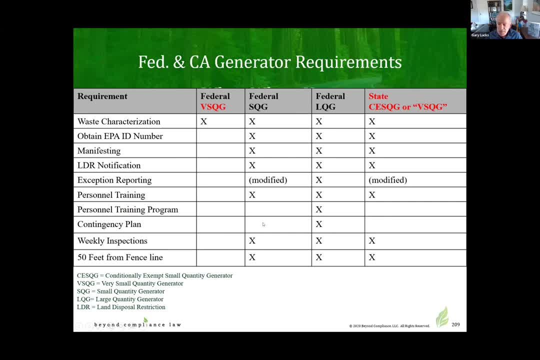 Michael Mann. The exception reporting is lighter and the contingency plan is not required. so more requirements for a large and less requirements for a small quantity generator Michael Mann. Under California law, California does not recognize the small quantity or the very small quantity Michael Mann generator, and so what would otherwise be exempt under federal law is treated or managed just as if it was a small quantity generator. so the state equivalent of a small quantity generator must be managed as 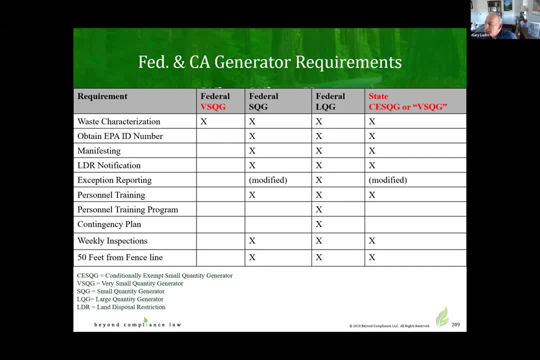 Michael Mann As if it was a Michael Mann. You know, this is a little typo, i'm really. this should be a small quantity generator. Michael Mann must be managed as Michael Mann. If it was, no, no, no, i'm right, i'm right. I conditionally is that, yeah, it would otherwise be exempt under federal law- must be managed as if it's a small quantity generator. so that is correct. 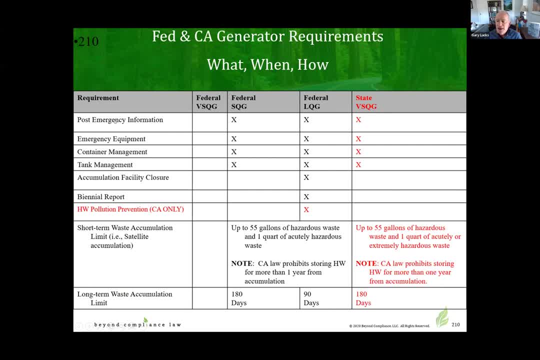 Michael Mann federal. other requirements under large quantity generator there's all kinds of emergency equipment that must be maintained and inspected at the areas where you accumulate large amounts of waste before they're shipped off site. the containers must be a certain design and Michael Mann condition and labeling, as well as tanks. 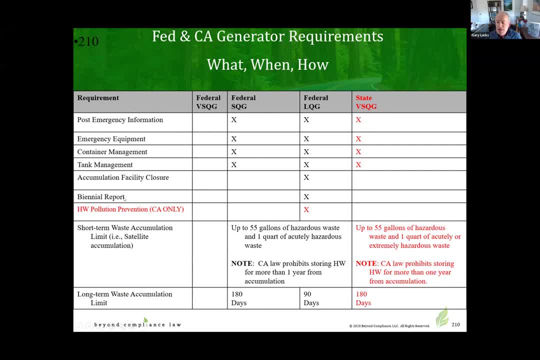 Michael Mann, If you close one of these facilities as a whole closure process, there's every other year reporting to DTSC. California has a specific law known as SP 14 that's designed to ensure ways to reduce the amount or bar hazards of a chemical of. 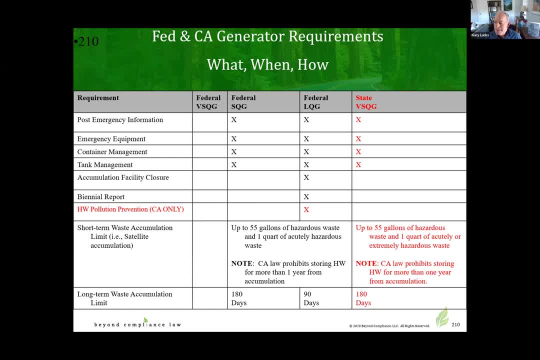 Michael Mann Large quantity generators. and so they are, Michael Mann. They have to develop a very involved plan for pollution prevention. and then you can't accumulate, Michael Mann, More than 55 gallons of a hazardous waste at or near where it's generated. it must move to the long term accumulation area within three days of reading, reaching 55 gallons. and once it reaches the long term accumulation area, you can accumulate for more than 90 days. 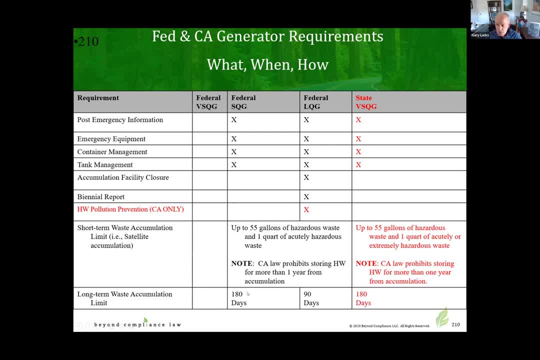 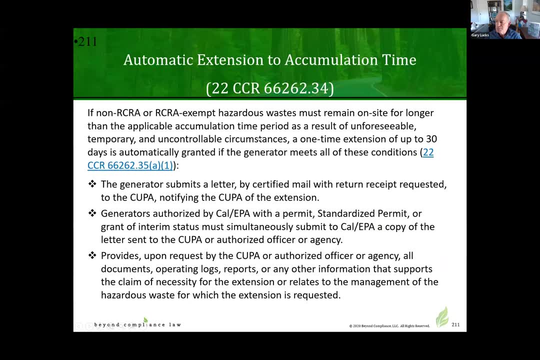 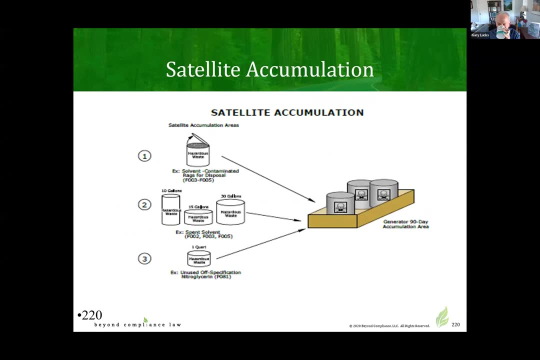 Michael Mann For large quantity generators and 180 days for small quantity generators. and again, more bells and whistles in the large quantity compared to the small quantity column. Michael Mann, i'm just making a judgment call here. so, Michael Mann, You can only accumulate 55 gallons of a hazardous waste at or near the process where it's generated. 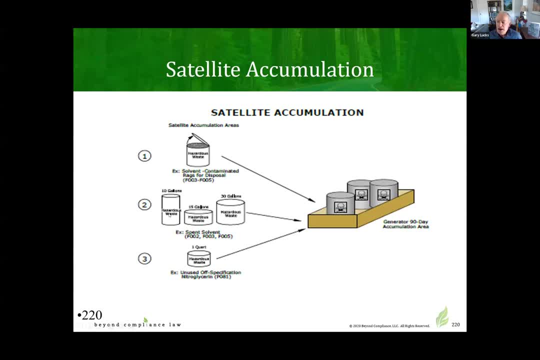 Michael Mann. So 55 gallons. but notice, here you've got- it's probably a little hard to see, but you've got- 10 gallons of one way stream, 15 of another and third, that's 55 gallons all together. Michael Mann, The law, the rule says no more than 55 gallons of a particular way stream, but you've got three different flavors here so you can actually accumulate 55 gallons of each of them. so that'd be 165 gallons because of three different flavors there. 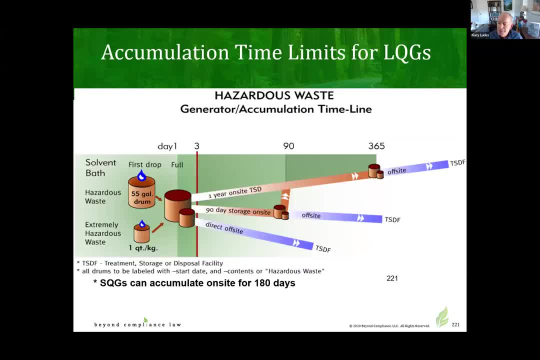 Michael Mann. So just that's illustrating the satellite accumulation there, Michael Mann. Ultimately, the way it works under federal law is different than under California law. under federal law, Michael Mann, You can indefinitely accumulate hazardous waste, Michael Mann, At a facility, as long as you've never accumulate more than 55 gallons. 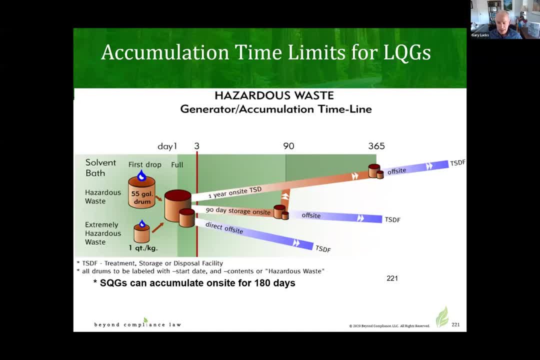 Michael Mann. So, for example, Michael Mann, If you're Michael Mann In name a state outside of California, let's say Nevada, Michael Mann And you're you're the the the Tesla battery Omega facility. they're generating waste and 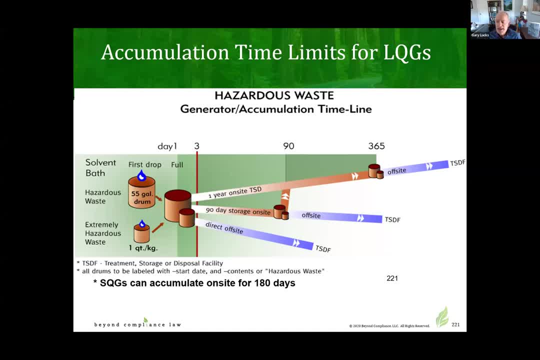 Michael Mann, In this one particular business unit they generate, let's say, they generate a gallon a month. so in one year they've generated 12 gallons, in two years 24 gallons, and so on. Michael Mann, they've not reached 55 gallons, so they can accumulate. 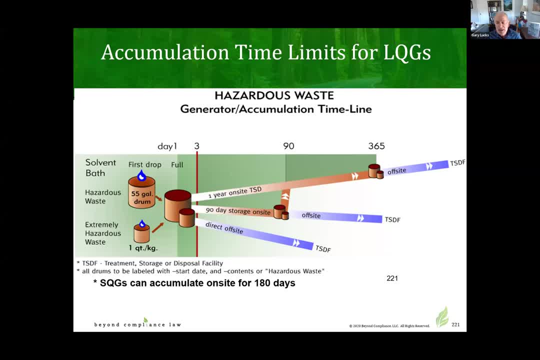 Michael Mann indefinitely. but once they hit 55 gallons- maybe it's it's three or four years from now- then they've got three days to move it to a long term accumulation area on site before which it goes off site. under California law it's more rigorous. under California law we say it's got to go off site within. 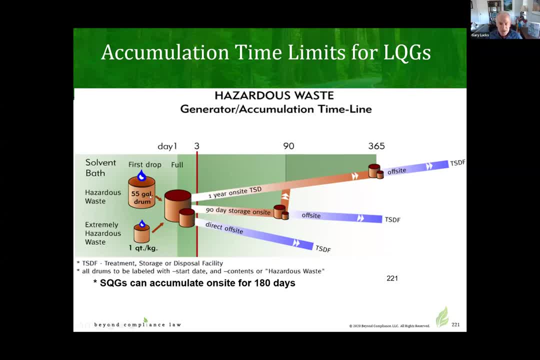 Michael Mann. 55 gallon volume, Michael Mann, Or one year, whichever comes first, Michael Mann. And that's a big deal, because Michael Mann The one for every day you accumulate waste more than the limit. it's under California law. it's $70,000 per day per violation, so it's a big deal. 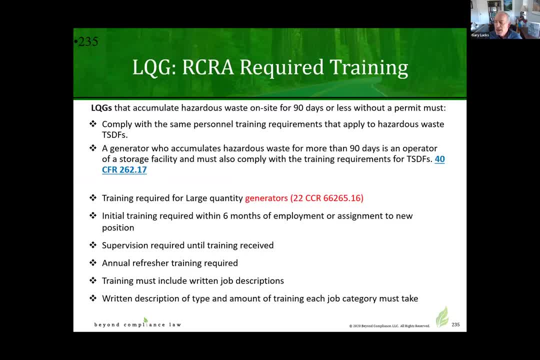 Michael Mann. More details here for later review. Michael Mann- The long term, the large quantity generator training, as I mentioned, is annual training. Michael Mann And a new employee must be working under the supervision of someone who's been trained until they get their training for at least six. 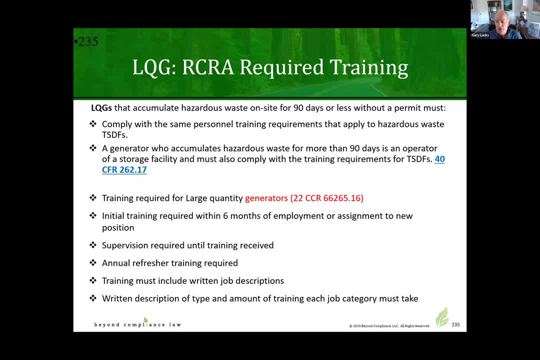 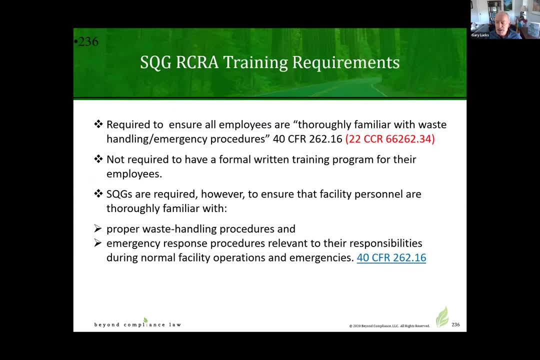 Michael Mann And then, but after six months they need to get their own training and then annual training after that. and then also there needs to be a written training plan. Michael Mann- Small quantity generators- don't need a written training plan. they just need to be thoroughly familiar with waste handling. 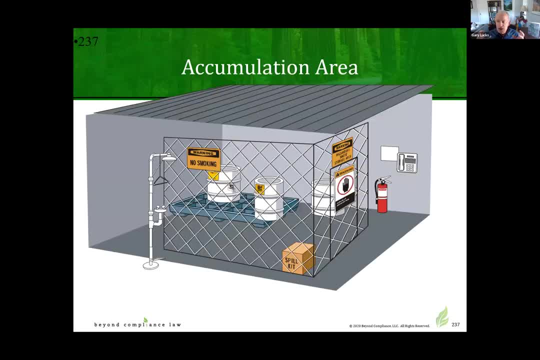 Michael Mann, So it's a lighter requirement for small Michael Mann Quantity generators. the long term accumulation area is a very rigorously managed Michael Mann Part of the facility because it's a Dane. it's dangerous to accumulate higher volumes of potentially incompatible chemicals that are generated from different activities at a site, so we need to be sure that we have appropriate equipment. 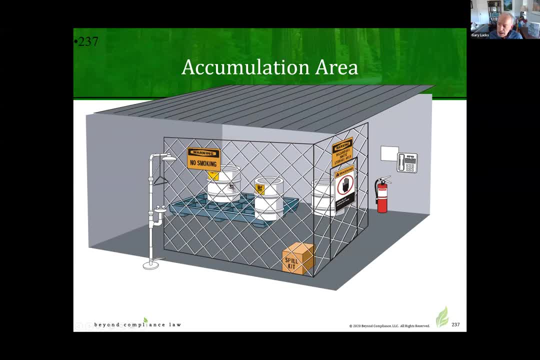 Michael Mann. Like fire suppression- a way to get some and help- a spill kit, a way to decontaminate yourself, Michael Mann, So we need to be sure that we have appropriate equipment that we're exposed to, let's say, an acid. 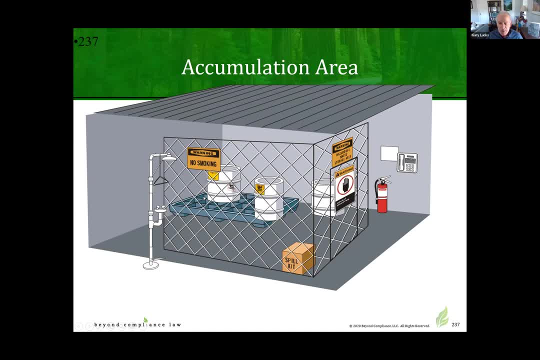 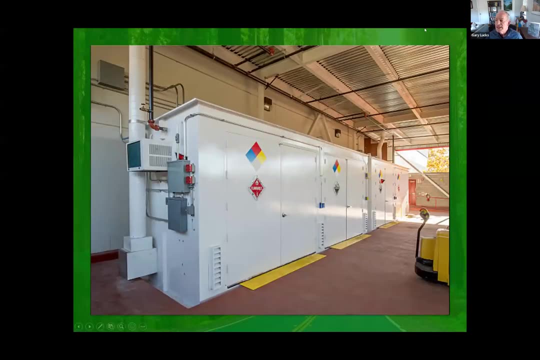 Michael Mann. And then secondary containment to keep chemicals from spilling and incompatible chemicals away from each other, among other things. so very easy to Michael Mann fall out of lines because these rules are just so prescriptive. here's an example of what a long term accumulation area might look like this. this left hand side might have the corrosives. 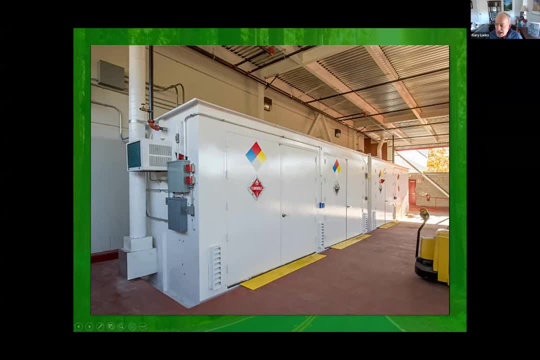 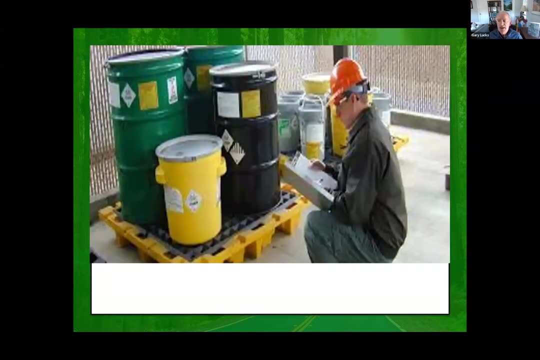 Michael Mann. We want to keep the crosses away from the ignitable and the reactive, so each Bay may have a different Michael Mann type of waste stream. need to inspect on a weekly basis to ensure that, Michael Mann, Everything we talked about: the equipment's working, the properly labeled, they're not being accumulated more than the accumulation timeframes, and so forth. 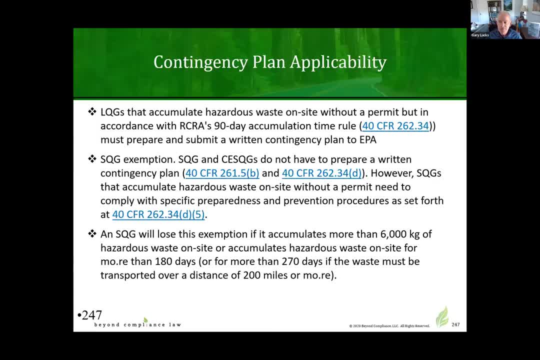 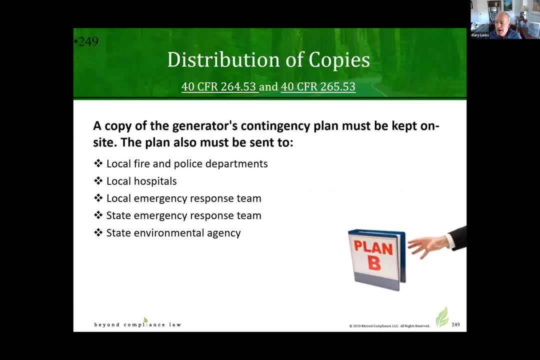 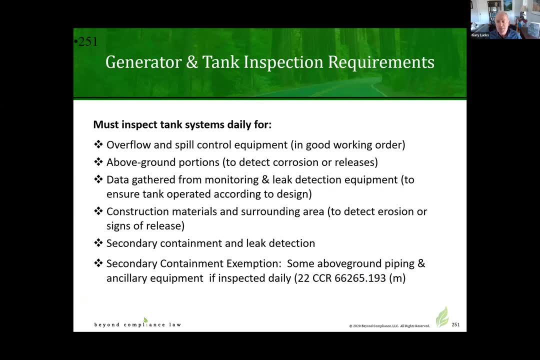 Michael Mann talked about the contingency plans that address earthquakes, fires and so on. they must be submitted to the fire department, police department, the local hospital. Michael Mann, um Michael Mann, hazardous waste tanks under subtitle see must be inspected not weekly but daily. daily inspections for hazardous waste tanks. 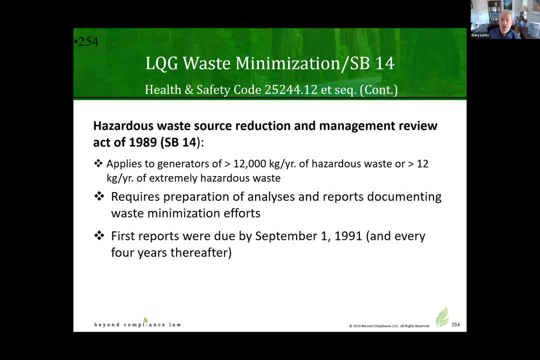 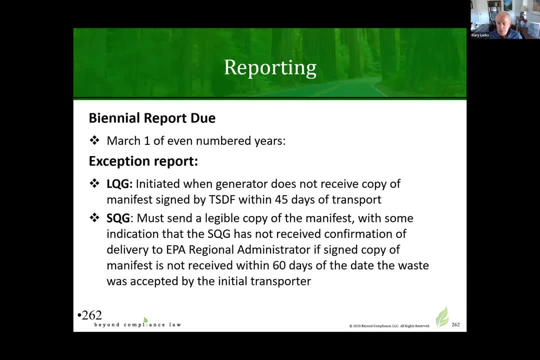 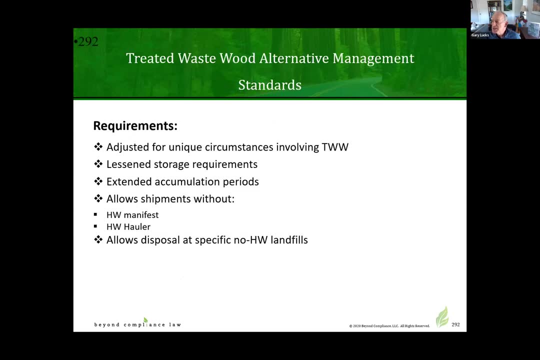 Michael Mann. SP 14 is the California unique law that requires large quantity generators to develop a pollution prevention plan. Michael Mann, We talked about the biennial reporting. Michael Mann- Oh, i'm sorry, reporting for Michael Mann Manifest. I already covered that talk about land disposal restrictions. treated waste would. 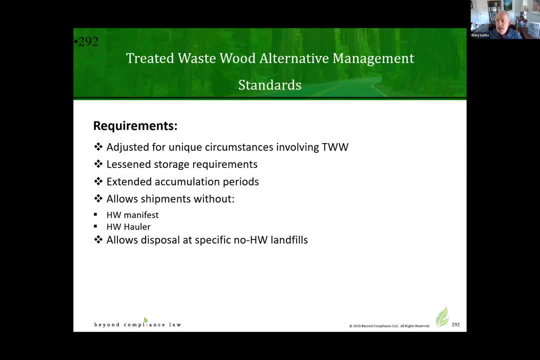 Michael Mann, what's treated waste would? treated waste word is basically your wood pallets in the warehouse, railroad ties and telephone poles. they're treated would so they don't preserve, but the treatment is toxic. it's got chromium, arsenic, Michael Mann, copper, and so any waste would that's treated cannot be managed as regular refuse because it's hazardous. 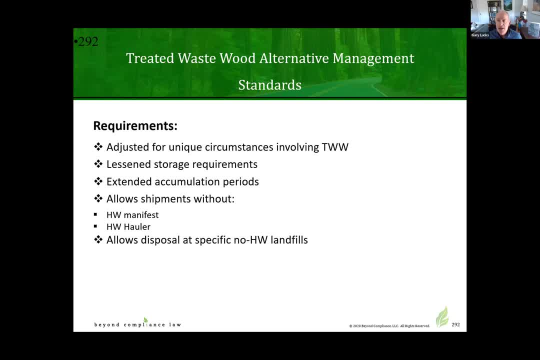 Michael Mann And under California, Michael Mann, California law, the legislature just passed a law that became effective January 1 that makes permanent more relaxed requirements for treatment treated waste with it as not as rigorous as if it was a hazardous waste but optionally can be managed in a lighter way. 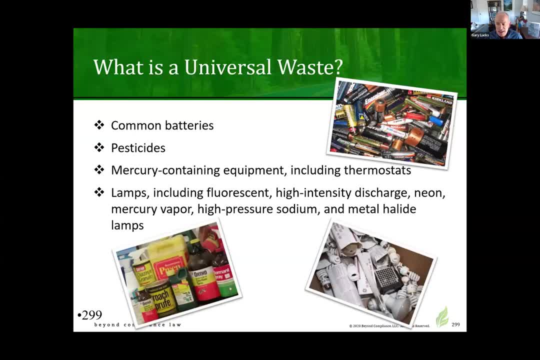 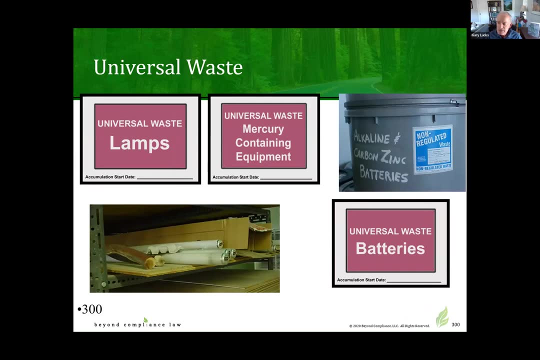 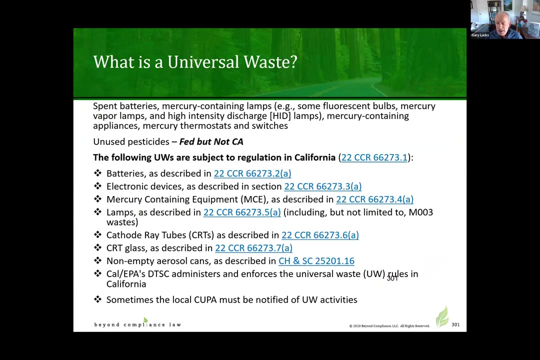 Michael Mann. same thing goes with universal waste, which are things like batteries, pesticides, fluorescent lamps. they can route more lightly and don't have to comply with as rigorous labeling, Michael Mann, And accumulation hold times. they need to have certain labeling, as you see here, and it also includes not just batteries but cathode Ray tubes in in TV sets, CRT, in computer monitors, among other requirements. 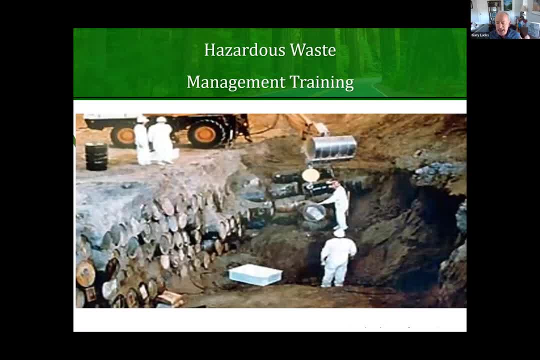 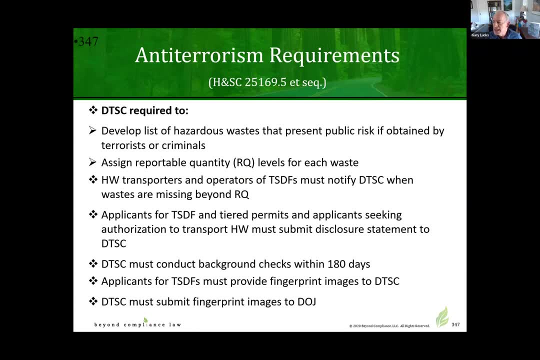 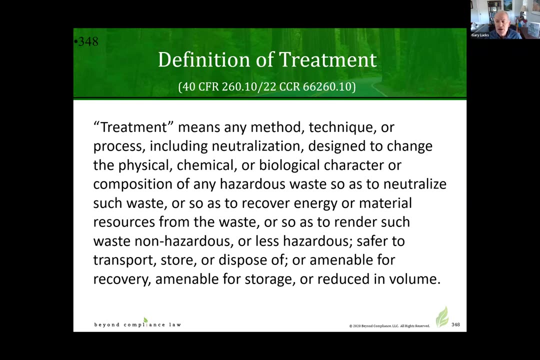 Michael Mann, The long term or the off site facility that takes all these ways has to be very heavily managed. we're not going to go into those details at all, other than Michael Mann. we believe, and have gone over them in a multiple times in podem convo, of those laws and Hari. 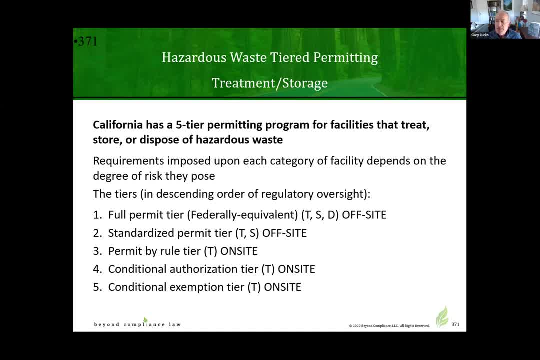 Michael Mann. The second piece of information I have for you is the Michael Mann Partly. I think this is a great topic, Michael Mann. A lot, Michael Mann, To share with you. that Michael Mann, First of all, I do want to point out 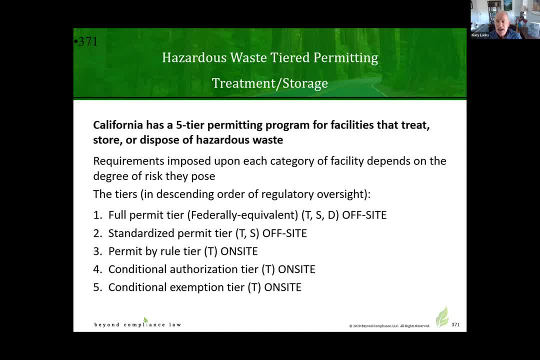 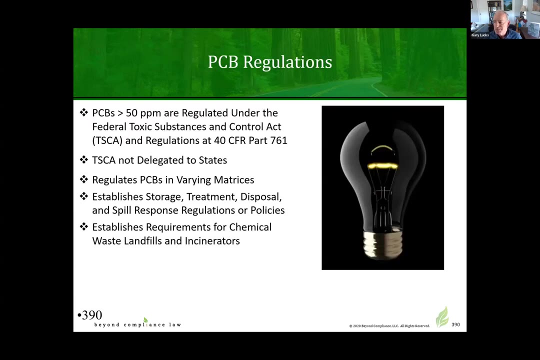 permits that govern the commercial facilities that will take the hazardous waste that arrive at their facility. And in some cases facilities can actually do their own on-site treatment and long-term storage under what's called different tiers of activity, under what's called the hazardous waste tiered permitting program that's managed by the CUBAs. PCBs- polychlorinated. 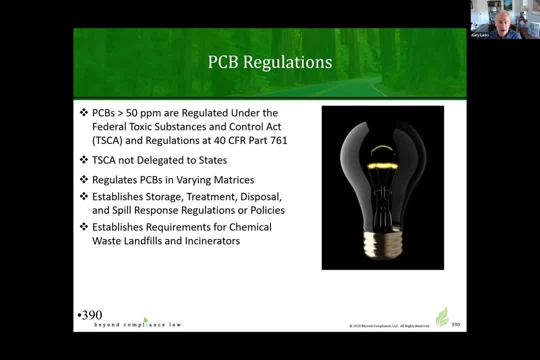 biphenyls. you'd think they'd be regulated under the hazardous waste rules but, due to a quirk of history, are regulated under the Toxic Substances Control Act And the federal law only regulates polychlorinated biphenyl- PCB wastes of 50 parts per million or more. Anything less is not regulated. 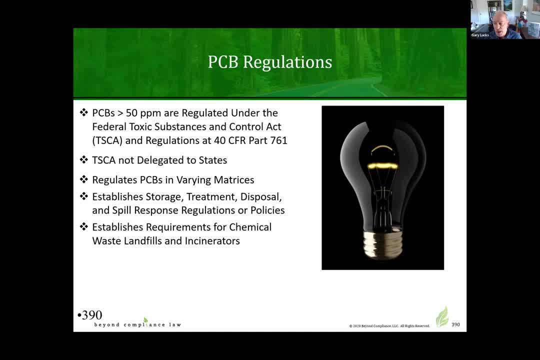 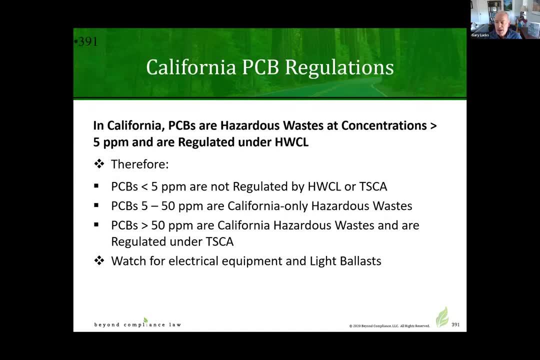 under TSCA, but it is its own cradle-to-grave program that in many ways, but not always, is similar to the regulation RICRA, subtitle C: cradle-to-grave program. California regulates PCBs less than 50 parts. 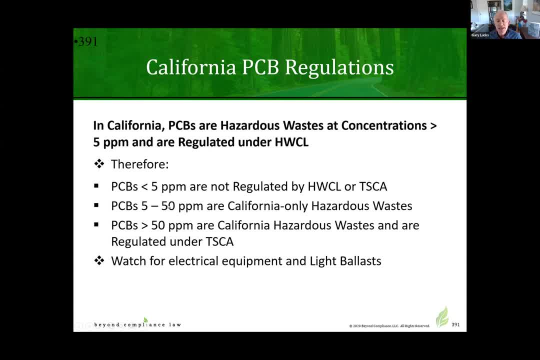 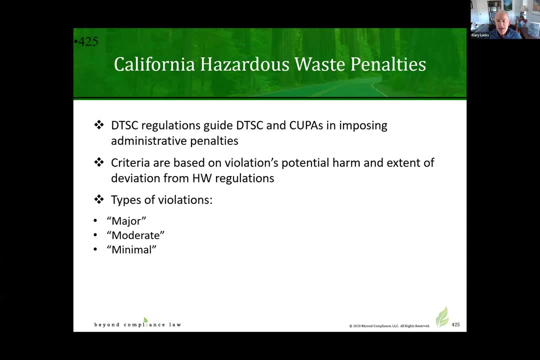 per million. A PCB less than 50 parts per million is a California-only non-RICRA hazardous waste. So another example where something that passes the federal would fail the state and must be managed accordingly and labeled it as such: Penalties extremely expensive to violate. 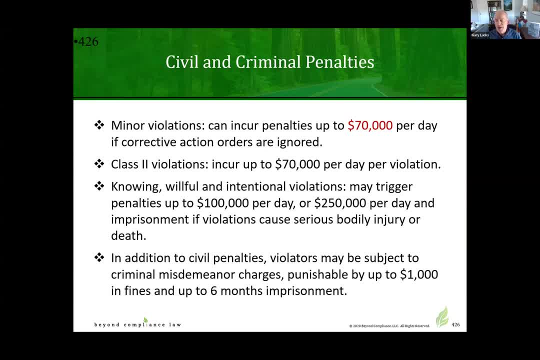 hazardous waste laws. The state legislature three or four years ago raised the penalty per day per violation to $70,000 for a civil or administrative penalty and more for criminal willful. The federal government under the Obama administration raised it to over $100,000. And so many people do not know that. 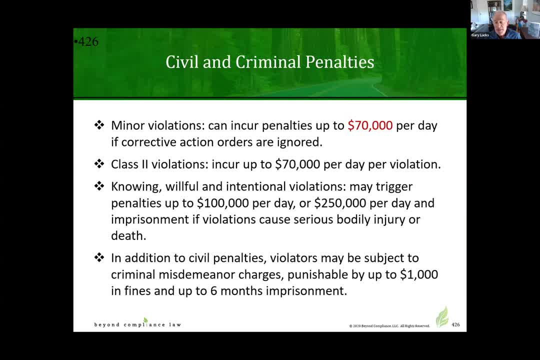 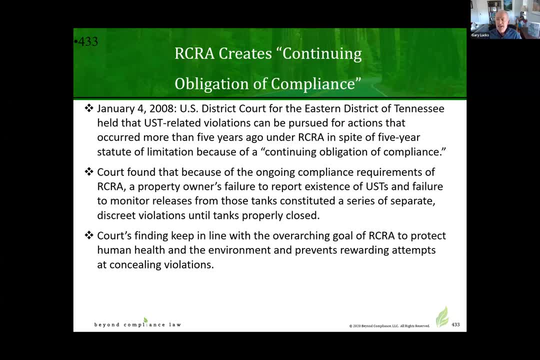 the federal law's penalty structures have been dramatically increased, including hazardous waste, in the last couple of years, And so the federal law has been dramatically increased in the last couple of years years. The last thing I want to share with you is remember RCRA covers more than RCRA. 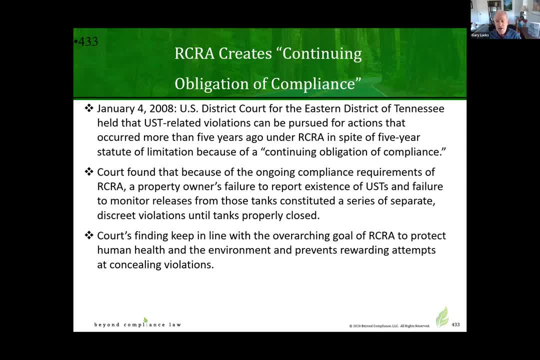 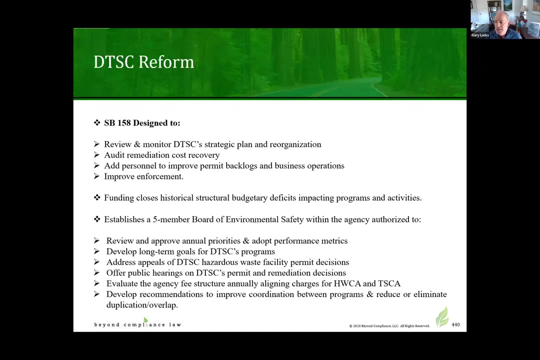 subtitle C for hazardous waste also covers underground tanks and municipal waste. There was a district court case in Tennessee that basically blew past the idea of a statute of limitations And because in the statute RCRA creates a continuing obligation to comply notwithstanding the statute of limitations. I promised the last thing, but I was wrong. 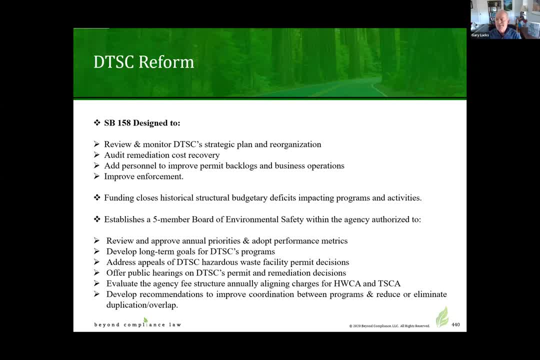 There's one more slide And the legislature just approved a long-awaited law that became effective this year: Senate Bill 158.. When I wrote briefing papers for Governor Newsom about a few years ago, a big issue at the time was reforming the Department of Toxics, which was 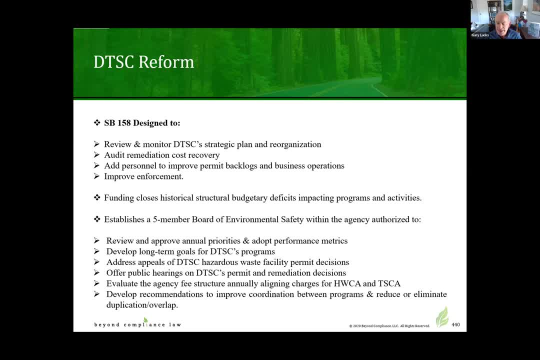 an agency that was found to be not as effective as other agencies, And so the legislature just reformed the Department of Toxics, which was an agency that was found to be not as effective as other agencies, for a variety of reasons, And in my briefing paper I shared some of the root causes. 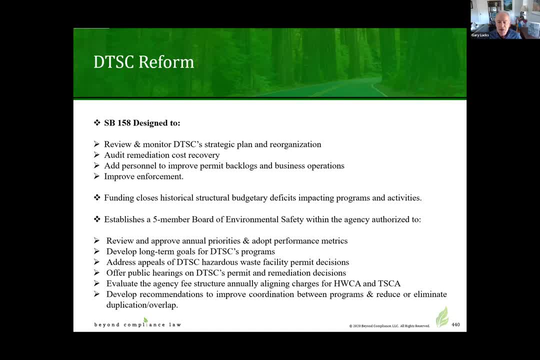 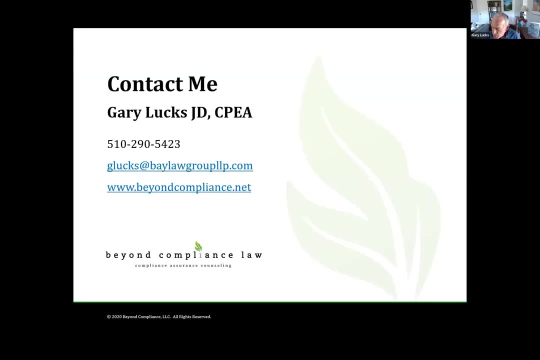 that other people had studied. SB 158 addresses all these issues. that, among other things, calls for increased funding and a five-member board of safety that is like a board of directors that oversees the agency. So we sprinted through what is probably a six to eight-hour class. 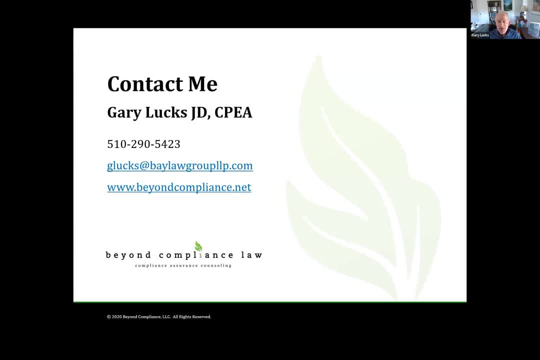 and still have time for questions. So apologies for going so quickly, but I hope you have an opportunity to ask some questions now. Thank you so much, Gary. Yes, And I was actually going to ask you, but you squeezed it in. I. 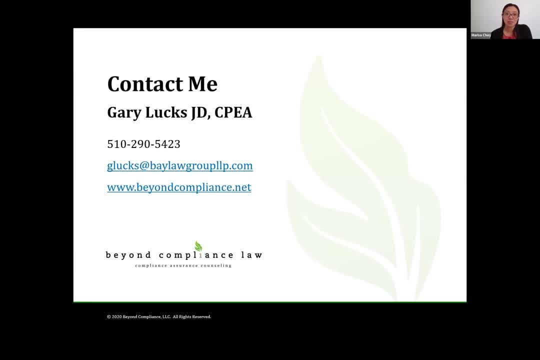 wanted you to just touch on what are kind of the stakes right in terms of enforcement and penalties, because I think that's often for listeners where it comes out, As you've heard, there's lots of landmines and traps for the unwary, because it's very prescriptive and there's all 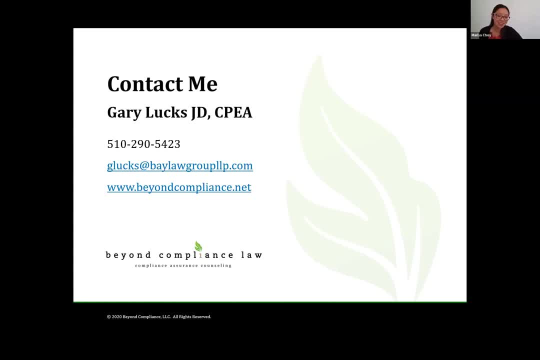 these code sections And who knew that you had to label things certain ways and store them in a certain way and train all the people. So there are lots of ways to trip up And that's why you have to either find auditors or consultants or hire lawyers to help make sure things are in. 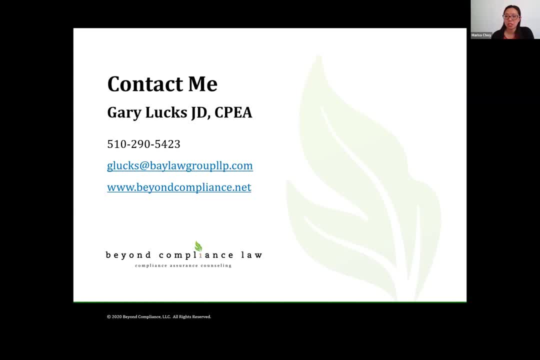 compliance. We did get a couple questions and the person may have figured it out, but she just wanted to clarify the toxicity test for the mixture rule. You mentioned that for the other properties, like ignitability, corrosivity, if a single drop goes in, if it's mixed in, it's just a matter of whether the mixture passes or 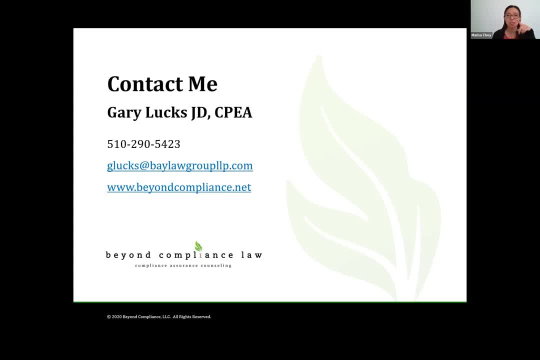 fails the test. But it sounded like toxicity. just a single drop contaminates and the mixture becomes a hazardous waste. So she wanted to know, curious, how the toxicity test applies to the empty container If only one drop means it could still be a hazardous waste. So, Gary, is it correct that? 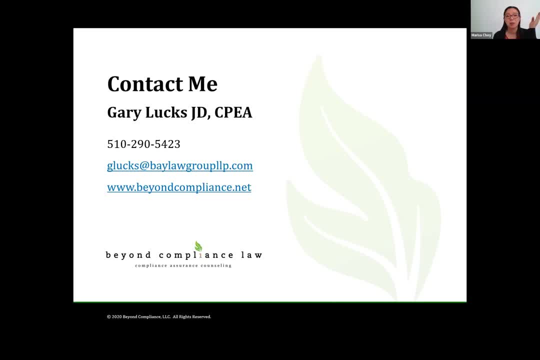 an empty container, if it had a single drop left residual of toxic material, even though it's- quote- empty, would it still be a hazardous waste? Good question, The answer is no. It's so many gray areas here, but I think the definition of the empty container. so there's the mixture rule which we 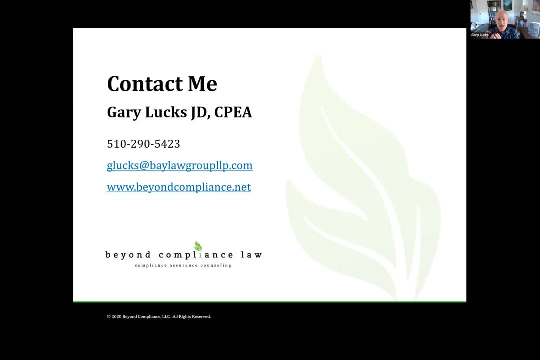 talked about dilution and the pool Right. And then there's the empty container rule, which is just for containers. So the fact that it's a container, then the empty container rule would override the mixture rule. So it's the empty container rule And therefore, if it's less than 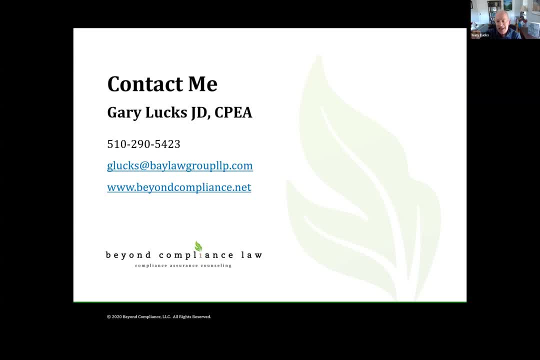 one inch of a toxic material, then it does not have to be managed as a hazardous waste. Yeah, These rules are just. it's, oh my God, there's a lot to them. Yeah, Yeah, Great question. Yeah, Exactly, Very good question. Now we know. Okay, I guess let's see if anything else comes in. 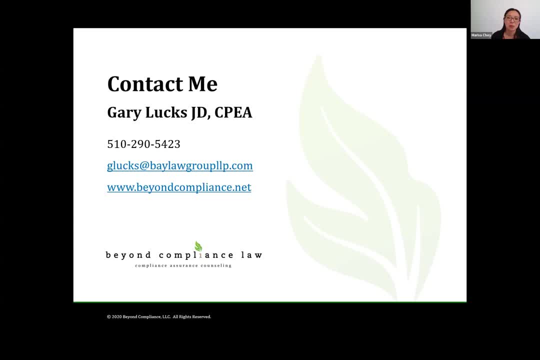 I just thought you know, in your long experience and history with helping companies run audits and respond to enforcement or compliance issues, what are some of the most common- maybe mistakes or unintended slip-ups that you see just for people to keep on their radar, And maybe you can talk about the types of companies and industries that these 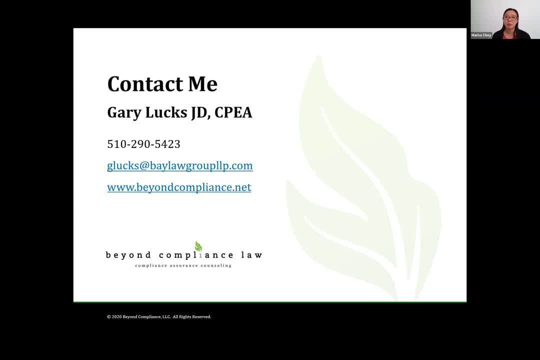 regulations apply to, because I think there may be people on the phone or on the call who are not environmental lawyers and they're wondering: gee, does this apply to me? But I think it's pretty wide ranging, Like you said: construction, a lot of industry, metals, oil and gas. 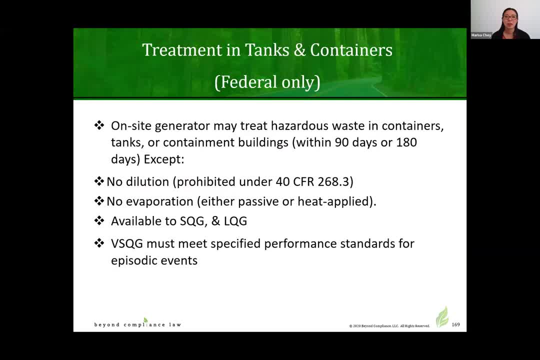 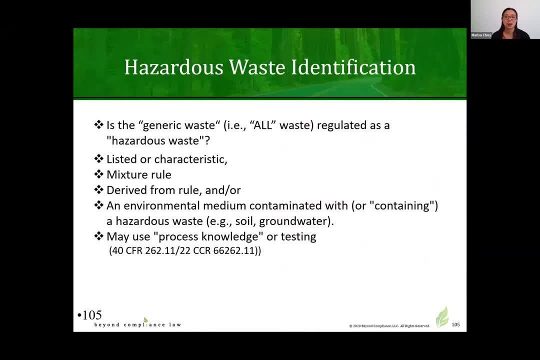 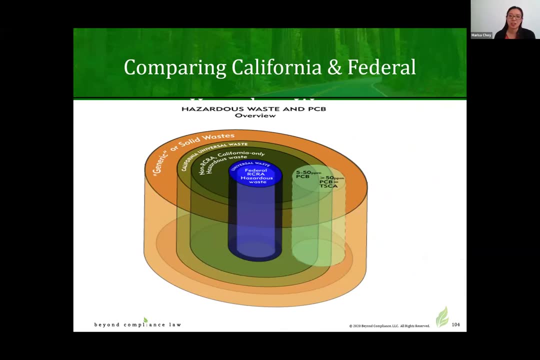 you know and even probably folks have seen. you know, bring in your batteries or your old computer equipment, because there are all these rules about how waste is managed And, like Gary said, the waste is supposed to go. the different streams have to go to certain categories. They have to travel with licensed 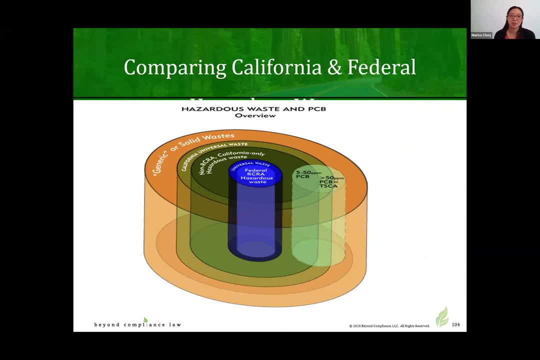 transporters and they have to end up with the right kind of landfill or ultimate disposal facility. Yeah, Great, Great question. So the two parts, I'd say the area where people often get tripped up is here. They test, they're in California and they don't run all the tests and they assume 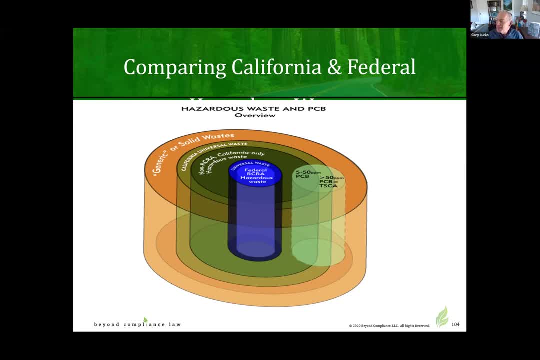 oh well, I passed this test, but they're sticking their head in the sand, or just not knowing that there are other tests You have to. if you fail one test for toxicity, you do the less rigorous federal test, think you're home free, but you've not run the California tests, or? 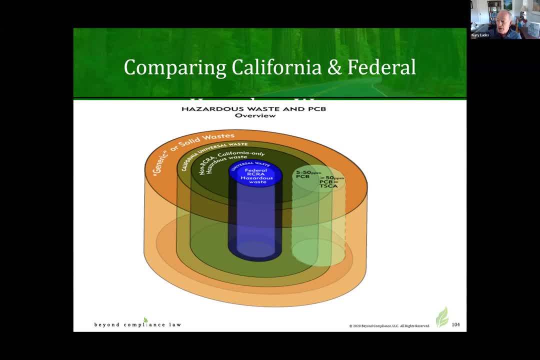 tests, You have to run everything. If a regulator says, well, we're going to run the total threshold, limit concentration and it failed that, then it's a hazardous waste. And if you manage a hazardous waste in regular refutes, that's a per day per violation. you're talking hundreds of thousands. 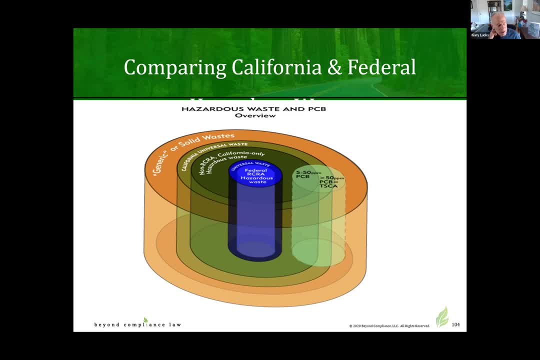 of dollars in theory. So that's one area where I think people get tripped up. They often get tripped Well. to your other question, these rules were designed for industry that they've been applied. Even I'm working with some retail companies that, and some of you may- 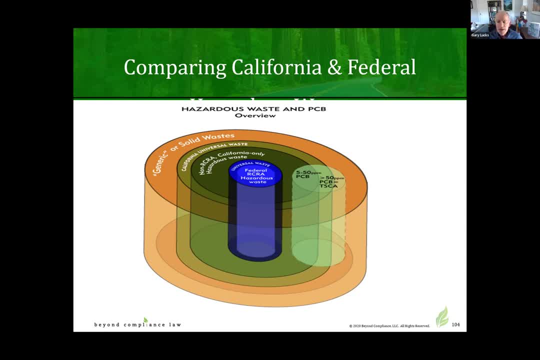 know that several district attorneys have been dumpster diving in supermarkets and retail operations And they're finding, you know, bleach in the dumpster, which you know the. the bleach is a non-empty corrosive, for example, And so they're not. so these are broad based. 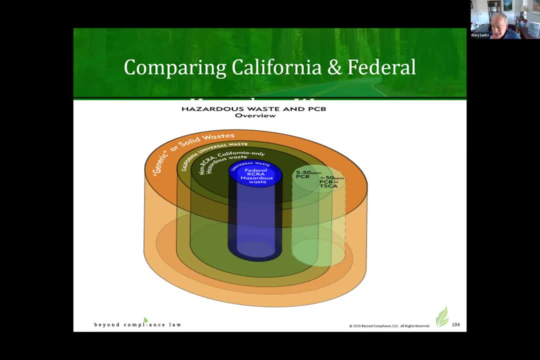 rules And the bottom line to me is: I think organizations- well-meaning organizations- fail these rules all the time. I've done over 500 audits my career and I always find problems, especially at the long-term accumulation areas. So my advice to people is: you got to train the heck out of your employees and make it a user. 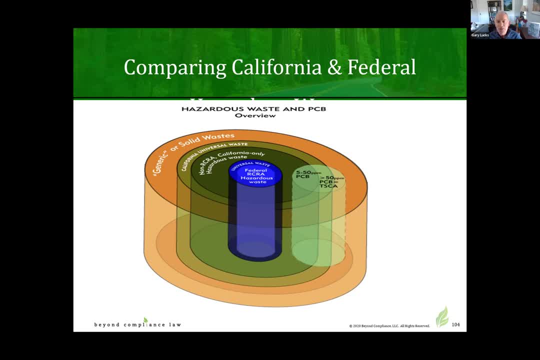 friendly training, So they'll get it, and refresh them, So they'll get it, because there's no excuse for not getting it right. And then I think people should deputize people to do self-inspections, and you should do regular audits, or at least regular audits of the activities at a facility that they 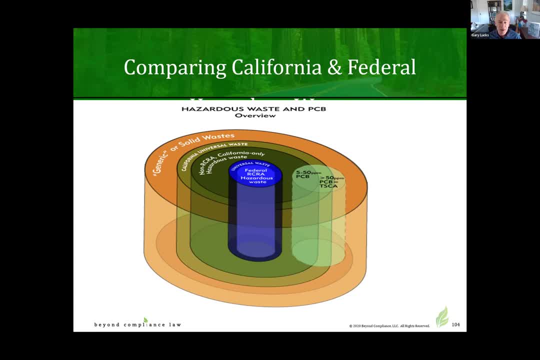 think are the biggest risk. hazardous waste is definitely a big area, Air quality is a big area, but whatever target on your back is most likely Speaker 2- put those resources into auditing or training, Great, Yeah. Well, hopefully in our- if we can manage to- to wrangle a second section. 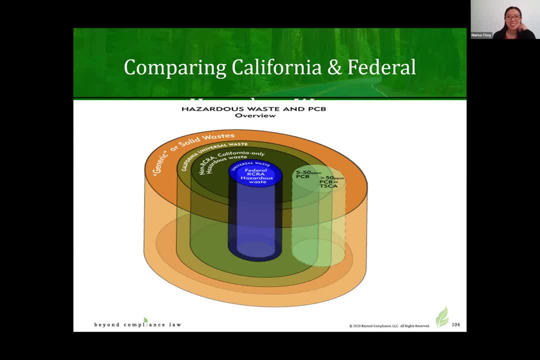 we'll hear a little bit more of of a real world examples and some of our clients who who have had those dumpster diving audits and and you know, get in trouble. but I know we're at time, So if people need to drop off, understood. there's just one last question, And so I'll let 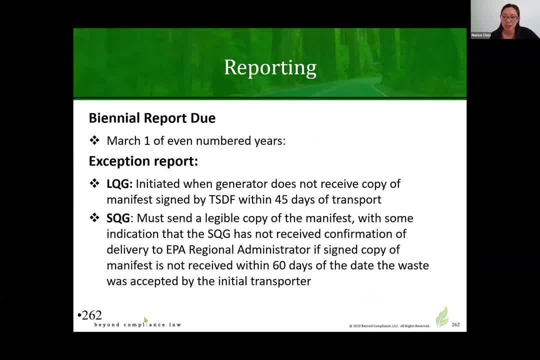 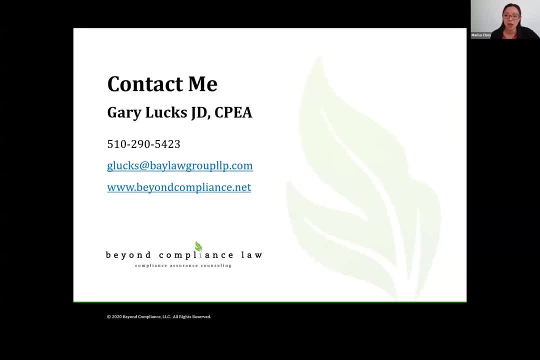 you answer it, Gary to. to wrap up, Kevin Woldhagen wrote. thank you for the great presentation. Have these regulations have the effect of inspiring businesses to develop better products that aren't as harmful to the environment, or do companies just try to comply with the regulations as best they can? 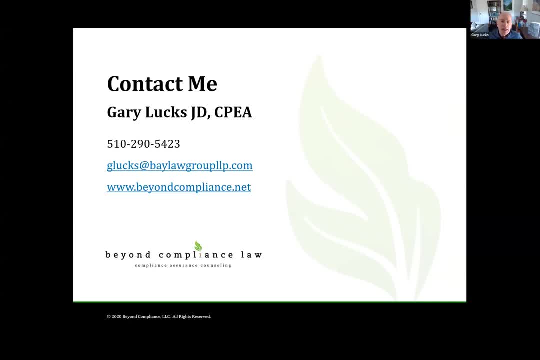 That's a great question. I think it's. this law does not, in my view, drive product formulation. What drives product formulation is prop 65- sustainability drivers, where the supply chain or stakeholders are wanting to, that motivate the company to set themselves apart through greener products, And of course that's always a risk of greenwashing in. 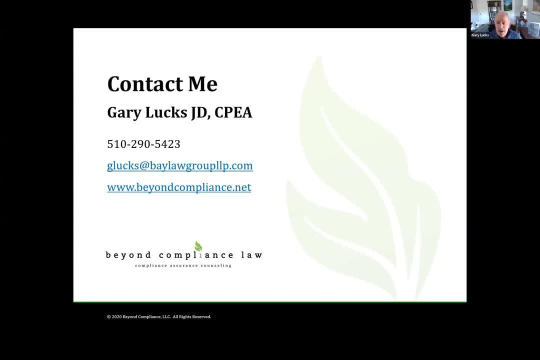 the law which I'm writing a chapter in the treatise on, on that very thing. right now There's a lot, that's a big deal, Like a lot of companies are focused on sustainability and they're- they're all ready to promote their success stories and sustainability And they unwittingly 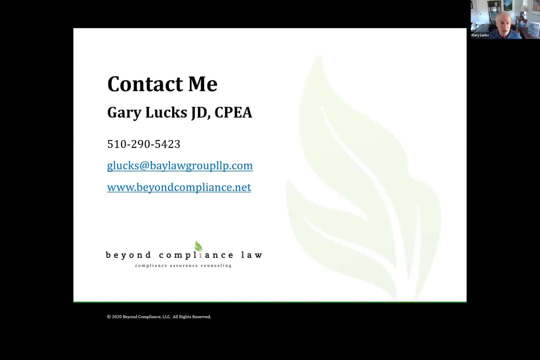 they run afoul of the Federal Trade Commission's rules governing greenwashing and the state business of professions- code 7800.. But nonetheless, prop 65, overreach on sustainability or, excuse me, prop 65, sustainability drivers are the ones that result in product formulation. And then 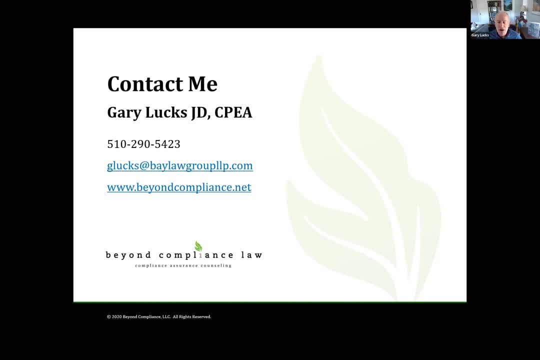 there's also the AB 1879 law, which calls for product stewardship and that's slowly advancing in the Department of Toxics, to deter the more dangerous products from being introduced in the commerce, And lastly, TSCA, the Toxic Substances Control Act. 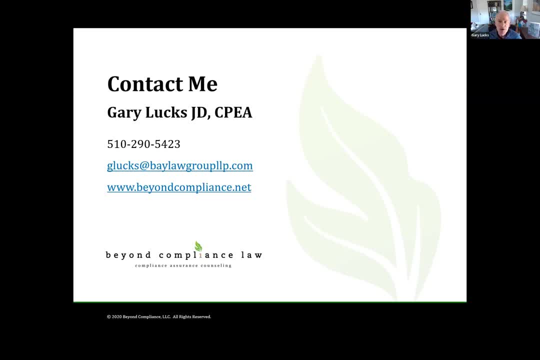 is also, especially with the new Obama regulations. it's more of a driver to encourage more benign alternatives. But hazardous waste rules, I think, are not the driver. Yeah, good to know that. that comports with some of the things that I've seen as well. 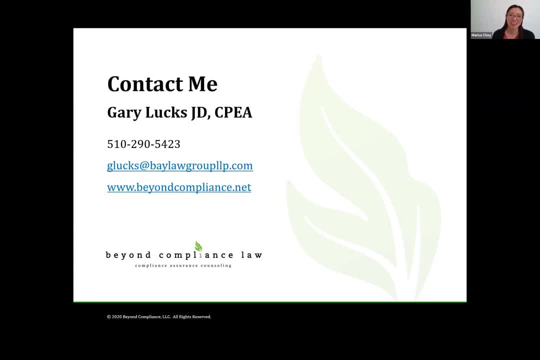 And, like you said, if you have someone out there, you can probably find something wrong. So it's a little bit of doing the best that you can. Well, I see that Larry has put his info on the screen And again, I encourage everyone to check out the website. 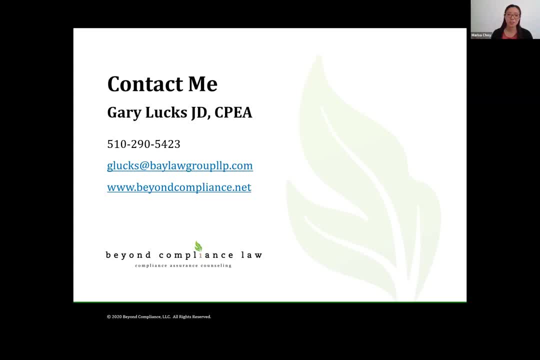 and tune in for later sessions of the completely free 101 sessions, and they will be recorded and available online. Well, we're a pleasure. If you have any questions, email me, I'm happy to respond, And thanks for the opportunity, Marissa. 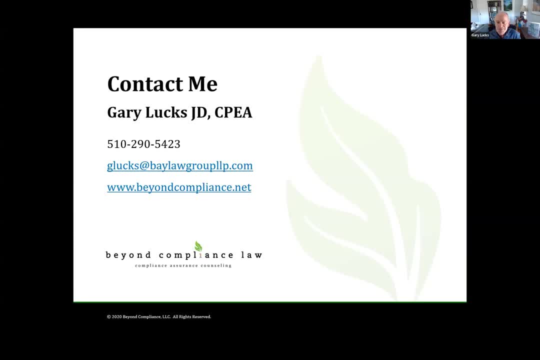 and have a great rest of the day, everyone. Thanks, Thank you all. Take care.